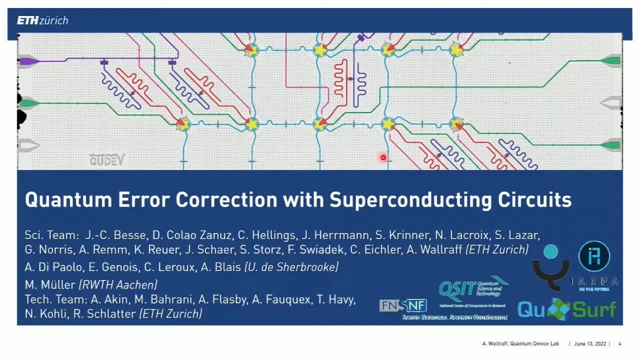 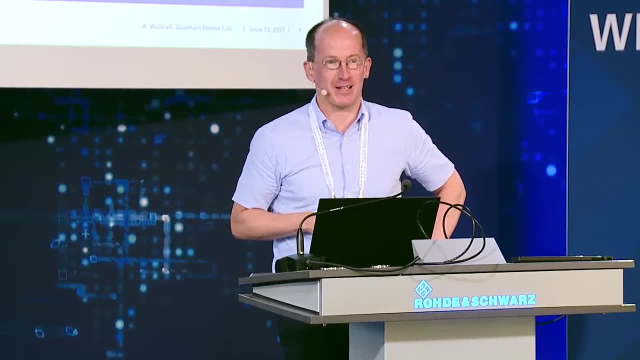 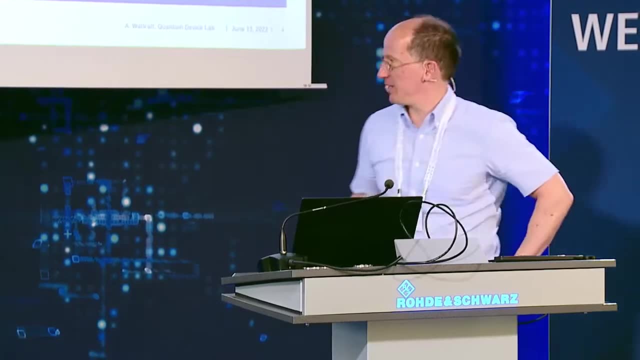 There was lots of competition. Essentially, everybody wants to implement error correction on larger scale superconducting circuits, Like, obviously, all the academic labs and also all the big IT companies like Google and IBM. So let me see how I position myself and whether my pointing works. 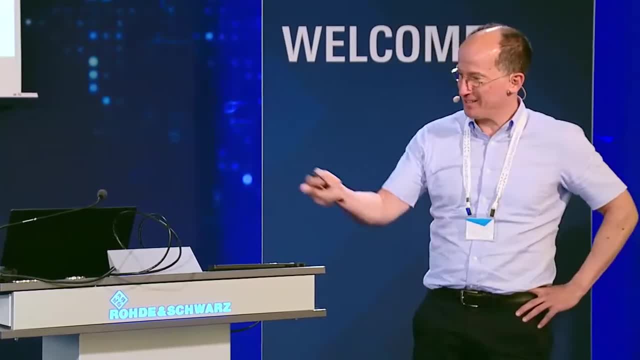 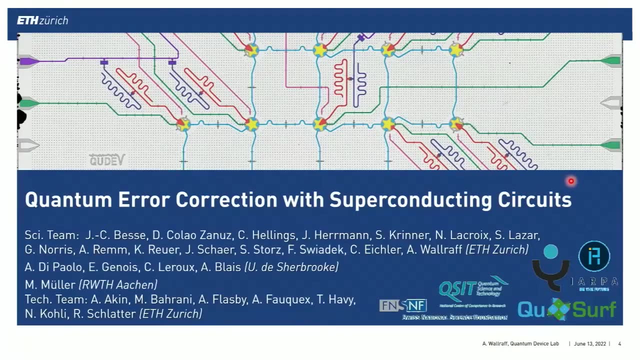 Yeah, here we go. Maybe this looks more familiar to me than just looking directly at my screen. All right, So the title of my talk is Quantum Error Correction with Superconducting Circuits. It has been done with a team of experimentalists at ETH. 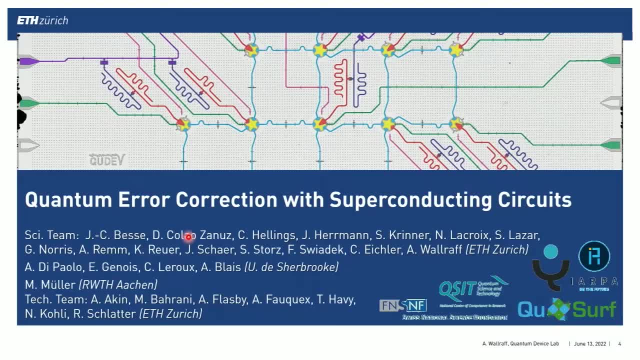 So they are listed here. It is really a team effort, So lots of people have contributed. As I said, we have worked six years on it. There are then two who were really in the lead for pushing the experiment across the finish line. 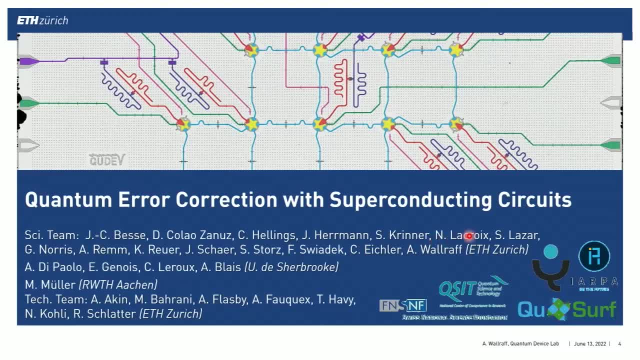 And that is Sebastian Krinner, a postdoc, and Nathan Lacroix, a young graduate student. But we have also collaborated, in addition, very successfully with a group of Alexandre Blais, who is at the University of Sherbrooke, who is really a long-time collaborator with our lab. 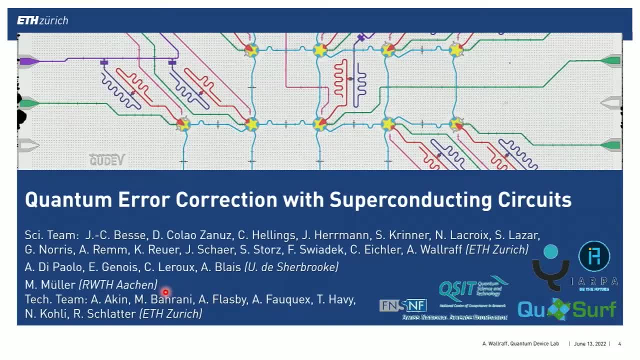 and also with Markus Müller at RWTH Aachen, And since it is also quite technical, I would like to thank our technical team as well. And then also: yeah, good things take time. So this experiment took six years, but we are also at ETH since now more than 15 years. 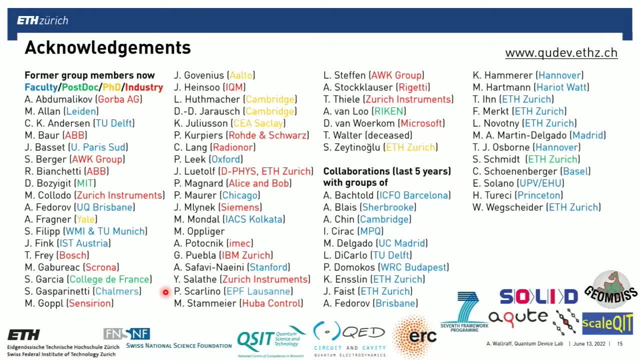 And so quite a few people have contributed to our lab During those, and maybe some in the audience recognize their names somewhere on the list. So there is Anna Stockklauser, who will be on the discussion session tomorrow, I guess. 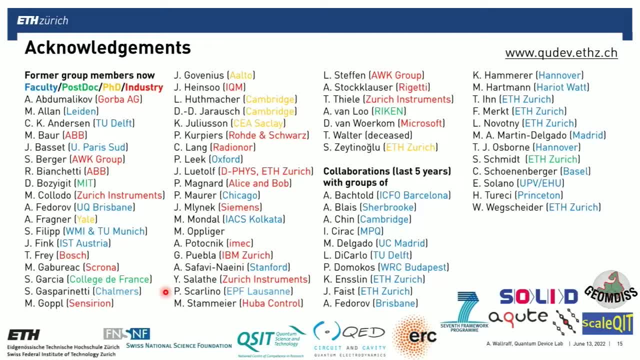 who is at Rigetti now, was a grad student in our lab. Who else So? there is Stefan Philipp, who is a speaker tomorrow- was a postdoc in our lab. There is Philipp Korpiers, maybe somewhere in the back, who was a grad student in our lab. 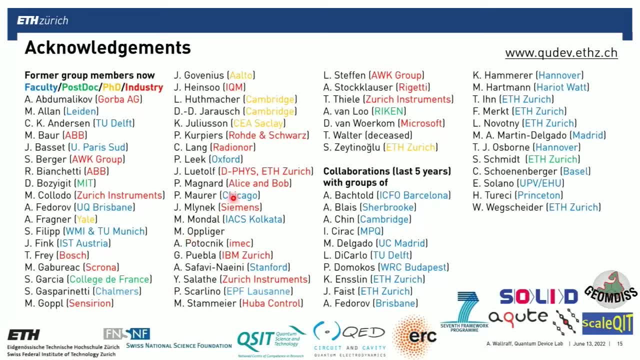 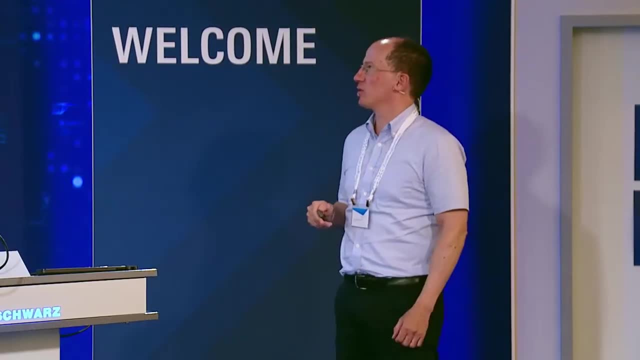 And if you now look at it, there is quite a few faculty members all over the world who did some work in our lab And the rest is sort of distributed equally among kind of technology companies in the quantum realm and also sort of small and big startups. 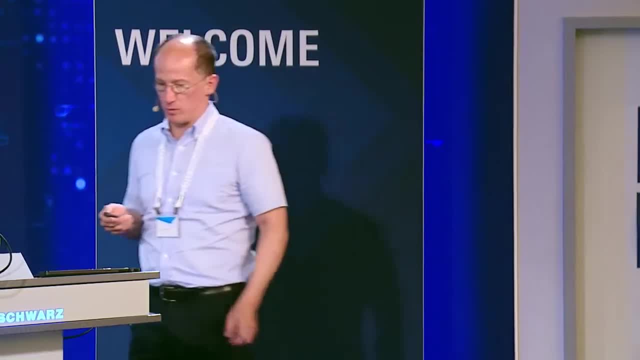 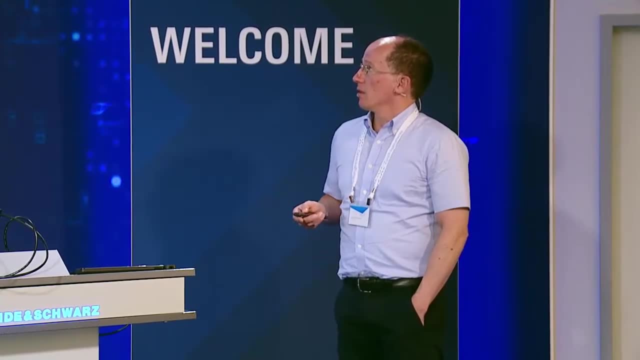 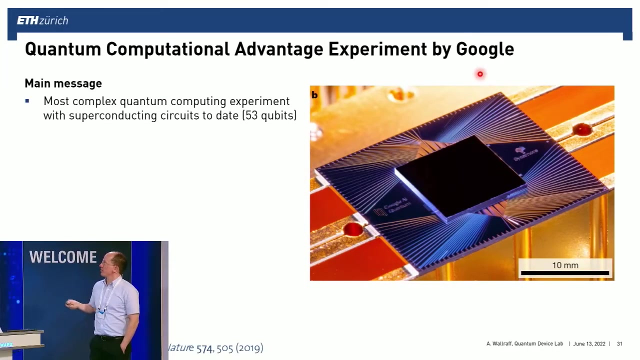 So that is nice to see, and we are very thankful for everyone who has contributed to our lab throughout the last 15 years or so. Good, So why quantum error correction? So maybe I guess all of you remember this breakthrough result from Google. 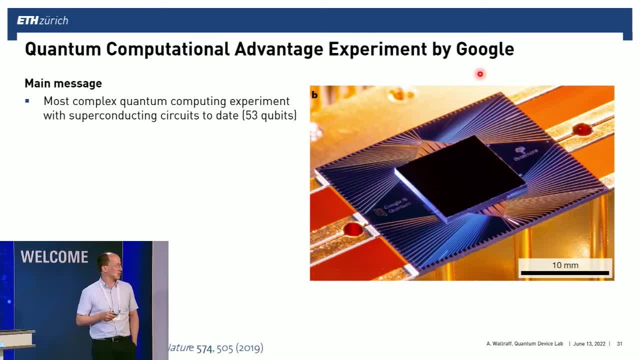 now, maybe three years back, It is this quantum advantage, quantum computational advantage experiment That was really impressive and it still is really impressive. I would say They had 53 qubits on their device, which is shown here on the right hand side. 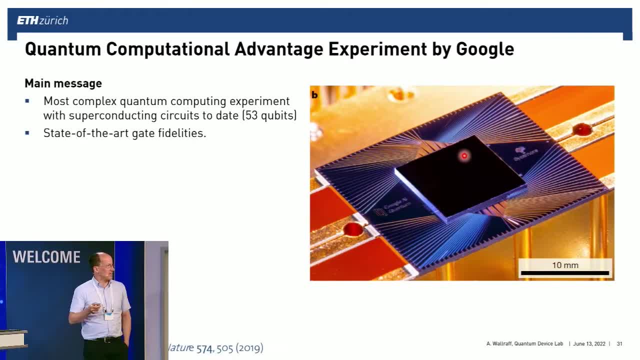 I think they had sort of state of the earth, State of the art, gate fidelities for single qubit and two qubit operations And even though it is now three years ago I think things improved somewhat. but I think this really represents the state of the art still quite well. So what did they do at the time? They demonstrated an advantage in their little 53 qubit quantum computer over a conventional computer. Essentially, they picked a problem where the difference between how a quantum computer would perform and how a classical computer would perform is maximized to some degree. 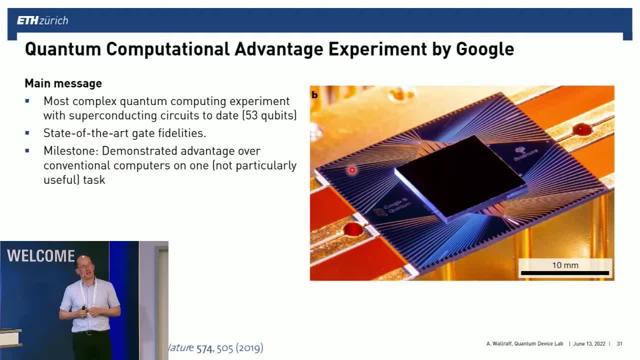 And this is very impressive- So they could run head-to-head the quantum computer against the classical computer. The challenge with it is, though, that the task that was looked at wasn't particularly useful, So they essentially ran a random gate set on their 53 qubits. 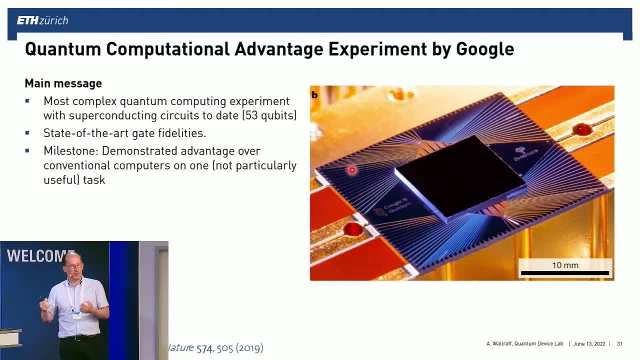 and this creates a very different, very difficult to predict and calculate, but random entangled state of all these 53 qubits, which is very hard to simulate on a conventional computer. So maybe one word about why is it that this is then hard? 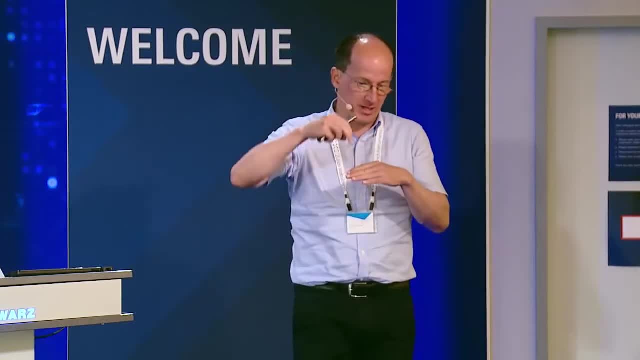 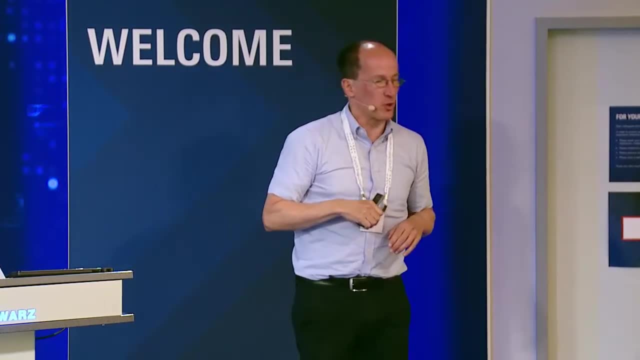 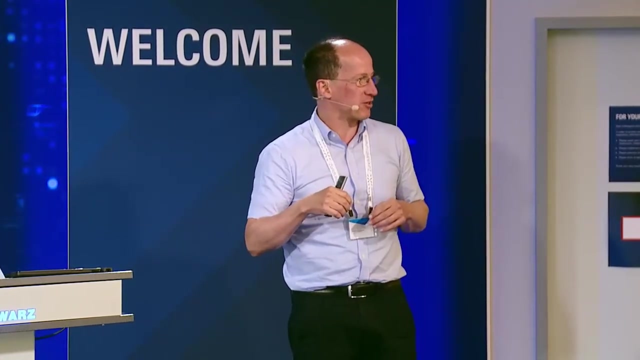 or why are more interesting questions? why does the gap between how the quantum computer does and the classical computer shrink for more interesting questions? That is mostly because more interesting questions basically have some logical structure to them And the fact that there is some logical structure to the problem. 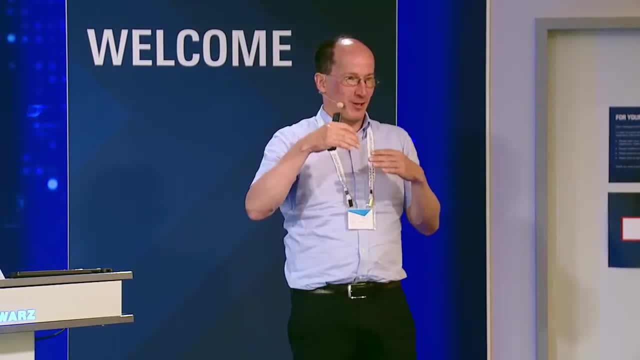 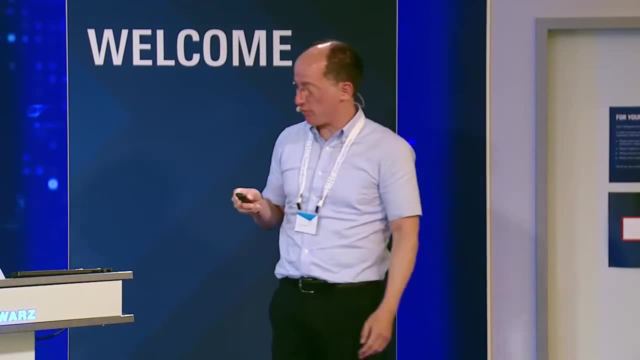 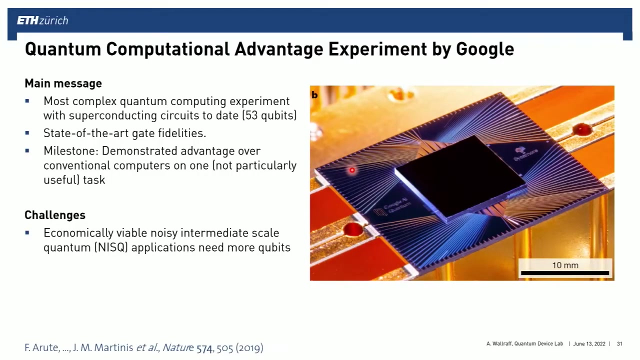 and how you would solve it algorithmically gives the classical computer a better standing against the quantum computer. Essentially, this gap shrinks in between the performance of the two systems. So therefore, this may be not a particularly interesting task, It still constituted a milestone. 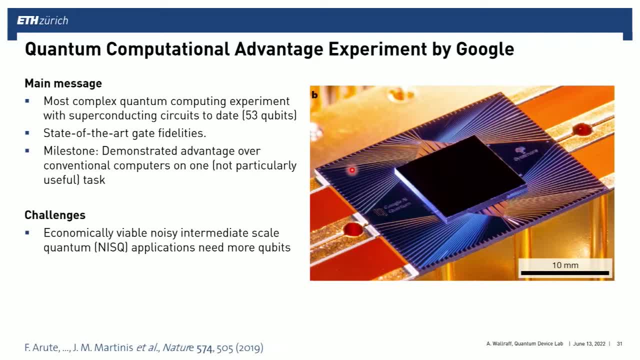 because it was the first time when a quantum computer was doing something that was hard and maybe impossible to simulate on a classical computer. So clearly 53 qubits is not enough for doing kind of non-error corrected quantum algorithms in the future that are interesting and not simulable. 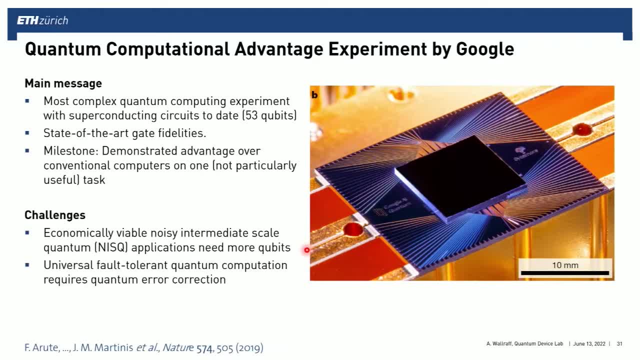 because of this sort of shrinking gap when the problem is interesting, And also, in the end, you probably want a fault-tolerant universal quantum computer, one that does not suffer from the errors that your qubits suffer from. And what these errors are I will explain in a bit. 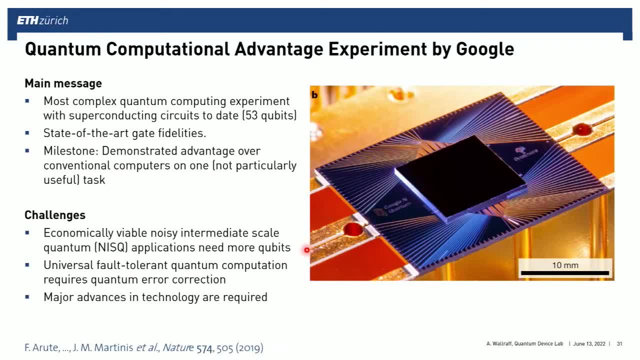 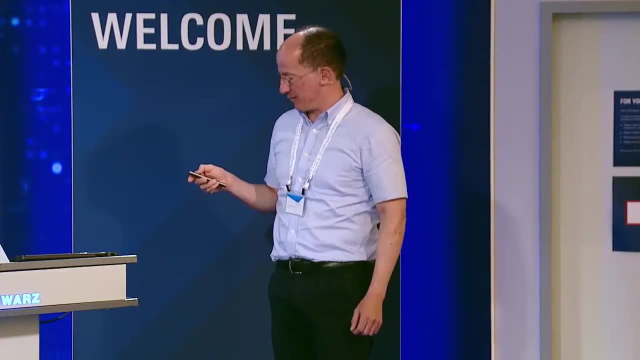 So maybe let us talk a little bit more about- And this requires still quite a bit of advance in technology at all ends, So I think, for scientists and students and research labs at large industries. so this means that there is probably lots of work ahead. 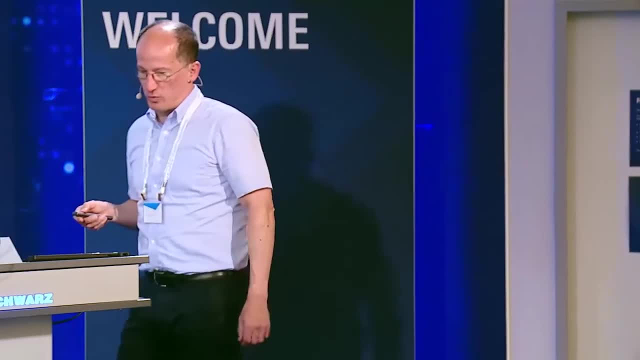 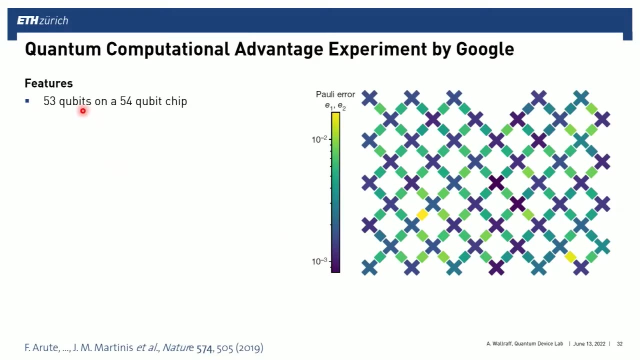 still at the current stage, So maybe to see a bit more what error correction might be needed, let us take another look at this Google experiment. So on the device, 53 out of 54 qubits worked, which was quite nice. 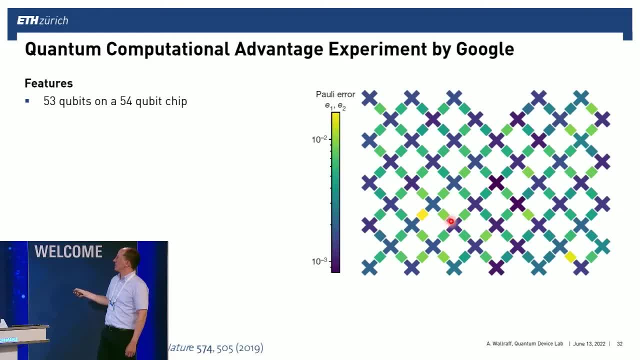 Here on the right-hand side you see a picture of what the device schematically looked like And that is sort of the level of detail that you get to look at the chip from Google these days. So if you want to look at what the qubits look like, 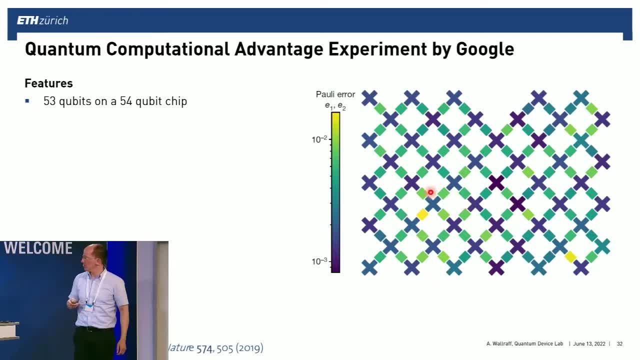 you have to kind of live with seeing a little cross that tells you the fidelity of the single qubit gate operations and the fidelities of the couplers between the two. So there were 53 out of 54 qubits were working. 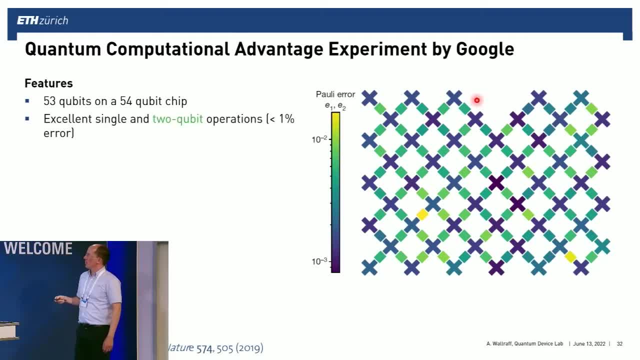 There was probably a qubit up here which did not do its job, So the two qubit operations were all really quite good at a 1% fidelity level. The single-shot qubit readout, the ability to read out the state of these qubits. 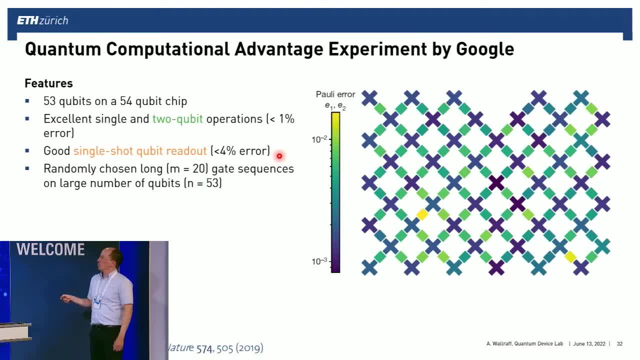 was a bit worse, maybe around 4%. And then what was implemented on this? a set of 53 qubits. essentially they executed pairwise two qubit gates, so between every one of these crosses as much in parallel as possible. So essentially they paired up all the qubits. 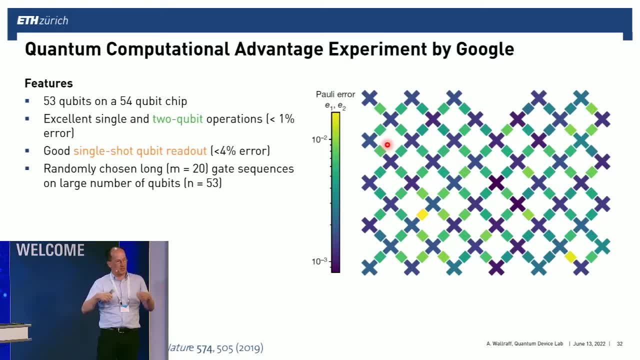 ran a two-qubit gate between it in one time step and then in the next time step they ran the next two-qubit gate And they did that for roughly 22 qubit gates in sequence. So you end up doing about 1,000 two-qubit gates. 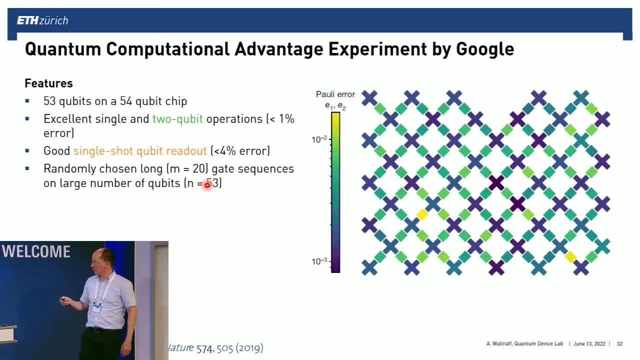 on this device in sequence And you add a few single-qubit gates to it and you create an outcome and you do measure all your 53 qubits and you ask yourself: okay, how well can you reconstruct that state or compare it to the target state? 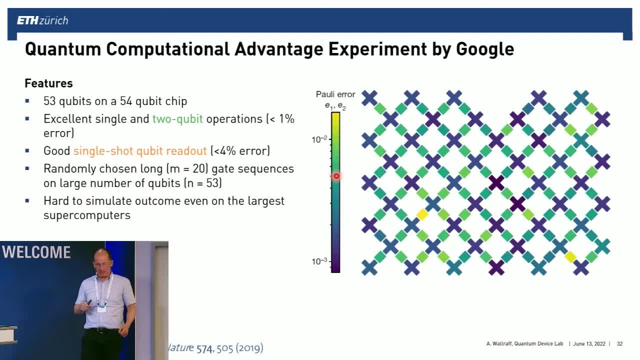 that it should have been realizing, the quantum computer should have been realizing. and look at whether you could have simulated that target state on a conventional computer And you compare how good that state is relative to the ideal state. If everything was perfect, if all the qubits were perfect. 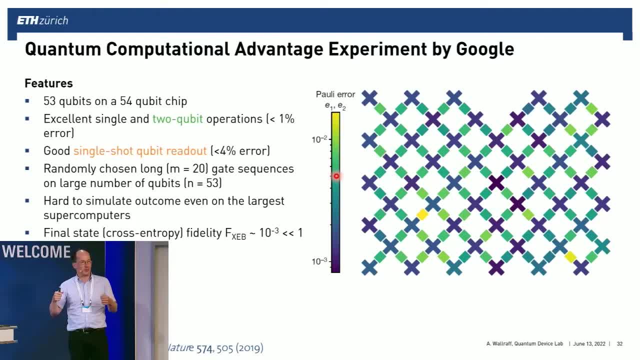 if all the gates were perfect, this ideality we would express as saying: okay, this state has a fidelity, and you wanted to have unit fidelity or 100% fidelity. So now, on this experiment, the fidelity of that state was 10 to the minus 3,. 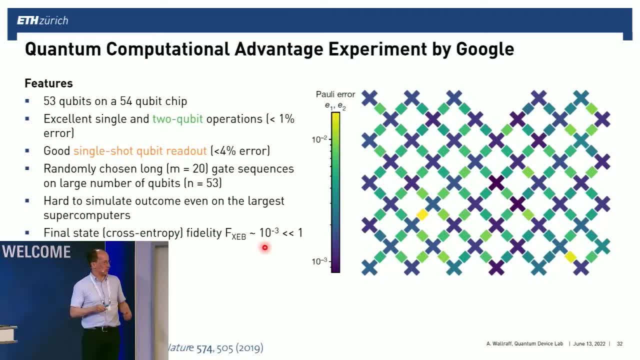 so that's 0.1%. So the state that was produced was not very accurately produced, but it was still very hard to simulate that state. Nevertheless, even if there was, maybe this state itself was reasonably far away from the ideal state. 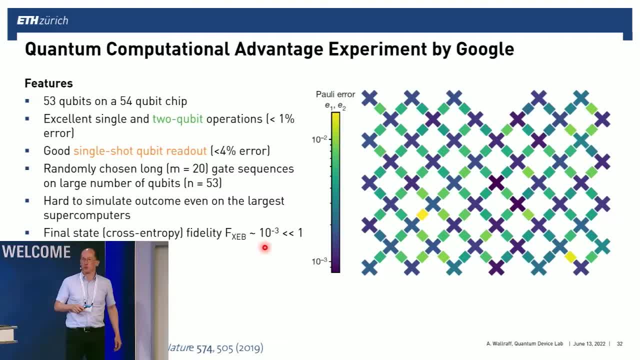 So in the end, if you want to use a quantum computer to calculate anything quantitatively, you want to do a quantum chemistry problem, for example. you want your problem also to be accurately solved. It doesn't want to be solved only a little bit. 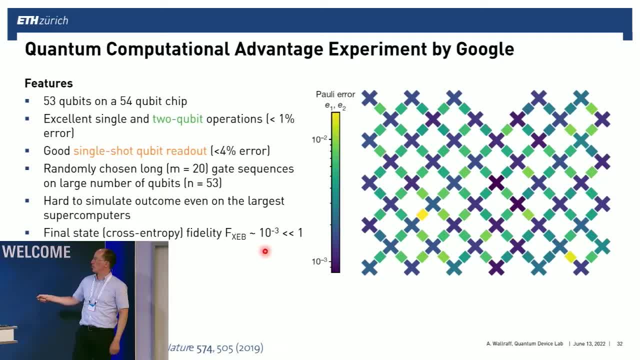 And so you have to deal with this problem here, that when you have gate errors that are partially induced by qubit decoherence, you probably have to mitigate them in some form to make sure that the final state that you create in your quantum computer is closer to the ideal state. 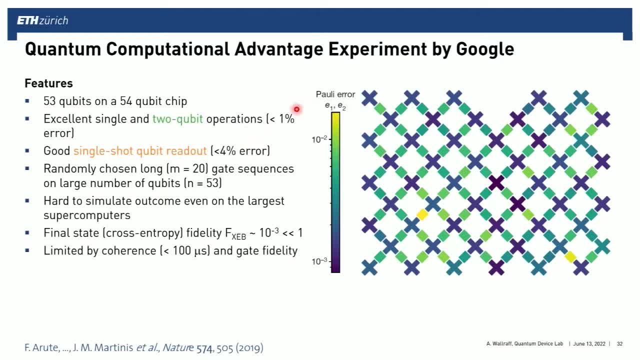 And in this case this was limited by a combination of the coherence times of their qubits, which were very good, and the gate fidelities that were limited by those coherence times but also by control errors. So in the end, 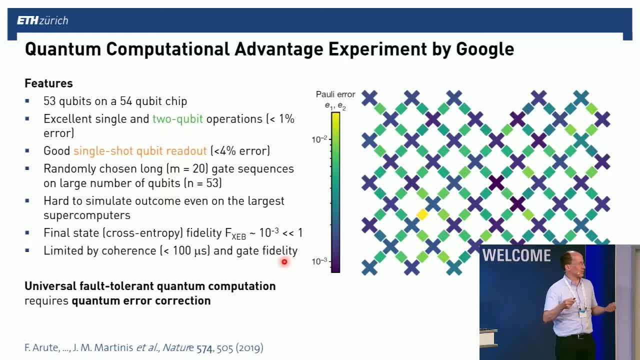 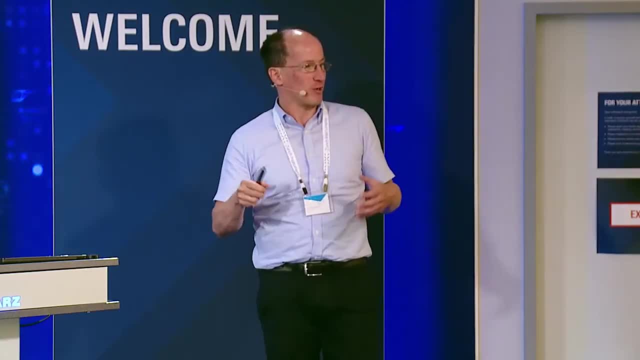 if you really want a quantum computer like that does universal quantum computation, I think many people would agree that it really has to be quantum error corrected And that's actually very challenging to do And the purpose of the talk today is to tell you sort of one of the fundamental steps. 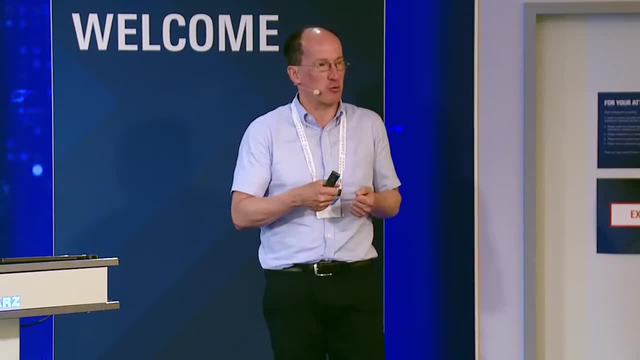 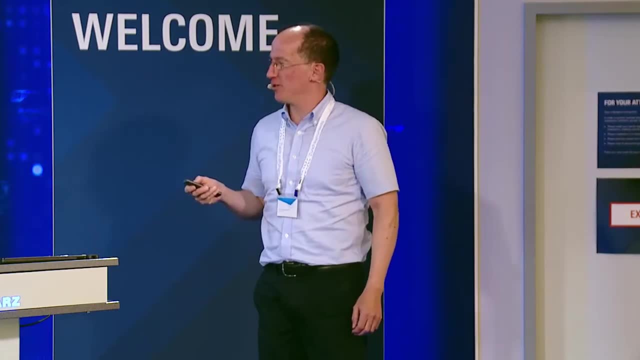 of how to error correct your quantum computer, first how you could possibly do it, and then how well it works. And then, once you see how well it works, you will also see that there's still much work to be done. Okay, so nevertheless. 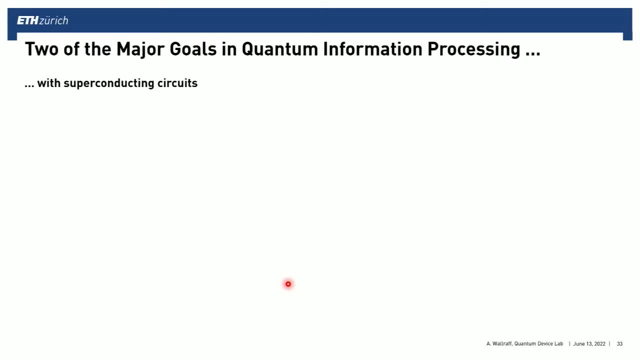 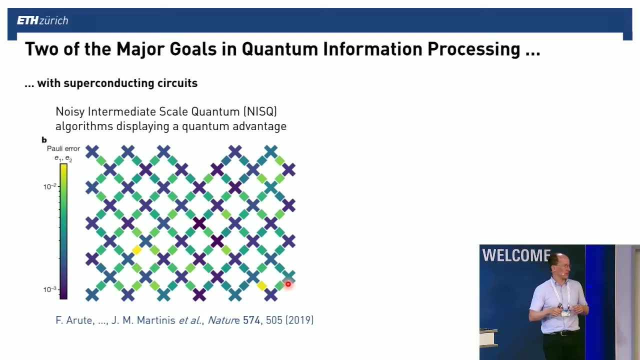 I think there's probably two strands in quantum information processing generally, but also with superconducting circuits. One, where you try to build the largest system that you could possibly build, take the largest number of qubits that you could get and run some algorithm on it. 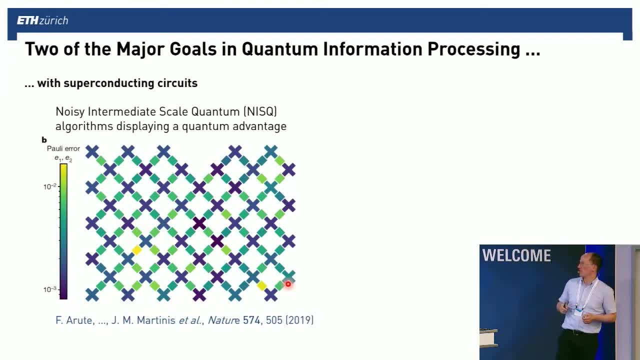 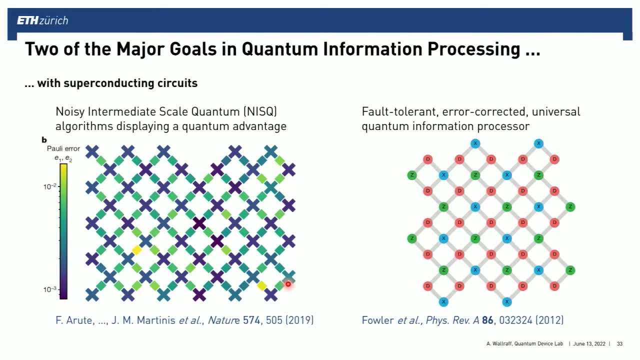 that is not quantum error corrected and see whether that's interesting and where you would get with that. And this Google experiment is in this category. And then the other thread of work is probably realizing: okay, you probably need to error correct your quantum computer at some stage. 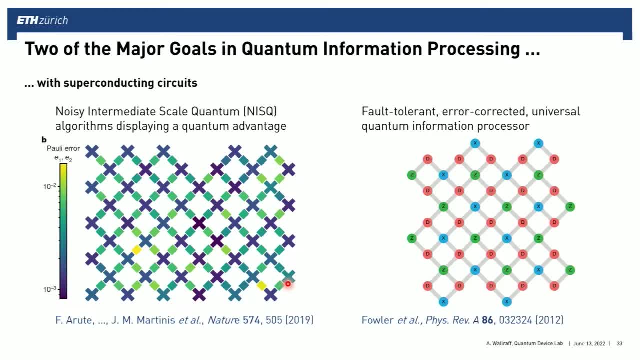 and try to go for that. And the problem with it is that for building error corrected quantum computers you will need to use a lot of physical qubits on your chip to encode a logical qubit on which you would do the error correction. So in some sense, 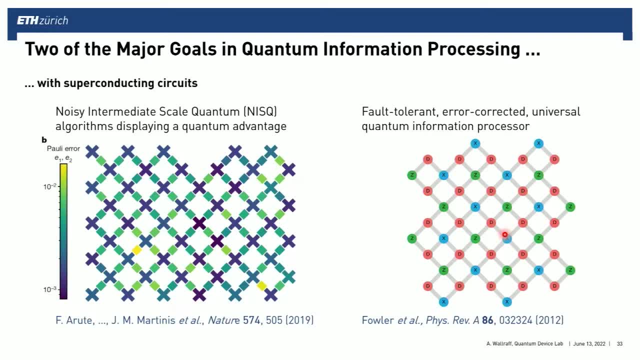 it looks like: oh, you take a step back, because now maybe you use a device that has about 50 qubits, So every dot in this diagram here represents a qubit, And you would use all these 50 qubits to make one logical qubit. 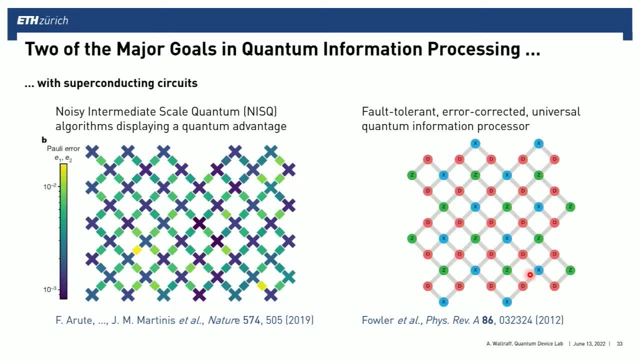 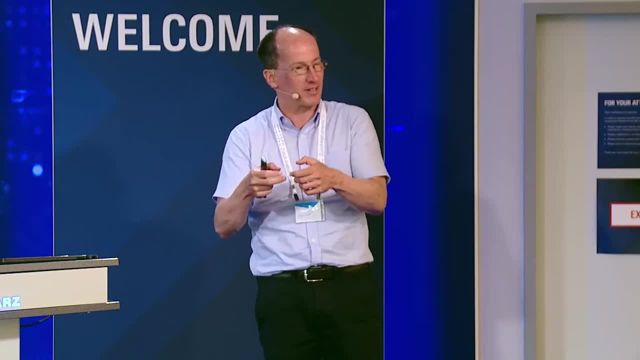 that you can then error correct, And if you do that successfully, in the end you have made use of these 50 and you have one logical qubit now, And with one logical qubit we will likely not yet do anything interesting. 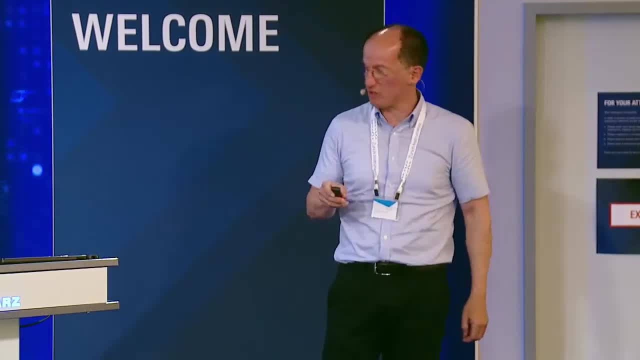 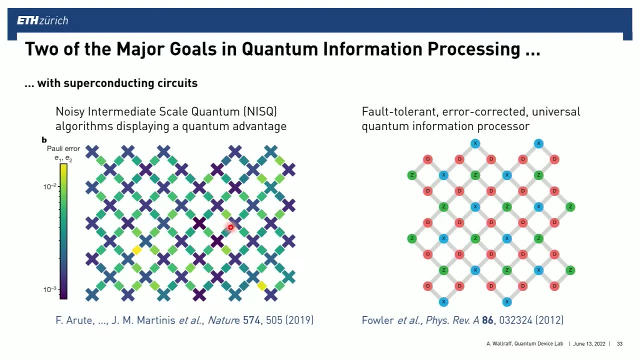 You need, then, maybe 50 logical qubits to start doing something more interesting, For example, repeating this Google experiment, rather than with 50 physical qubits. with 50 logical qubits would be nice, but that would require many more qubits to do. 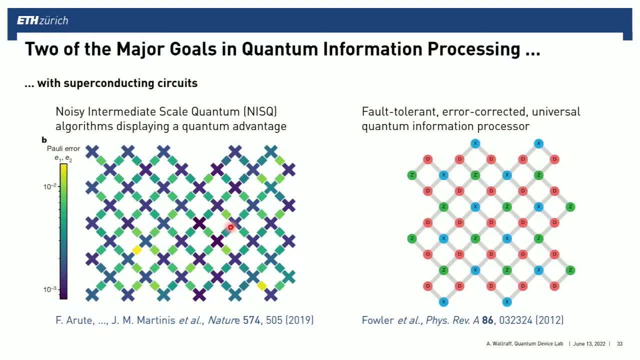 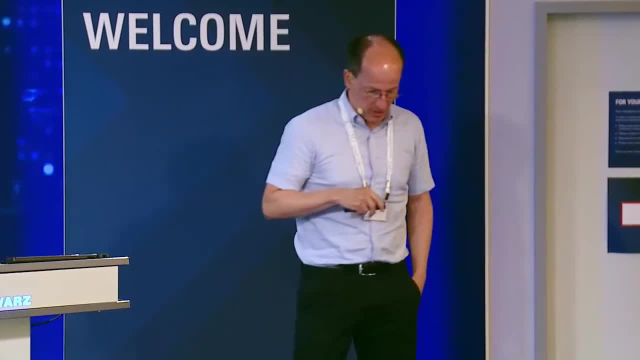 50 times 50, roughly, and maybe some more overhead. Okay, but these are the two strands that are followed in quantum computing with superconducting circuits. So we are going to be talking about error correction and maybe a caveat for the experts. 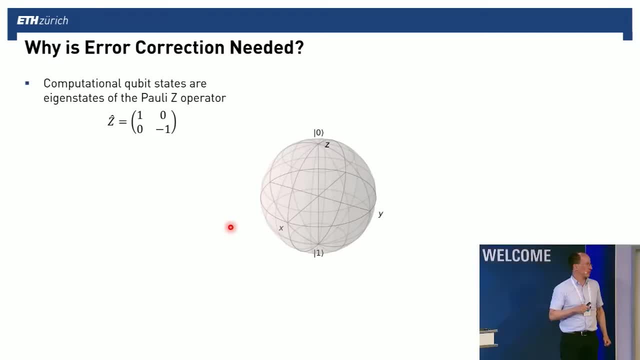 So there is maybe different ways how you could go to do quantum error correction in superconducting quantum computing systems. There is encodings that use qubits, where the quantum information is stored in a set of qubits, like of the physical qubits. 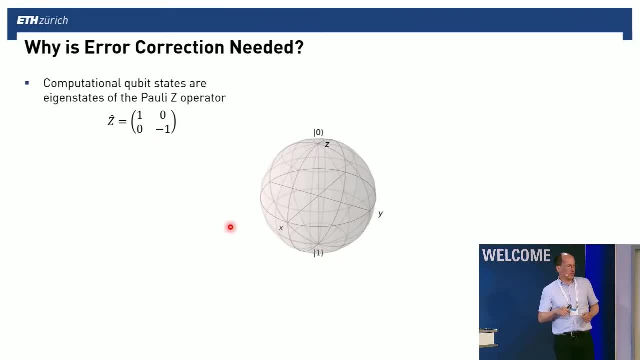 like transmon qubits that we would build, And there is a different approach that tries to store quantum information in harmonic oscillator states. So that is so-called bosonic encoding. So this is also very interesting and it is maybe at a similar state of affairs. 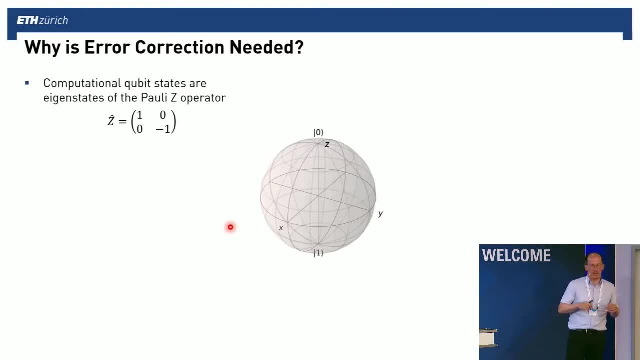 in its development And it, for example, gets worked on at Yale and at many other places, So that I will not talk about at all. So I will not compare these two approaches in superconducting circuits to each other. Okay, so I told you a little bit. 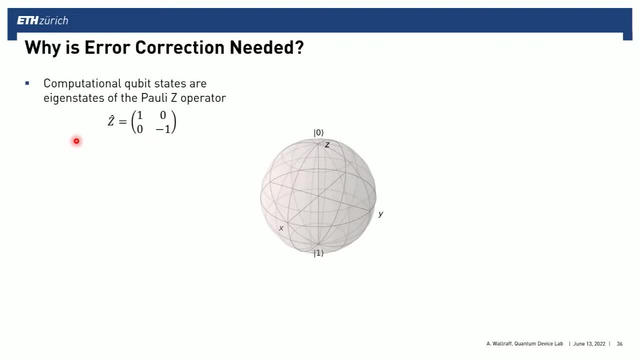 why error correction is needed And maybe one aspect that is special in correcting quantum errors in comparison to collecting classical errors. maybe classical errors like when communication systems were not that great. you needed to correct classical communication errors, looking at when zeros change into ones. 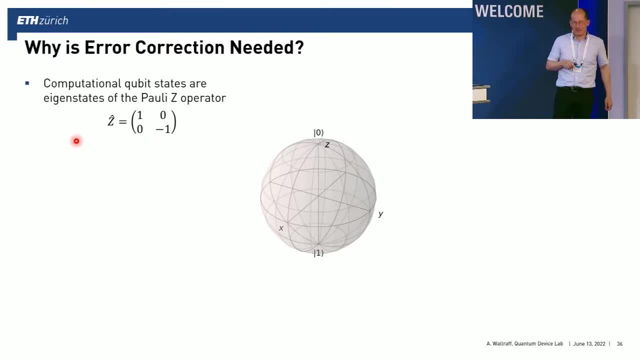 and ones changes into zeros, And there is lots of sort of classical theory and implementations for dealing with these types of errors. And in quantum systems there is not only one type of error, like a bit-flip error that turns zeros into ones and ones into zeros. 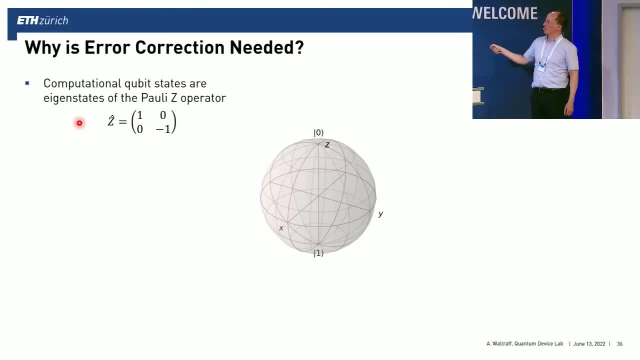 but there is also phase errors. So let us look at these bit-flip errors first. So in quantum computers you represent the individual quantum states, for example as vectors on a so-called Bloch sphere. So one of the things that you could do. 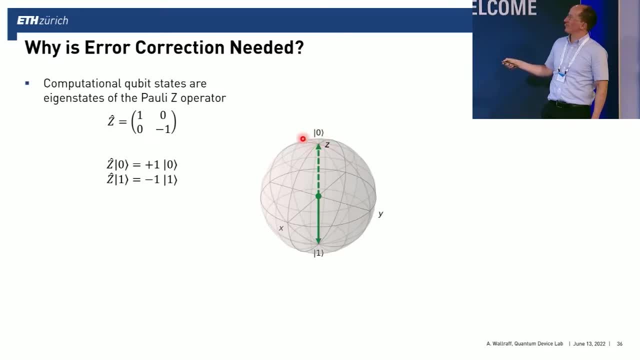 is, you could identify the logical or the physical, the zero state of your quantum bit as the north pole on this Bloch sphere and the one state of your quantum bit as the south pole of this Bloch sphere, And these two states are eigenstates. 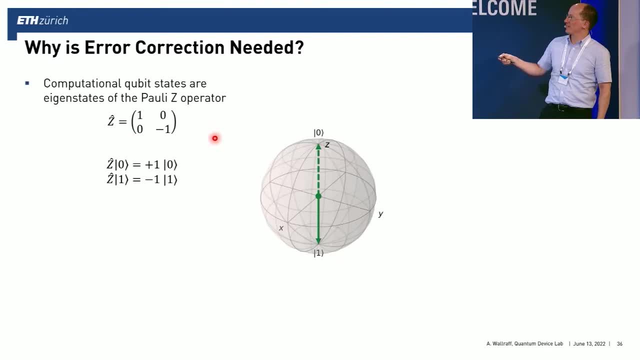 of this so-called Pauli-Z operator, which is representing the eigenstates of that operator, are the basis states for your qubit. So one reason why you need quantum error correction is that any quantum system couples to the vacuum fluctuations of the electromagnetic field in its environment. 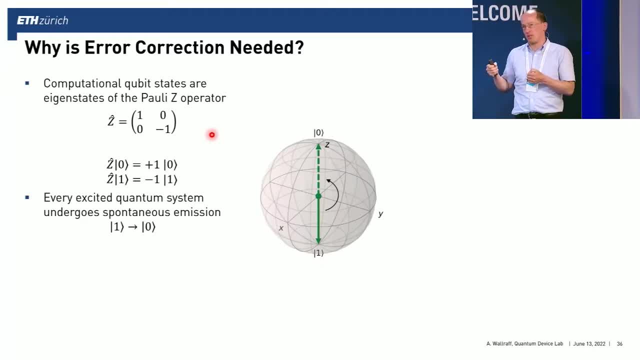 and that the dipole interaction between that quantum system and this electromagnetic field sets the rate at which excited states decay to ground states. So the process in which this Bloch sphere vector, pointing to the north pole, flips back pointing to the south pole, flips back to pointing to the north pole. 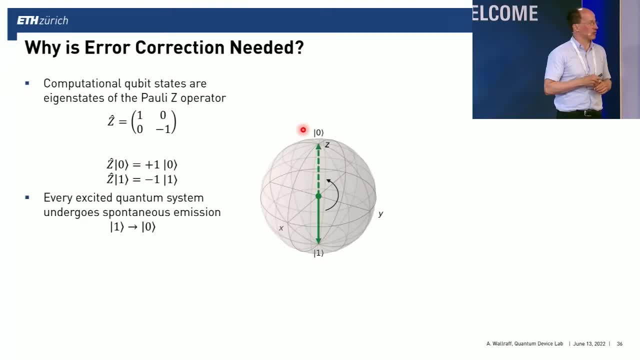 And that's unavoidable. And in the early days of quantum computing people were worried- or so is that the end of it already- That you would never get past this problem, And at the time it was not so clear whether you could even come up with an approach. 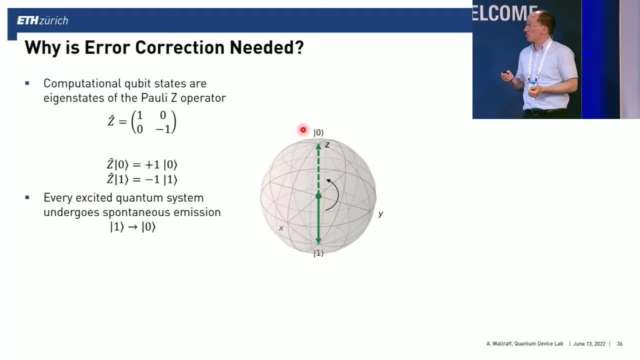 to fix that problem, And so it was really a major breakthrough to even theoretically realize that you could probably create an approach in which you could correct quantum errors successfully, And so that in itself is kind of pretty amazing when you think about it, And I'll say a few more words about it later. 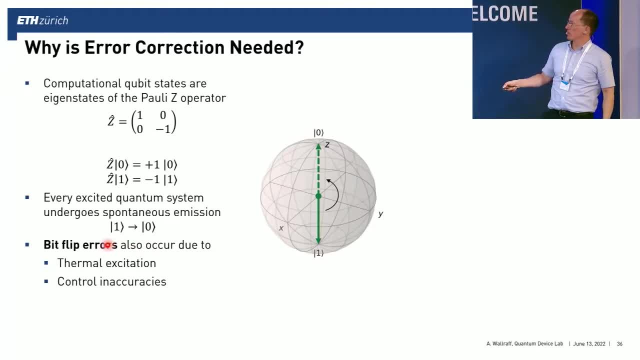 So these bit flip errors, they don't only occur because of this coupling to the vacuum, fluctuations and causing spontaneous emission of the qubit energy, but it could also be that zeros turn into ones because there's some little bit of thermal background, some thermal energy, in the environment. 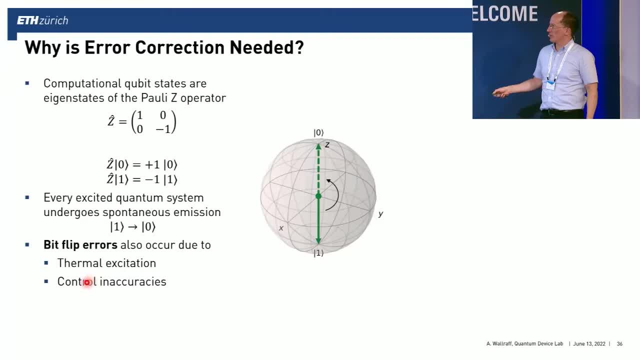 that brings qubits from the ground state to the excited state. And maybe even more importantly, and maybe at a place like this, it's very important to notice that the quantum computer is in some sense an analog driven machine, or so you apply analog control signals to it. 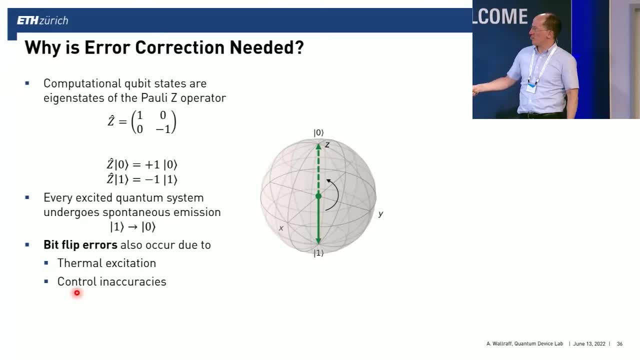 And even if you do very well and if you're at a company that knows about these things, you'll still make mistakes, Small mistakes, But these small mistakes will matter. But quantum error correction can actually help you against these small mistakes that you make yourself as well. 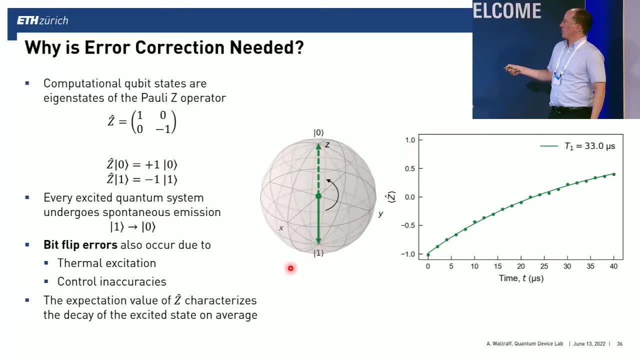 And then one standard thing that you do in quantum physics to measure how likely it is that these ones turn into zeros. you measure the expectation value of this Pauli sigma z operator, which gives you sort of the average of the quantum state that you encode in a single physical qubit. 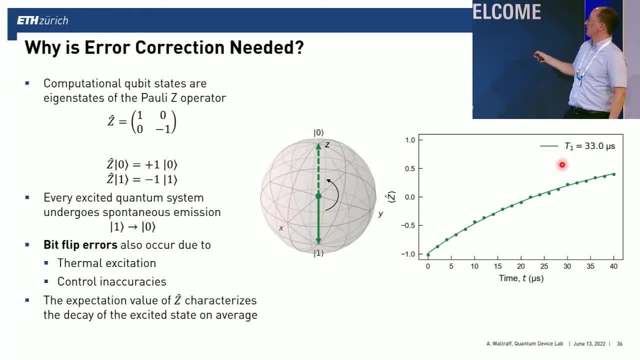 And you will see that that decays from the south pole to the north pole at some rate, and that rate is typically expressed as an energy relaxation time which, for the physical qubits on our device, is around 30 microseconds or so. So that's one type of error. 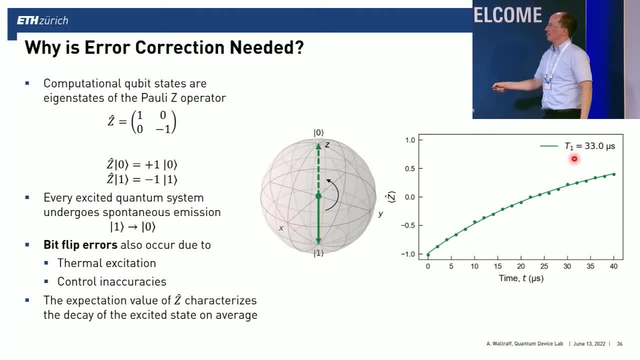 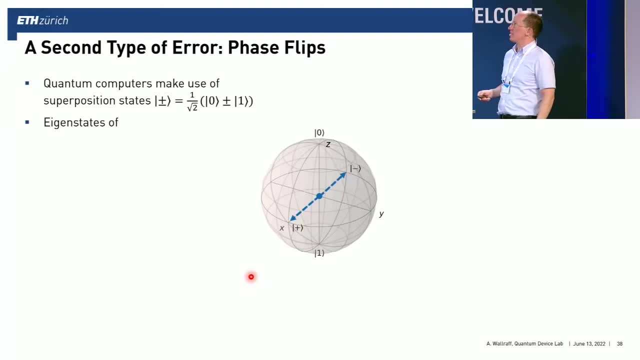 So bits are flipping from one to zero, and maybe they get thermally excited from zeros to ones, and if you're not perfect in controlling everything you will have control errors. So one type of error. So there's a second type of error, So in quantum computers. 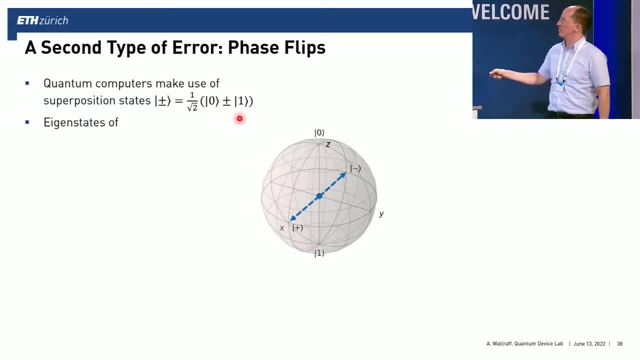 you make use of coherent superpositions of zeros and ones, and there's two examples given here where you make a coherent superposition of a zero plus one and one with zero minus one, and these states are eigenstates of the so called Pauli x operator and they point along this equator. 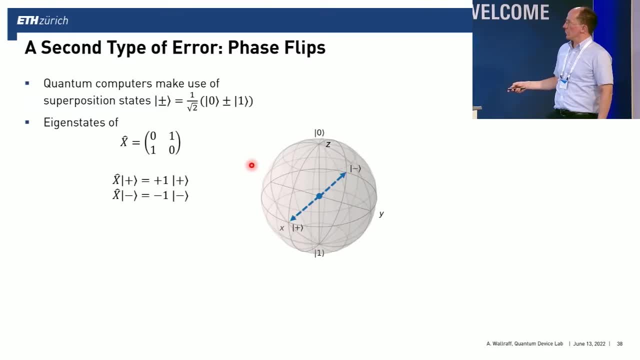 of this Bloch sphere here And same thing could happen there. there's reasons why errors could occur, Because something in your environment fluctuates in many. for example- I don't know if you know a little bit of atomic physics or spin physics- usually when you apply a magnetic field to a spin, 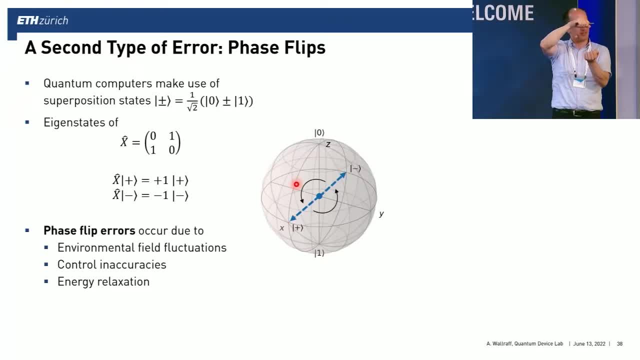 and that magnetic field fluctuates, maybe because you have a neighbor who runs their elevator or does a quantum hall experiment, or so then the transition frequency of your qubit varies a little bit and that changes the phase of these superposition states that you see here. 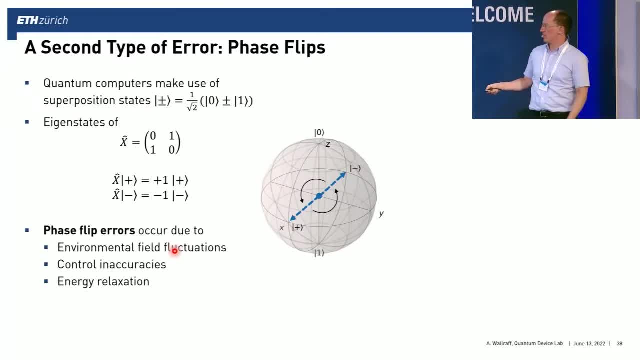 Or again, the electronics that you use has control of these frequencies. and also, if the one part of this state decays to the ground state, you will also mess up this phase, and that is a phase flip. So what is special in these quantum computers is that you have to correct for these two different types of errors. 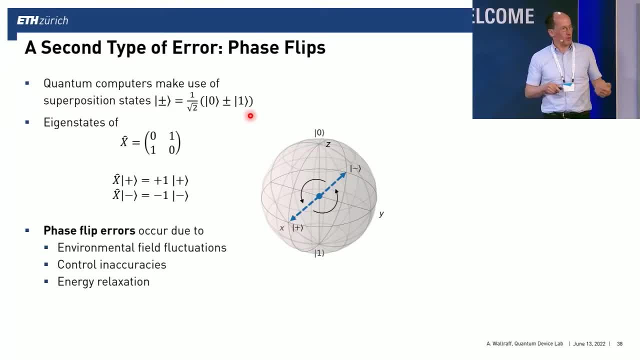 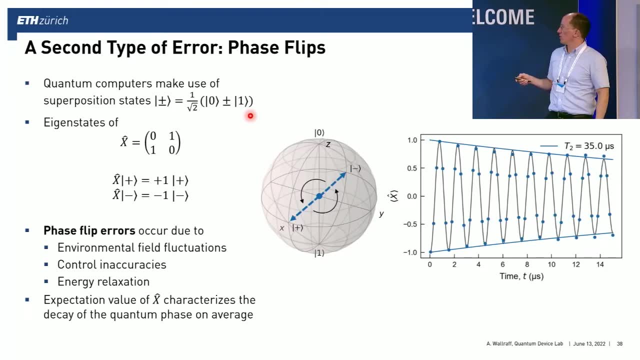 so bit flips and phase flips. So that makes it already more complicated in comparison to correcting classical errors in communications or in processing. And one way is to characterize how badly your superposition states are affected by these phase flips is to measure Ramsey decay times. 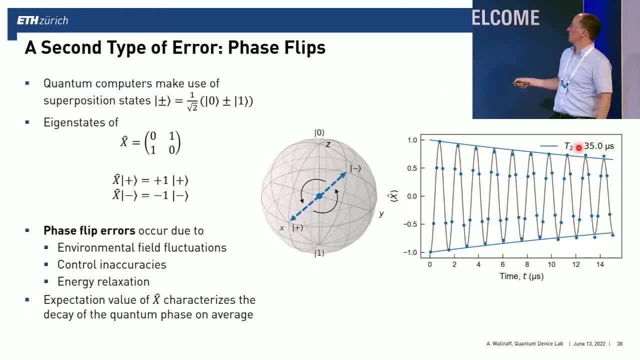 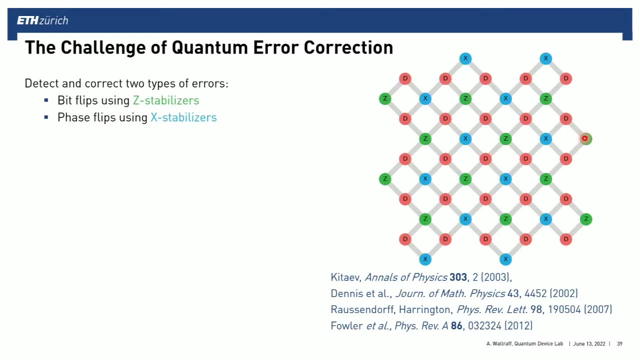 So here is a Ramsey decay time measurement for one of our qubits. It shows these Ramsey oscillations and the typical time scales are 30 microseconds. Alright, so these are the two types of errors that you want to be correcting in a quantum computer. 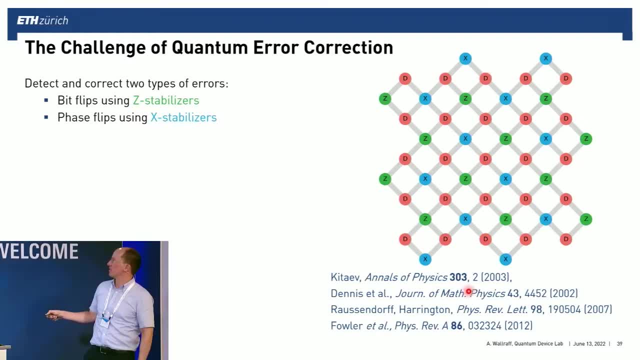 So the approach that I will be discussing is to use a set of physical qubits- so here you see, 49 of those- to both encode your quantum information in a clever way in the red ones of these 49 qubits, and those are then called data qubits. 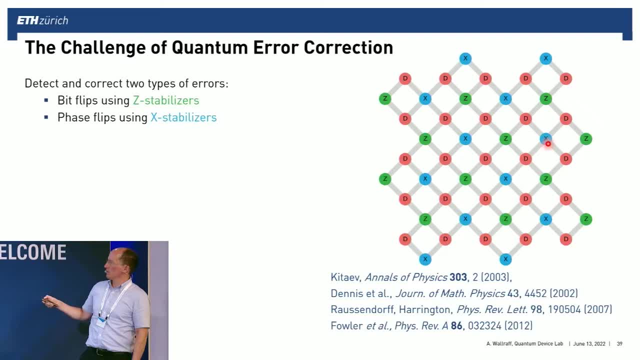 or code qubits and use the green and blue ones essentially to help you to detect errors successfully. And, as I mentioned, there are these two types of errors. there are sort of bit flips and phase flips and the green and the blue auxiliary qubits. they help you to detect either one of 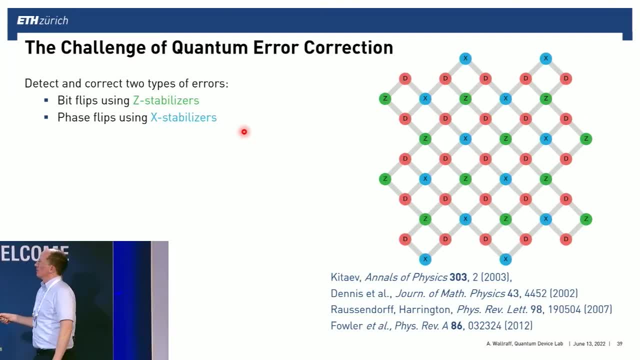 these two types of errors And then, once you will understand what this means, these green and blue qubits they implement so called stabilizer measurements. but I will explain to you what that really means. So one of the interesting things about quantum error correction is this fact that 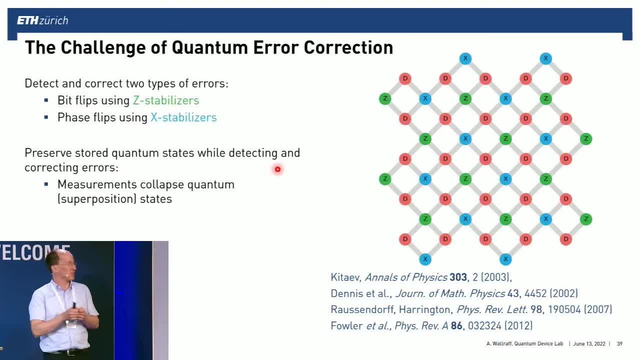 when you have a physical qubit in a superposition state 0 plus 1, when you go and measure it in its eigen basis, in the Pauli Z basis, then that measurement destroys this superposition state. so 0 plus 1 and you measure it, you will either get a 0 or 1. 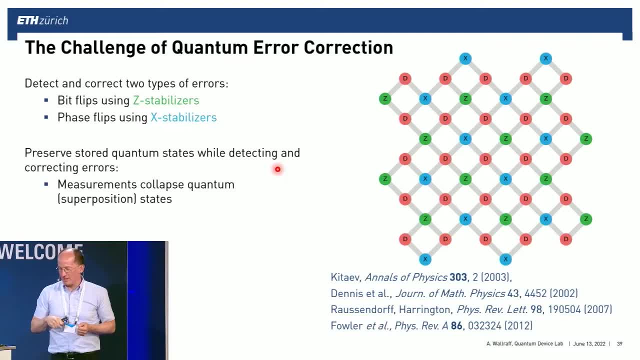 and afterwards it is dead, And so, therefore, it is like in quantum error correction. one of the challenges is: how do you perform even a measurement that looks at the state and judges whether an error has occurred without destroying the state that you were actually wanting to try to preserve through that? 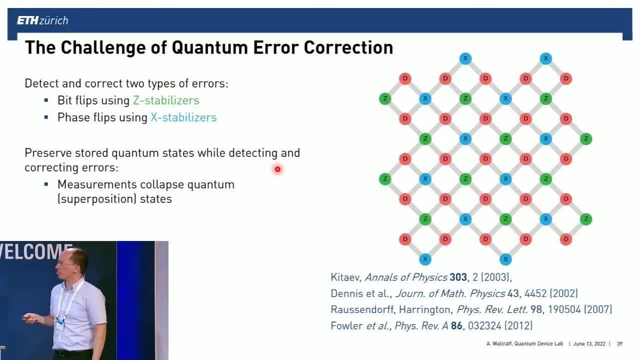 So you need to find a clever way how to go about that, Because measurements usually collapse quantum superposition states. So here the trick that is used is that one stores the quantum information in a logical qubit and that logical qubit is distributed over the many physical qubits. 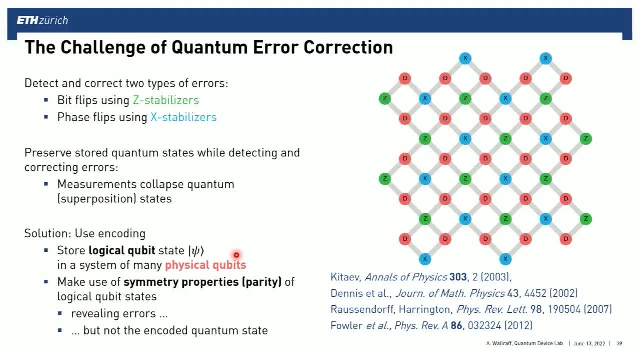 in this picture here. and then you come up with a clever way to store all the quantum information in these red dots, making use of a symmetry property of the red dots, and the symmetry property will be the parity of the quantum state encoded in the red dots. 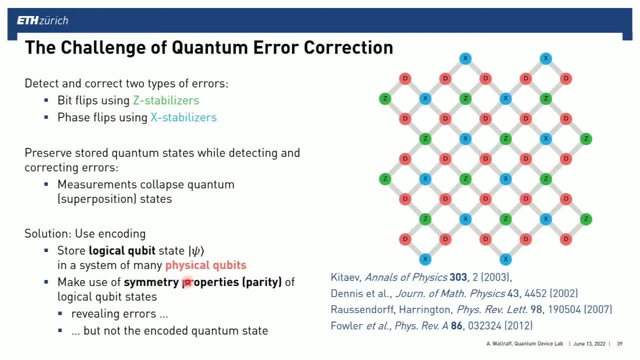 So the red dots will all be 0s and 1s and for example, if you encode quantum information in a situation where there will be an even number of 1s in this register of 25 red data qubits here, then you could check whether. 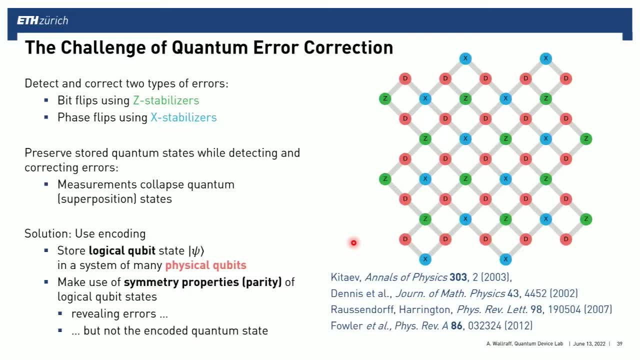 that number of data qubits in the one state stays even or changes to odd. For example, if it is even initially and there is an error on one of those qubits, that one qubit will go from 1 to 0 and now there is an odd number of 1s. 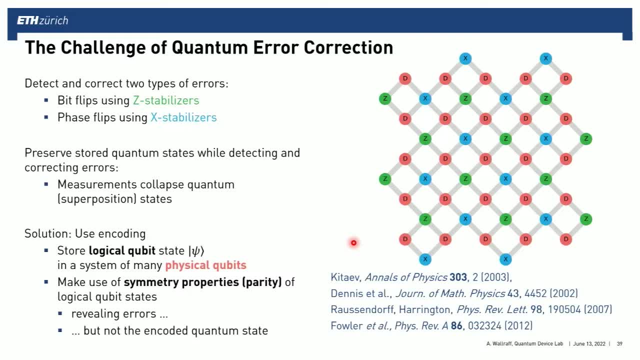 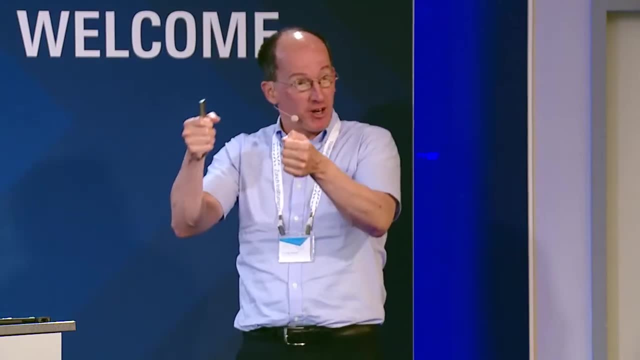 rather than an even number of 1s. Interestingly, what you will then do is you will try to encode your logical qubit in data qubit states which all have even parity, which all have an even number of 1s in them, and then, when you measure, 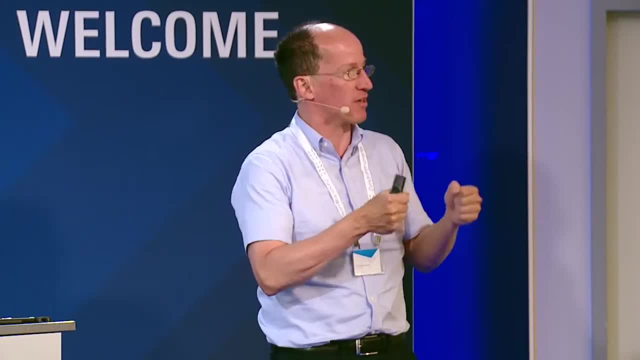 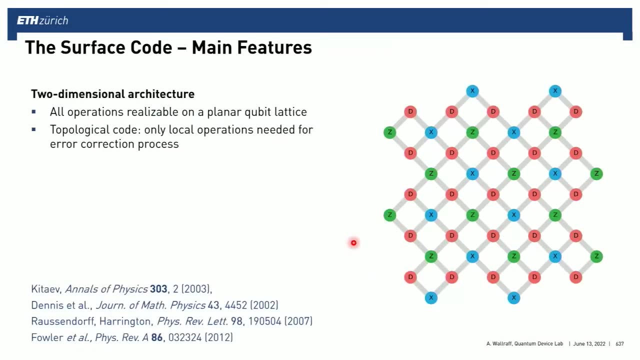 are there an even number of 1s? you can check whether an error occurred, but you will know nothing about the logical state that you have encoded, And I will give examples for that. Alright, so what we took for realizing this experiment is this surface code: 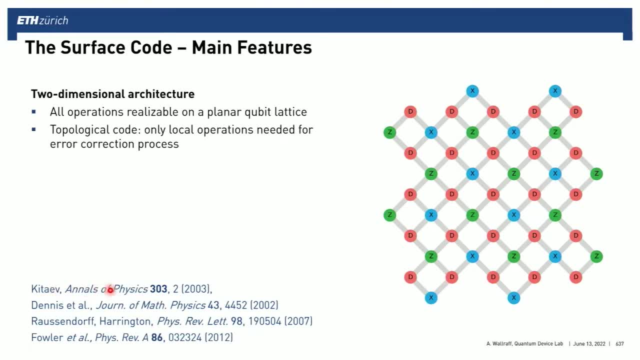 it has been invented by Alexey Kitayev and there is lots of history to it, so he was inspired by certain things that he learned, also from topological features of these systems, but maybe I will not say very much about it. what is special about this surface code? 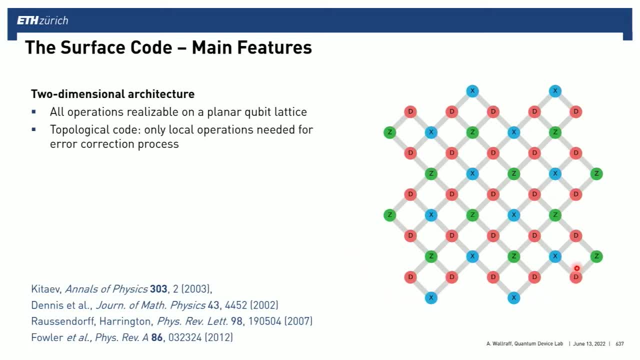 is that it is an encoding for quantum information that works on qubits and you can lay out these qubits in a plane art lattice like what you see here. and if you make qubits on a chip or so, that is good news. because if some theorist comes up and says: 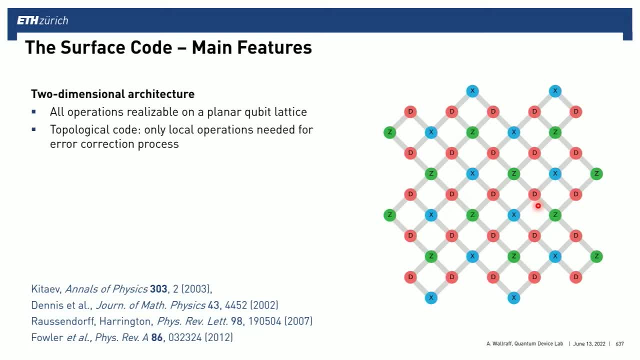 oh, you need to encode your qubits in some hypersphere or some torus, or so you maybe do not know how you will realize your qubits in a connectivity that is on a torus. so this is on a plane art lattice, and what is also special is that 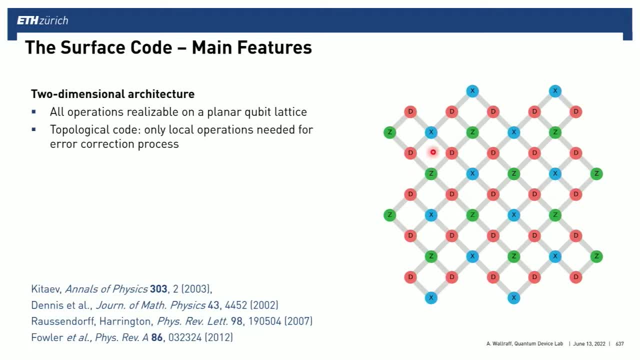 in case errors occur and I have not told you yet how you would note that an error occurred nor how you would fix it, you can actually correct for these errors by local processes, so you could check out where did the error occur and then you can do something. 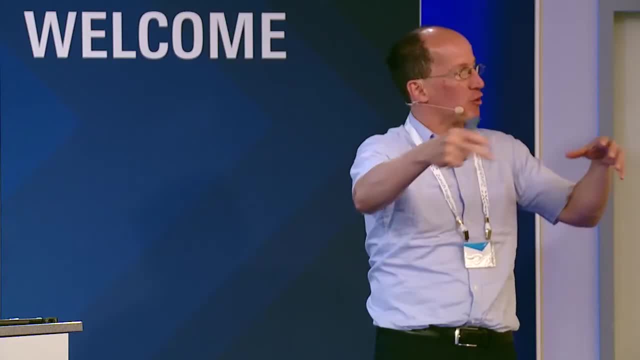 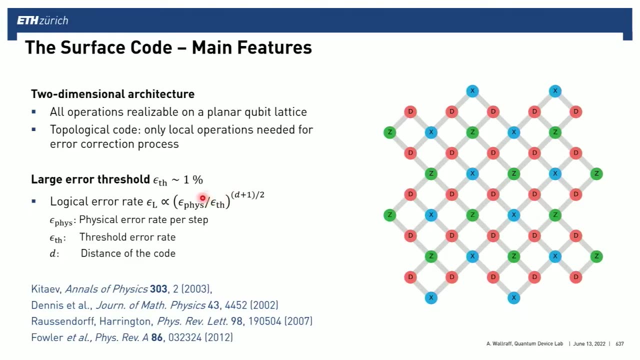 at the location where the error actually occurred and fix it that way, rather than doing something complicated on the whole set of qubits. and the other thing that is very good about the surface code is there is many other error correction codes for quantum information processing and they 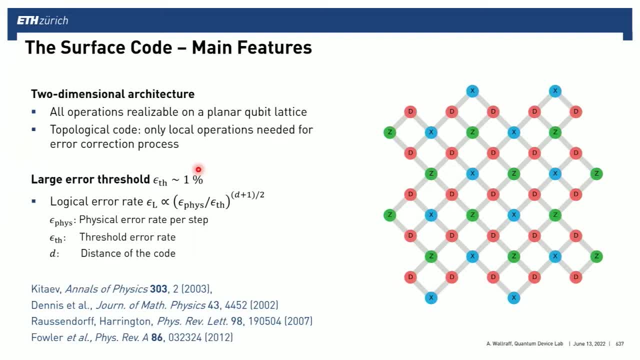 you can compare them against each other essentially by looking at how tolerant they are to physical errors in your hardware, and the surface code is the one code that has the highest tolerance to errors in the physical hardware, so it is still the best known code that you can have that tolerates the highest. 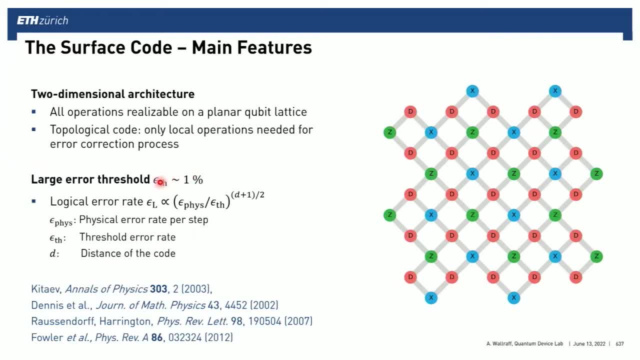 level of errors in your hardware and that defines a so called threshold and maybe some simplified model. this threshold is about 1% error in every component of the hardware that you use for implementing the surface code. so what that means is if everything on your hardware is better than 1% error. 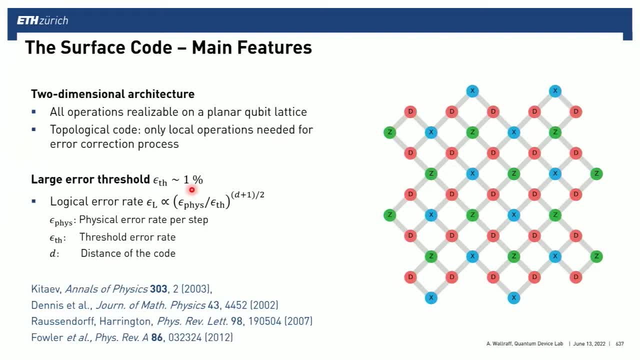 you will probably make the surface code work, and in the end it is a benefit for the quantum computer. and initially the early codes were way worse than that, so maybe they had a threshold of 0.001% and that would mean it would get even much better. 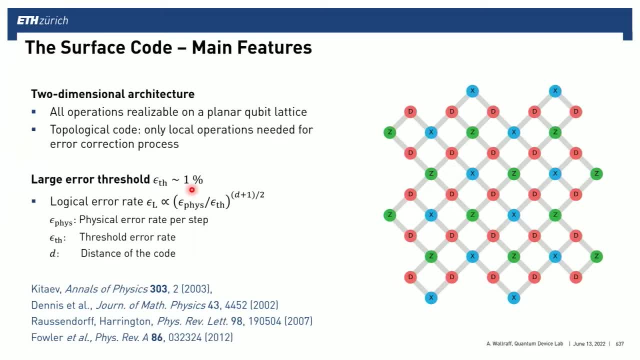 than it is now to even start trying to implement error correction in this encoding. so that is why surface code is important and I think it will be for anyone who lays out their qubits in a planar lattice or spins or superconducting circuits. they will need to look at this type of code. 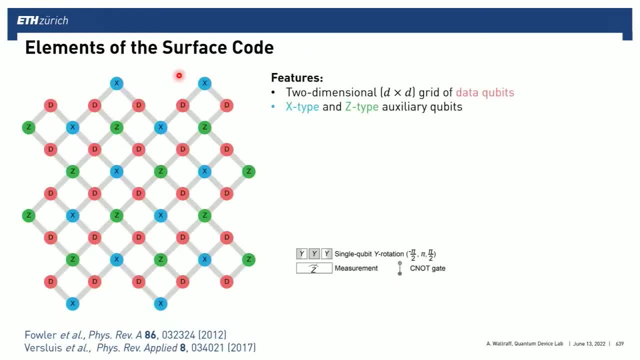 and there is nothing better currently. good, so. so what are the elements of the surface code? so there is a lattice here with 25 data qubits or code qubits in a 5x5 grid, so that is called a distance 5 surface code. 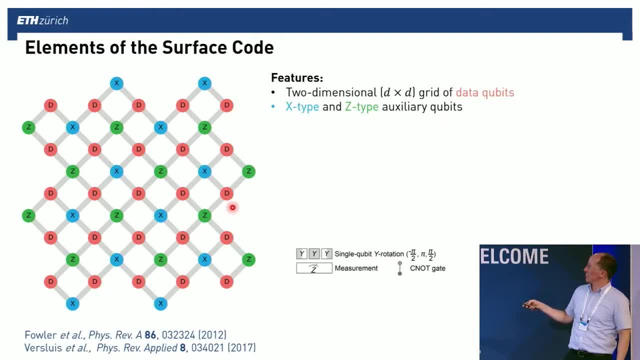 maybe you will see later where it has this name from. and then there is these blue and green auxiliary qubits that you see here and these grey bars that you see between the blue and green qubits and the surrounding data qubits. these define a so called 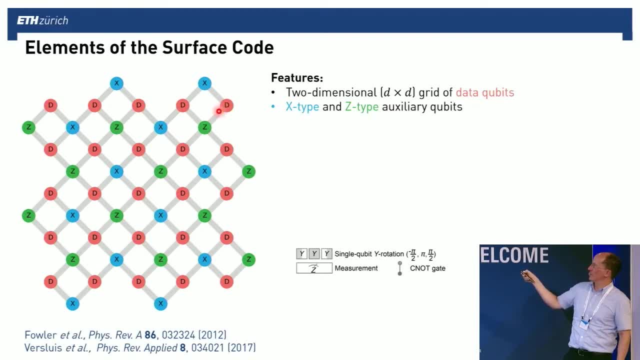 pliquette. so let us maybe look at this set of data qubits here. so there is four data qubits that are linked by a grey bar to this z-type auxiliary qubit, and this z-type auxiliary qubit is actually used to measure the parity of the four data qubits. 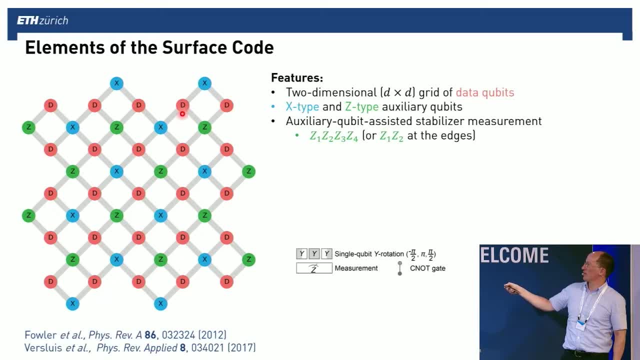 that it connects to on such a little square here which is called a pliquette. and one way: if you are a theorist and you like to think about it this way, one thing that you can think about the auxiliary qubit to measure is the product of the Pauli z operators. 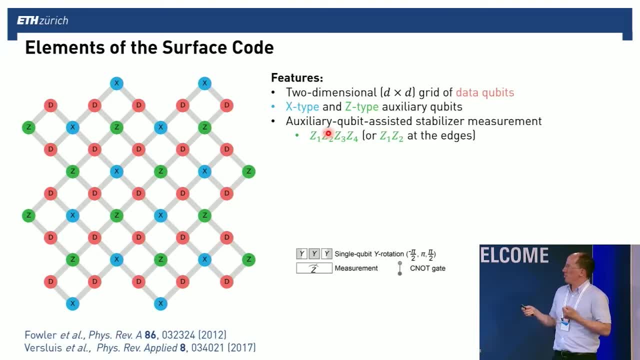 of these four data qubits that lie around it. but maybe that is not the most intuitive thing, but maybe a more intuitive thing is to say that this z-type qubit it measures, it tries to determine whether an even number of data qubits are in the state 1 or not. 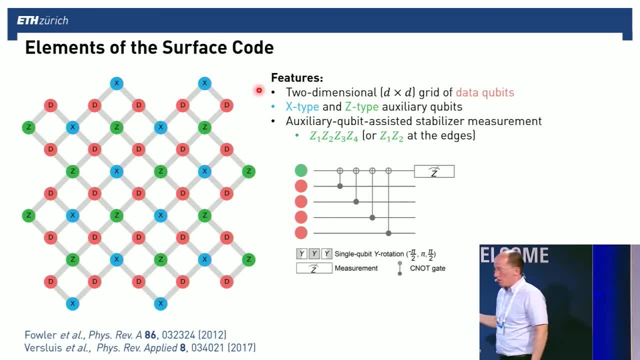 and I will give you a basic example for that in a second. alright, so here is the auxiliary qubit, the z-type one, and then there is four data qubits that are coupled to it in this pliquette, and we try to figure out this parity by applying. 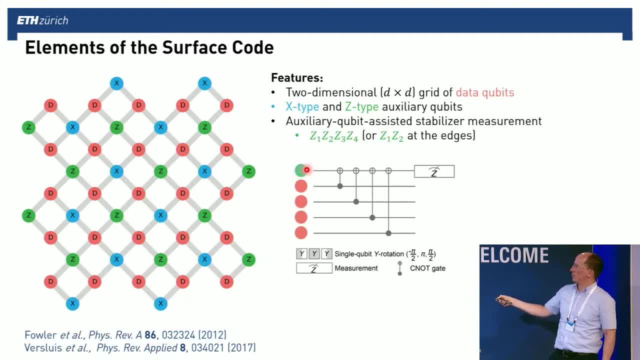 some gates to this, between the data qubits and this auxiliary qubit, and what you essentially do is you run four: two qubit gates that are known as CNOT gates. so these are the symbols for CNOT gates. subsequently between first data qubit, second data qubit, third and fourth. 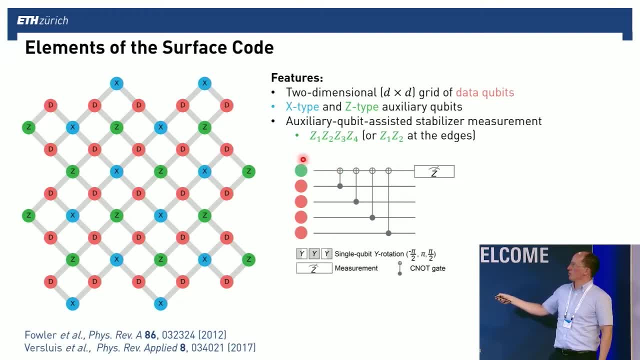 and this auxiliary qubit, and that allows you to to see from the state of this auxiliary qubit whether the data qubits were in an even parity, and on the next slide I will show you a specific example for that. so in a quantum computer, since there are not only 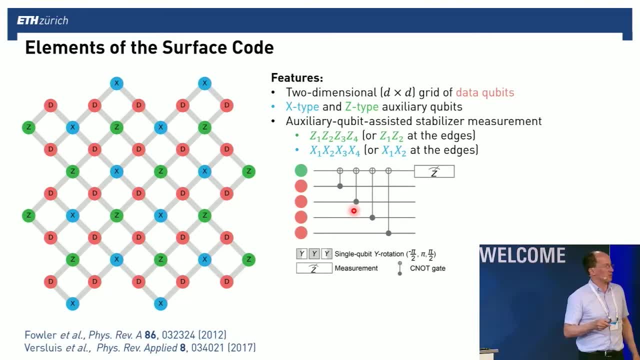 bit flip errors, but also phase flip errors. that is not good enough. so you need to do that also for these phase factors, for the plus and minus ones, and luckily this is very easy to do because it is essentially almost the same. you see here. it is the product of: 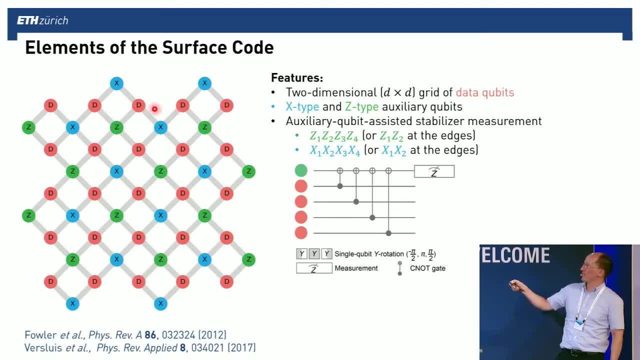 four x operators. so you take another plaquette. here there is again four neighbors and you try to measure this, and it essentially works in the same way as here. the only thing that you have to do is you have to do a basis transformation on your data qubits. 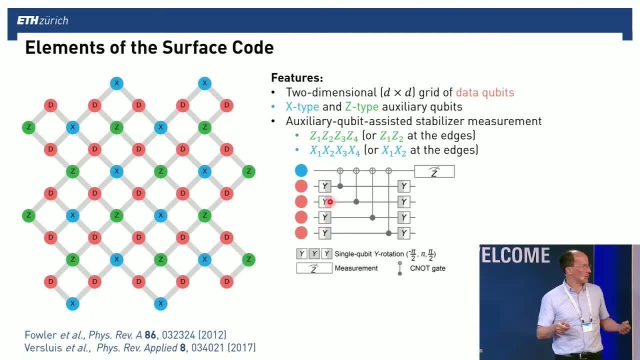 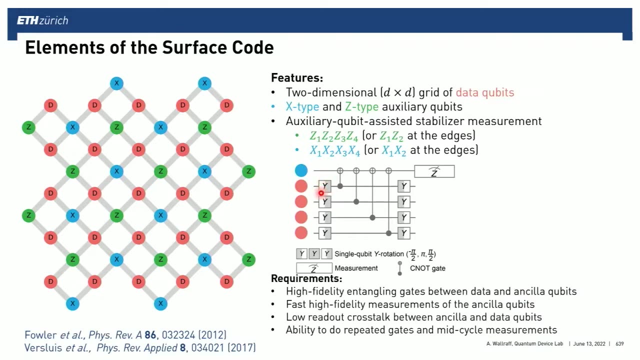 so you apply a pi half pulse to every one of your data qubits initially, and that flips the basis. so everything that was a north pole is now on a superposition state, and vice versa. and then the same gate sequence now measures um the parity, so that, whether the 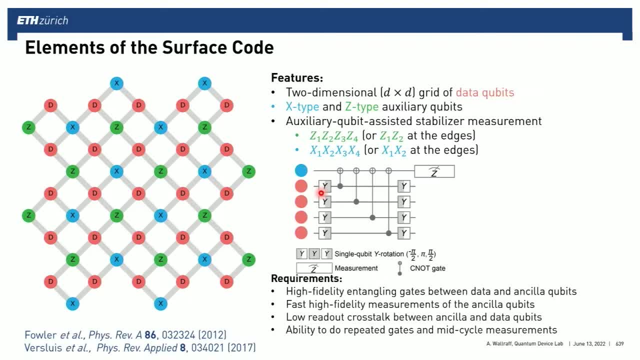 whether there is an even number of pluses. but in this other basis, okay. and so what the quantum computer does in the surface code? when it does error correction, it essentially all the time measures. these parities it tries to look at all the time are: is there an even number of ones? 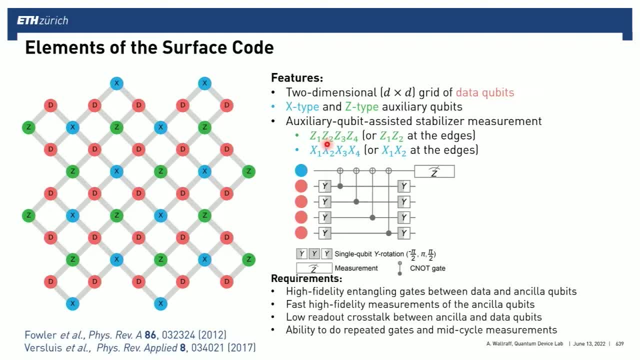 and an even number of pluses all the time. and for that to work successfully, you have to make sure that that the errors that are introduced by doing these two qubit gates, the single qubit gates, and this measurement on this auxiliary qubit that you need to perform to figure out whether 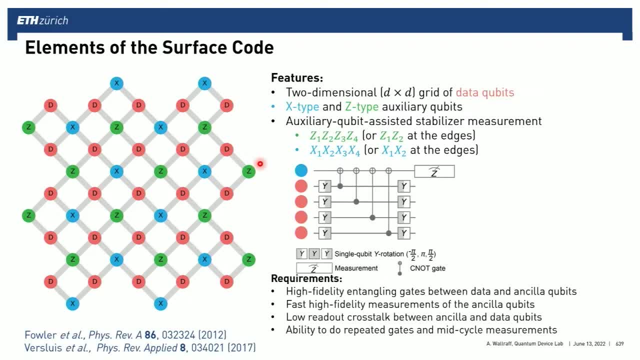 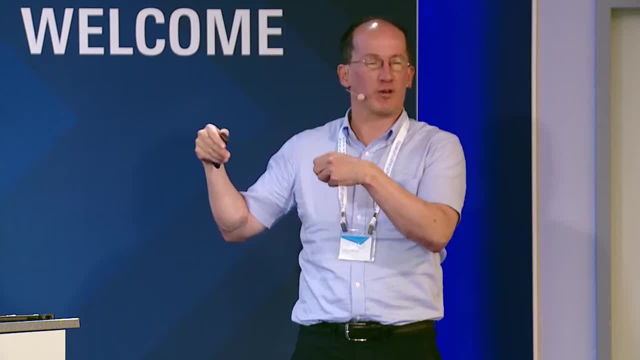 an error has occurred or not. these all have to be pretty good, and it's this threshold that I mentioned. so every one of these operations needs to be at least with, or with a with an error not larger than one percent, and if that's the case, yeah, then this has a chance of succeeding. 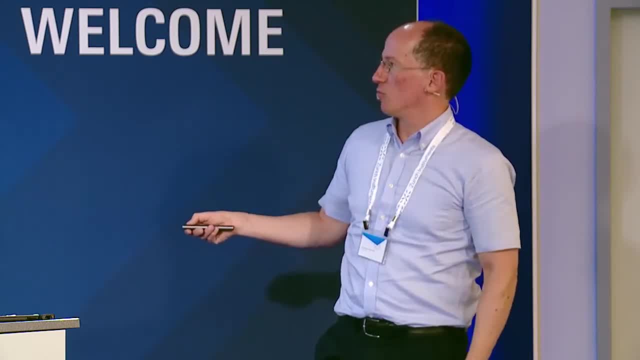 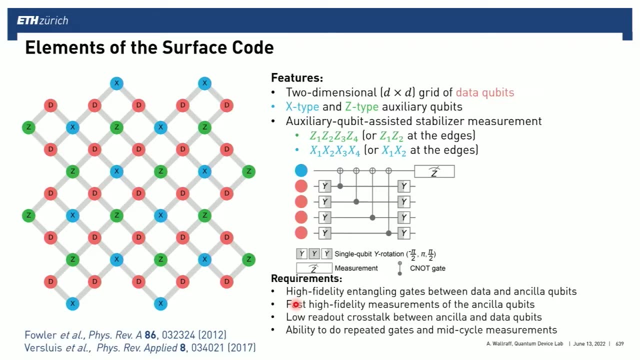 in making the logical qubit better than the physical qubits. um and- and this is challenging- for example, in this, in this example from the google quantum advantage work: there you saw the readout had four percent error and therefore with that readout they would probably not get this. 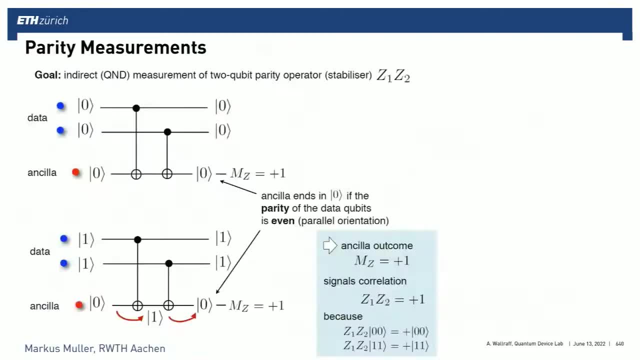 surface code to work well enough to actually be successful. good, so here's my basic example. so how does this work as a parity measurement? so I told you, a parity measurement means an even number of ones in your data qubit register. and here I did the even simpler example, not with 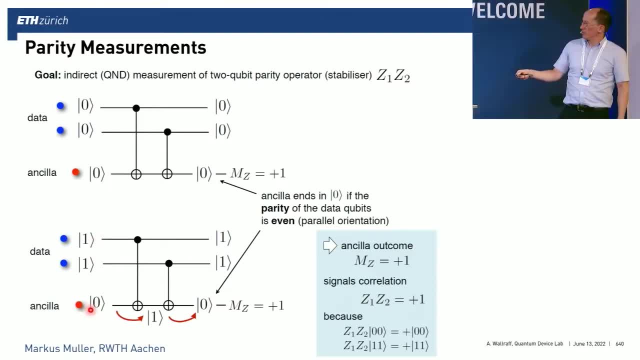 two data, with four data qubits but with two. so if you start with your helper auxiliary qubit in the ground state and now you apply two c knots subsequently between the data qubit and the and the auxiliary qubit, so every time the data qubit is 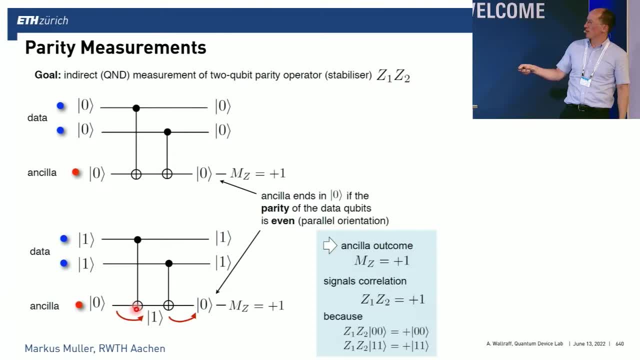 in one. the auxiliary qubit will flip the state from zero to one or from one to zero when this gate gets enacted. so when both of the data qubits are in one, you, the auxiliary qubit goes from zero to one and then back from one to zero, so effectively it remains. 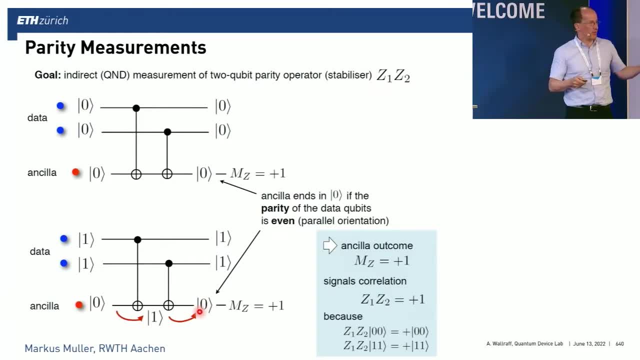 where it was, and and then that indicates that the parity was even so. there's an even number of ones, and now you could imagine, say, if you had more data qubits, like four, and all of them are in one, or then the auxiliary qubit goes zero one, zero one. 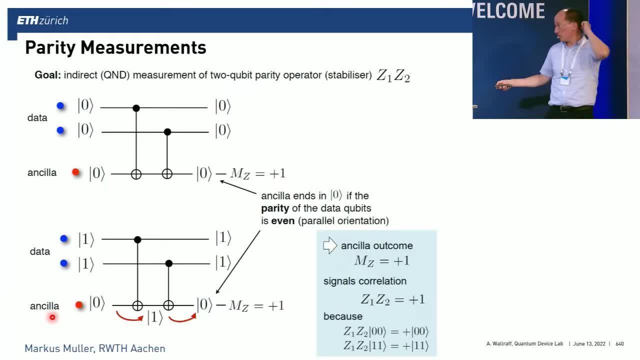 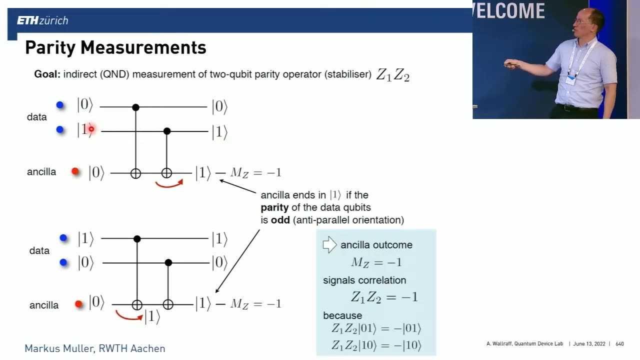 zero and be back where it was, and that indicates that you have an even parity state. and when the data qubits are in state zero, these c knot gates do nothing. they don't even act on on the auxiliary qubit but say: if now, say, one of the ones turns into a zero, 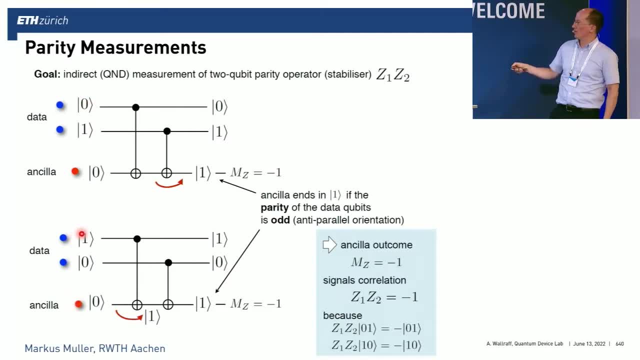 like here, or one of the zeros turns into a one. now you have an odd number of of two qubit c knot gates that act on this auxiliary qubit, and therefore your auxiliary qubit goes from zero to one and that tells you: hey, there was an error. 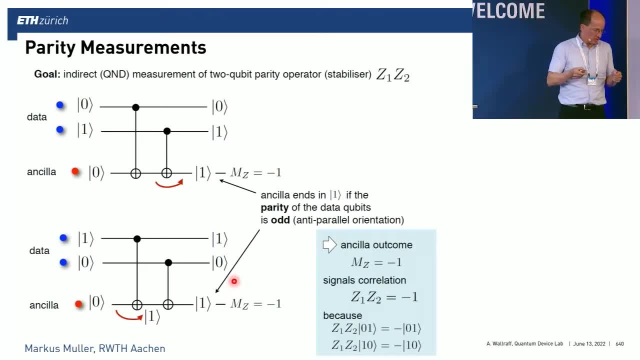 so now your parity has changed from from even to odd. and the trick is really encode all your quantum information in even parity states and use these, these auxiliary qubit stabilizer measurements, to figure out whether the parity has changed. and that's what it's about, good. 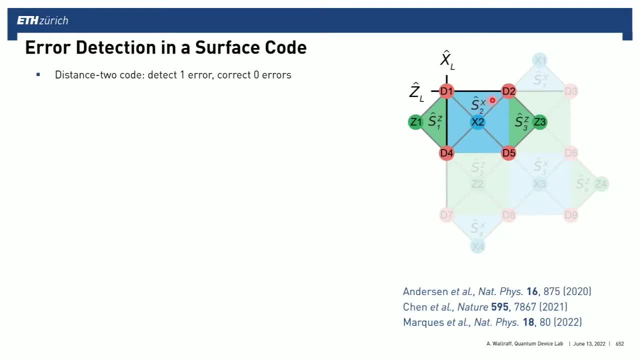 all right. so there's. there's one sort of basic example, so i showed you before. you saw this big grid with 25 data qubits. so here's a tiny grid with four data qubits and three auxiliary qubits, and here you can. so there's these. you measure parities. 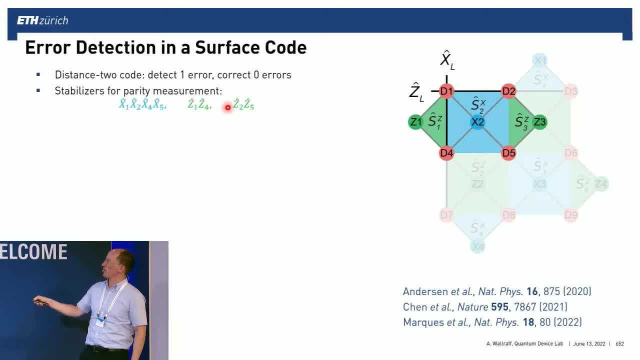 and the x and then the z basis. and here's this product of these parity operators are written down here and maybe you don't need to worry about that, but they all commute with each other and the fact that they commute means that they have common eigenstates. 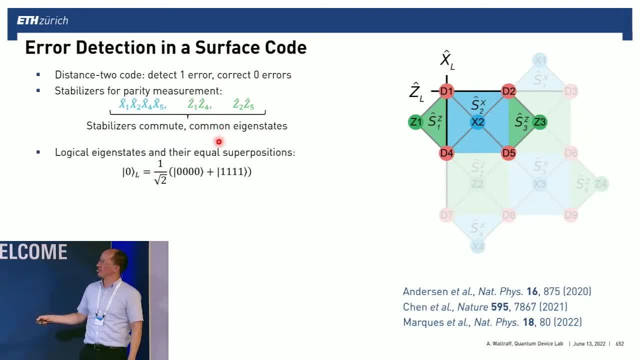 yeah, and, and here's some examples of these common eigenstates. so actually in such a device you would now encode the logical zero as the superposition. four zeros with four ones, so that's clearly an even parity state. so now you can turn that into a logical. 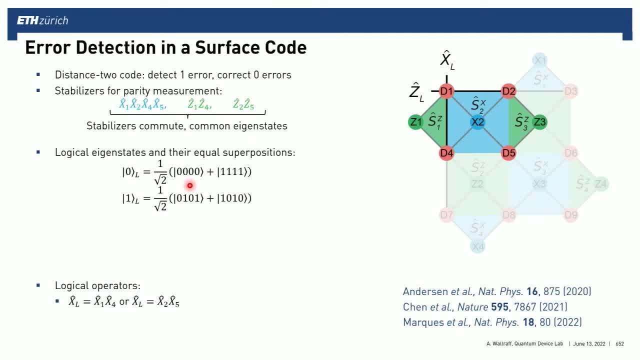 one by flipping, say, two of the qubits, say the first and the third one, and if you flip the first and the third one from a, from either a zero to a one or from a one into a zero, you end up with this logical excited state and you look at it. 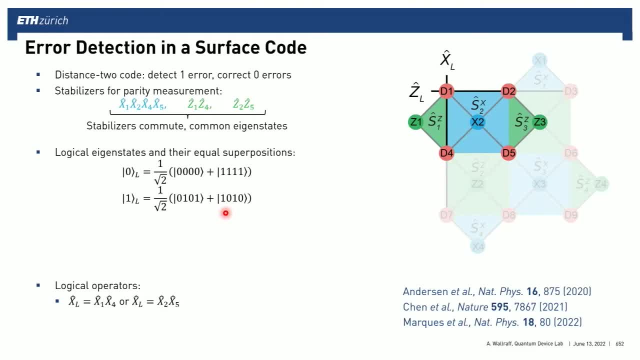 and you see there's still an even number of ones. so that's still an even parity state. so your parity measurement will not be able to tell are you in a zero or are you, are you in a one, and that's exactly what you want. so then, if you want a logical 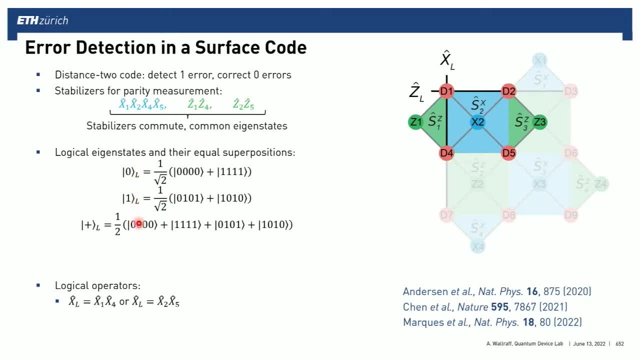 superposition state. you just make a superposition of zero logical and one logical and you look at it and you see, still, every component has an even parity and minus superposition state. you can. you can create by, for example, every time you have only one of the 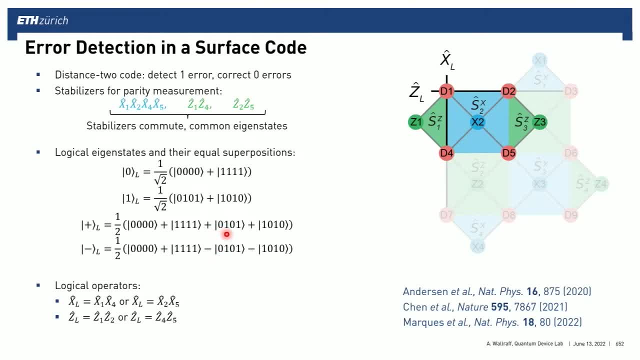 first two qubits in the one state, you flip its phase and that creates this logical minus and you look at it. so now there is four distinct states that you encode your quantum information in, but they're all even parity. yeah, i guess now you got it, and uh, so this is a little bit of a 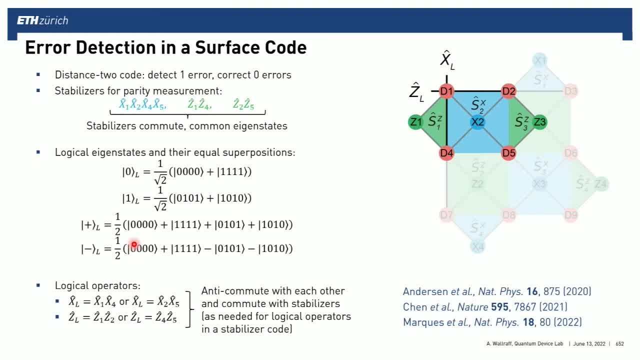 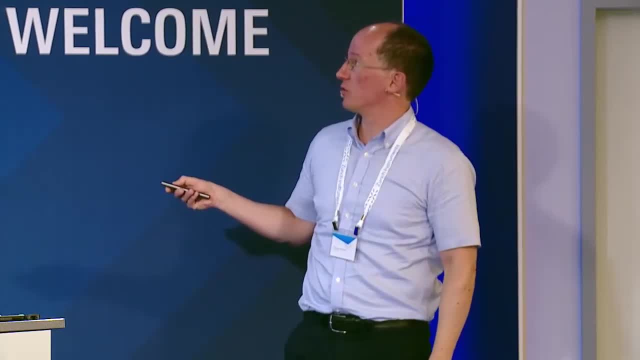 this is how this works, and, and you extend that to larger and larger sets of qubits, you do the same approach with nine qubits, or with 25, or with larger sets of qubits to encode quantum information, and so the experiment that we were happy with. 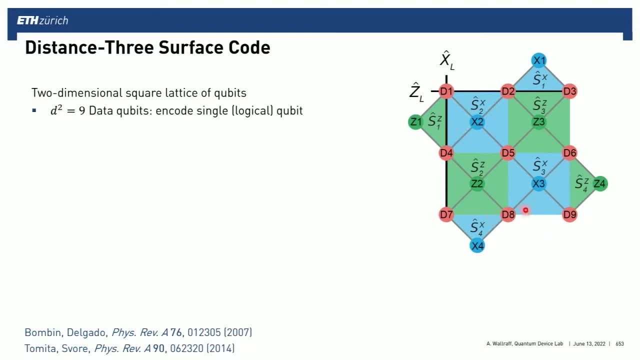 having done is to do this on a on this three by three data qubit lattice and uh with uh. so there's nine, there's nine data qubits here and uh. so this is actually the. the d is called the distance of a surface code, and that also relates to the number of 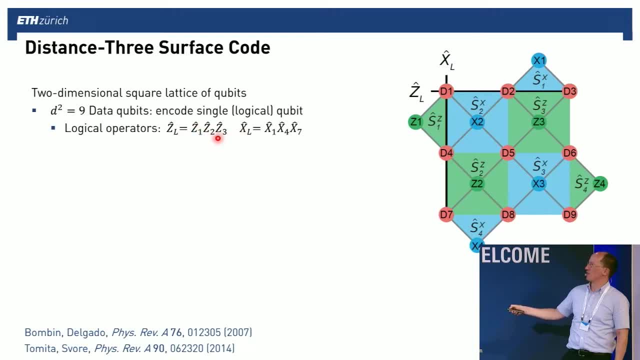 operators that you need to change the state of the logical qubit encoded in this surface code. so here the. if you want to change your logical 0 to a logical one, you need to apply three local pauli z operators to three of these data qubits. so in this case you would, if 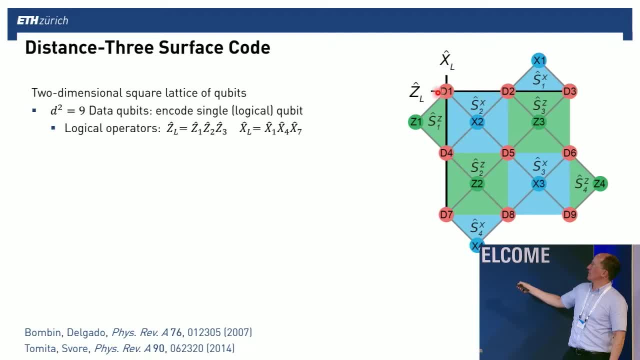 you apply a z operator to d1, d2, 2D3,, you will change the phase of the logical state. If you apply an X operator to X1,, X4, and X7,, you will flip the logical zero to a logical one. 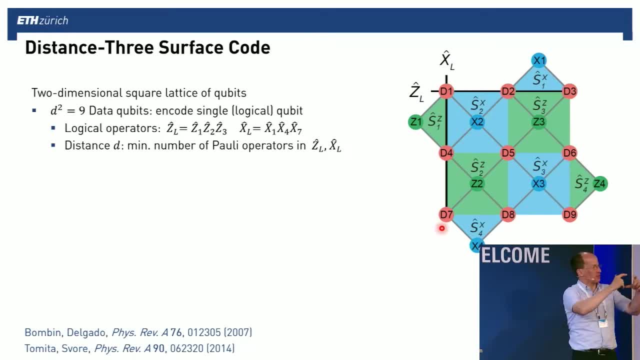 Now if I could write down the states for you, like as in the two-by-two example, but that will sort of quickly get difficult to look at. Then, if you are maybe a theorist and understand about commutators and so on, 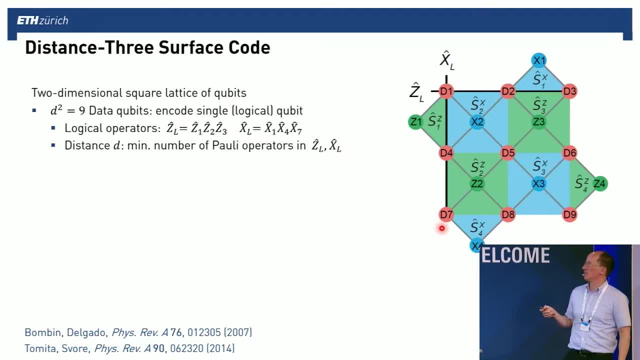 it is probably easier to understand it that way than looking exactly at the states and writing them down. In this case, there is eight of these auxiliary qubits. You can also figure out how many. They always need to be D squared, so the distance squared minus one auxiliary qubits. 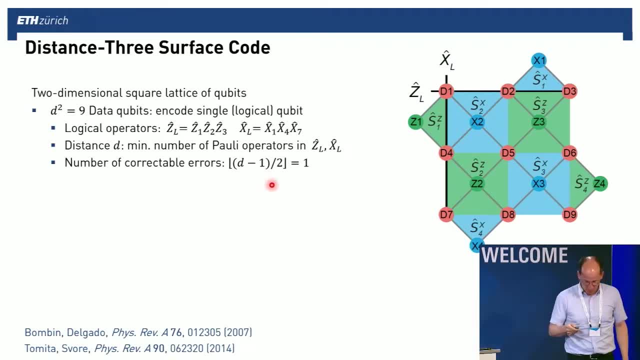 From the distance you can also check how many errors, how many simultaneous errors, you are able to correct. There is distance three surface code with nine data qubits. it is the smallest instance that can correct one error If you want to correct more simultaneous errors. 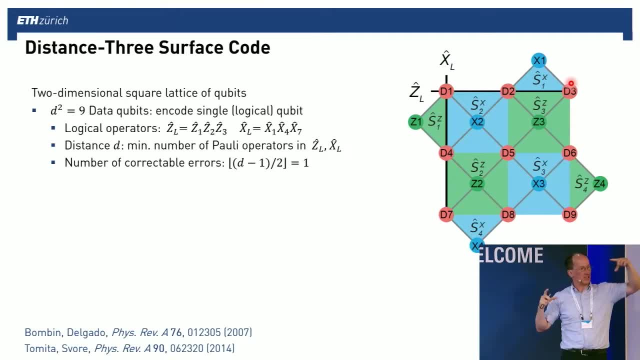 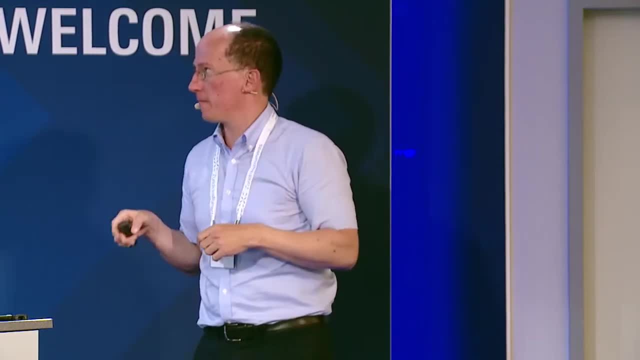 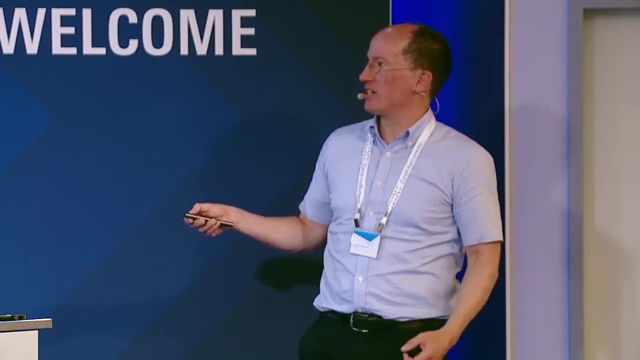 you need more qubits. For example, this distance, five, lattice. with 25 data qubits it can detect and correct for two simultaneous errors. always There is these auxiliary qubits. you do these parity or stabilizer measurements and there is kind of 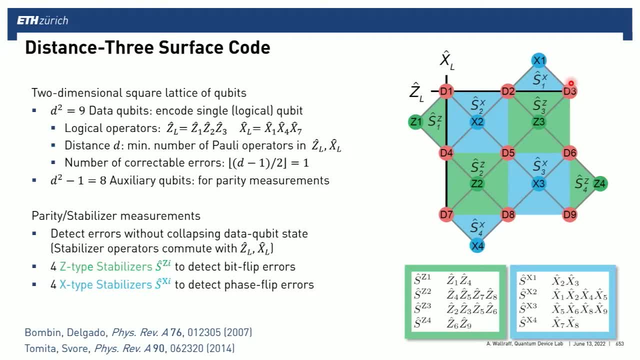 commutation properties and that you can look at and you can write down these, uh, these stabilizers, which are products of these pauli z and x operators here, and there's eight different of them, and sort of, in the center of the surface code there are weight four operators and there 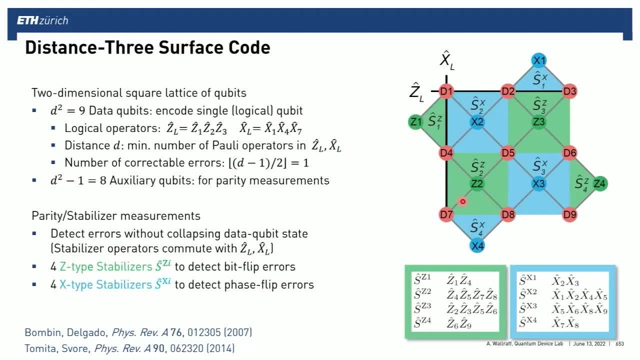 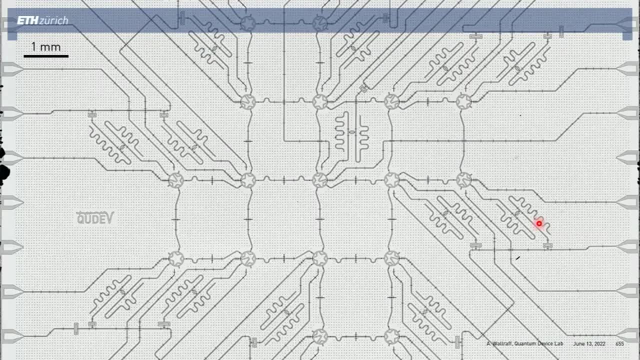 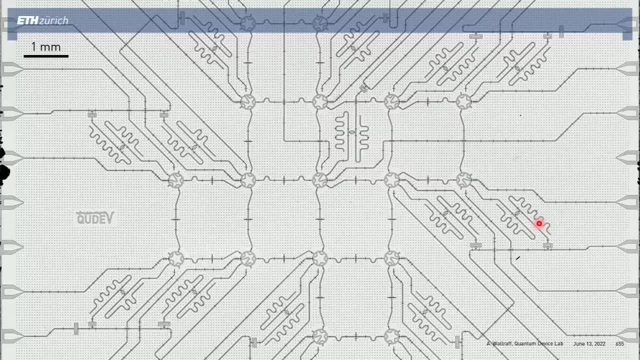 are some at the edge or so, yeah, where you see, like, like these qubits here, these auxiliary qubits here, they're only coupled to two neighboring data qubits, and so those are weight two, good, and then you try to build this thing in hardware. so so this is what a chip looks like and- and at this stage i i always say that you 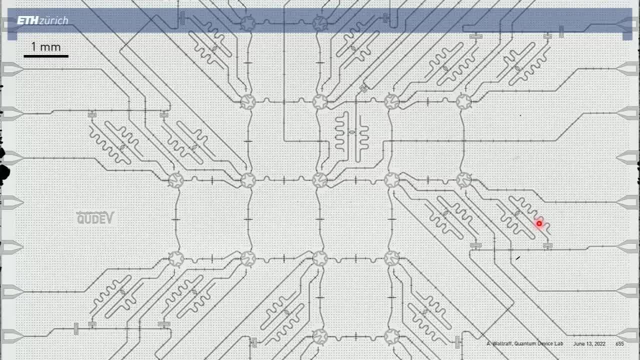 should feel privileged- privileged to be able to look at this, because i don't think there's any other lab that i've seen that would look. let you look at their 17 qubit chip or something. so i think your google's chip you've still not seen, and um, yeah, and so now here you can look at one. 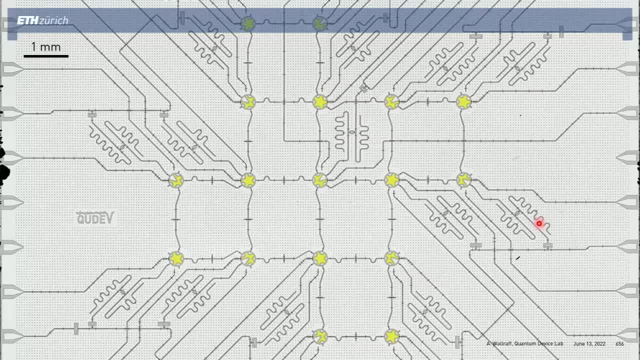 um. so the yellow structures are the superconducting qubits. they are laid out in the square lattice like the dots on my schematic um. so every qubit you can control with a, with a, with a microwave transmission line that is shown in in purple here, to which you 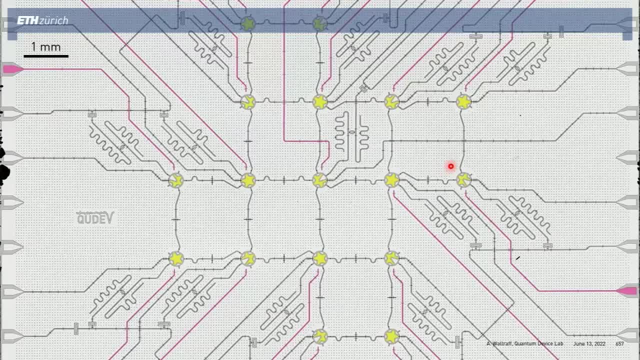 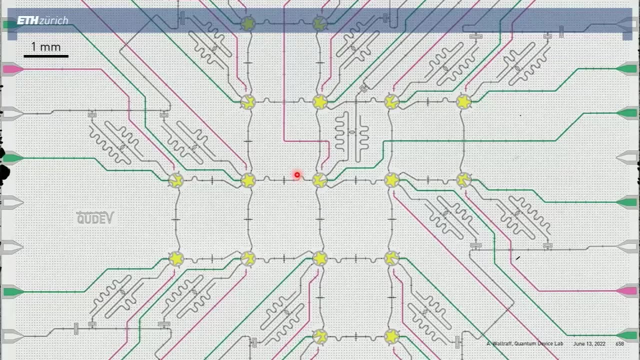 hook up a piece of instrumentation from your favorite manufacturer to apply short microwave pulses to it. then there is green lines here through which you apply short dc pulses that are needed for doing two qubit gates. these logical gates that i've mentioned, the. the two qubit, the c, not gates. 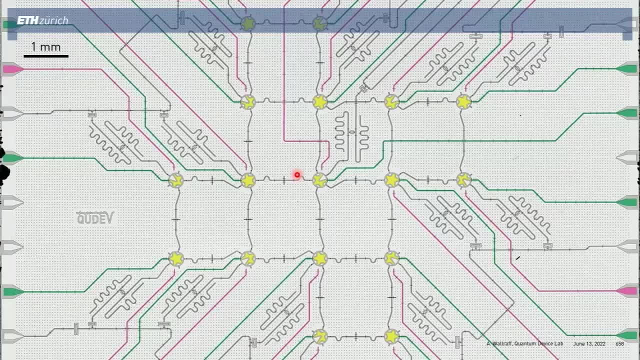 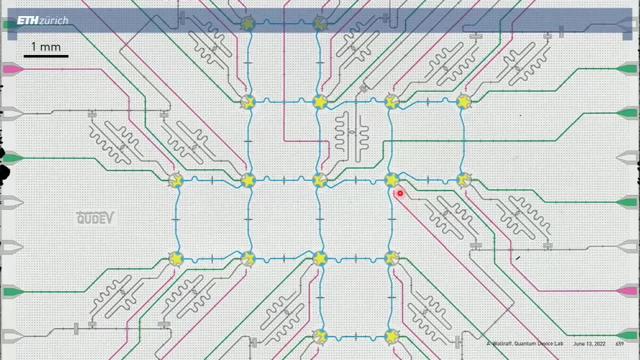 between the data qubits and the auxiliary qubits are realized by applying um, um, you know- voltage pulses to these green lines, here again from here, with the instrumentation from your favorite manufacturer. then there is a blue connections between the the yellow qubits and these blue connections. they 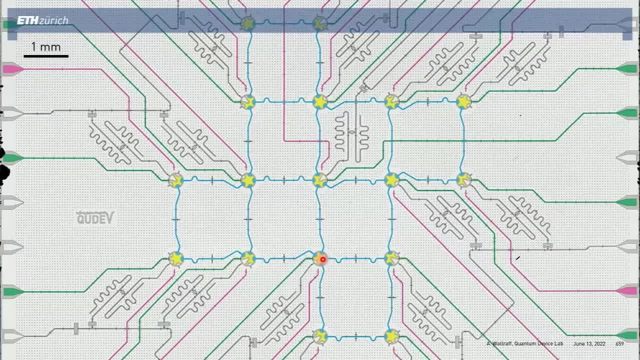 mediate interactions. so you can only do two qubit gates between pairs that are connected by these blue lines. all these lines that i've colored for you here are coplanar waveguide structures. on this device. everything is quite large, so you see a scale bar up here. 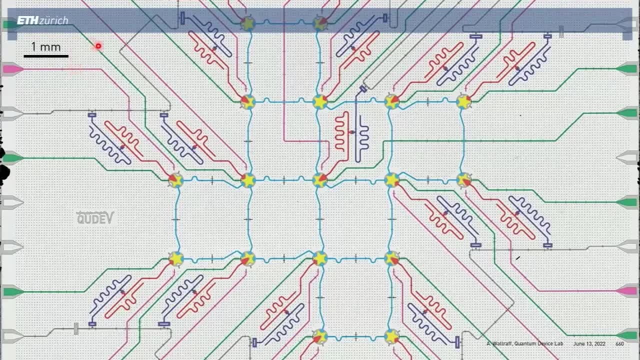 um, and maybe, then, one aspect that is very special about our chip, and which maybe helped us to do this experiment before ibm and google and anyone else, is that we had a very good readout for our super conducting qubits, and that gets done by hooking up a microwave frequency resonator to it with a. 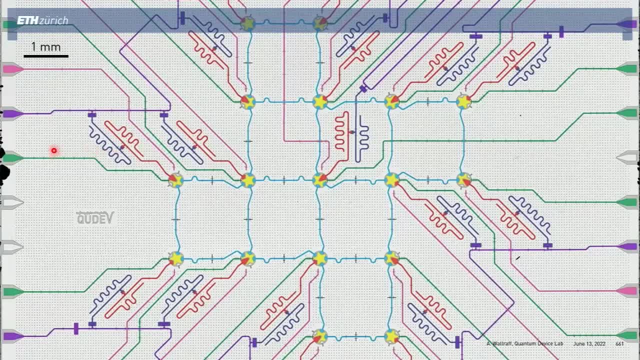 purcell filter and- and there are some frequency multiplexed feed line that is able to read out multiple qubits at the same time, and so, and in today's talk i've somehow chosen to rather explain to you the concept rather than how that works on the hardware level, on a chip. so if you had another hour, in the end i could. 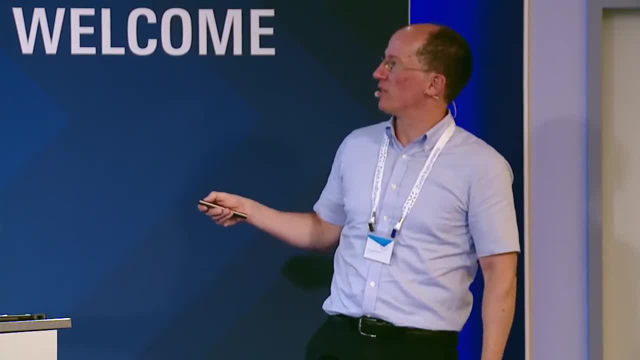 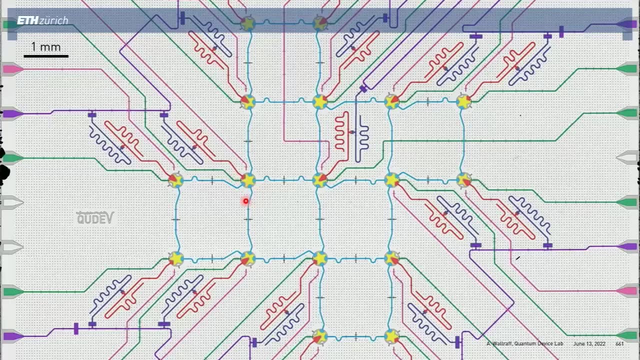 maybe give you some more ideas about that, but i rather thought i'd keep it with a, with a concept, and the reason why this worked for us first is is the fact that that this readout is really working very well and we've been developing that, uh, um, quite a bit in our lab since. 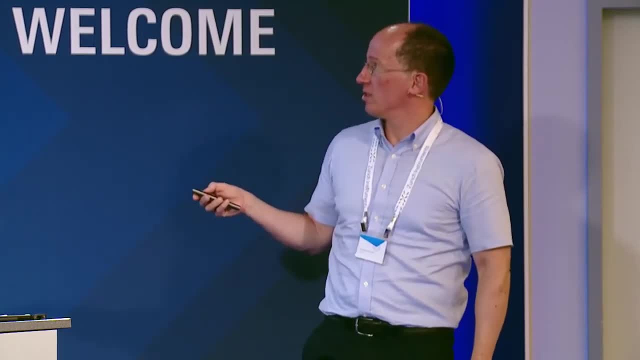 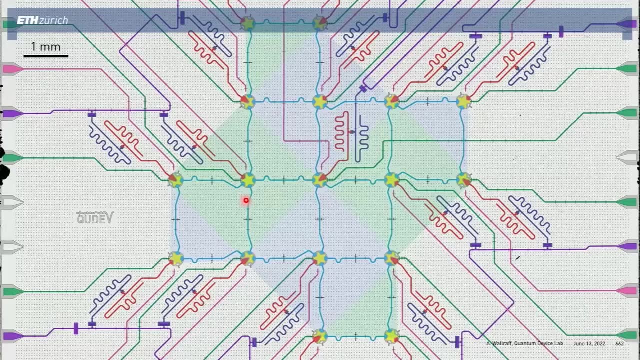 six years ago or so, and philip copious was involved in the first steps of that. okay, so here now. if you stare at this a little bit, you see that there's these placates and and the data qubits sit on the vertices of the plaquettes, and the stabilizer measurement qubits. 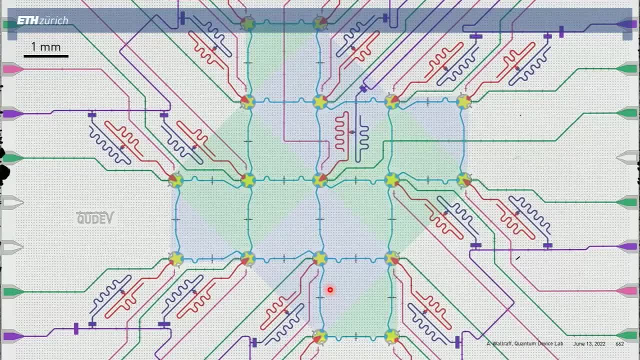 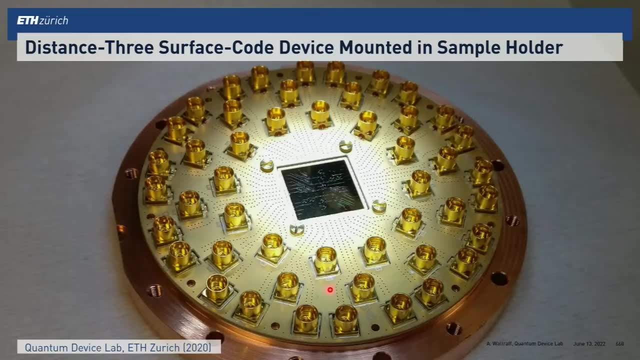 sit in the centers of these packets. and so now you associate this, this picture that you've seen before, with, uh, with the layout on the chip. all right, so? so then, uh, so here's the chip. so things are large, as i mentioned, so you see the, the structures on the chip, even under the microscope. here, 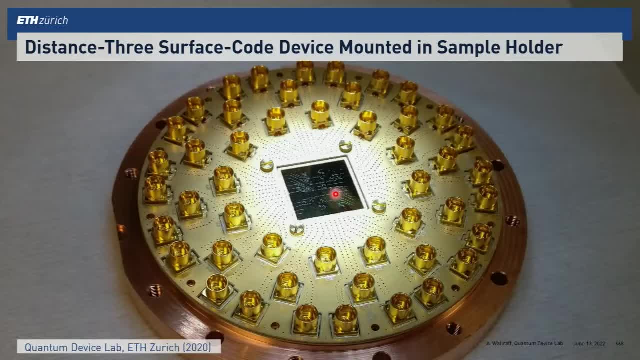 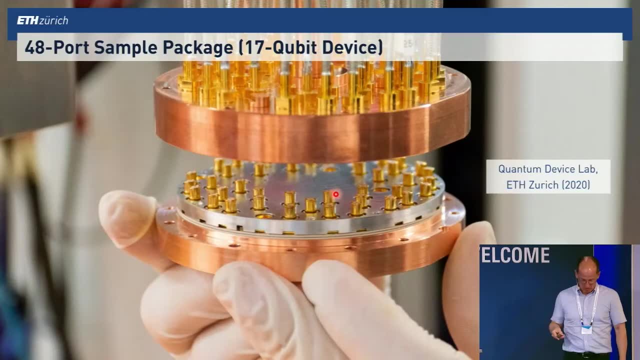 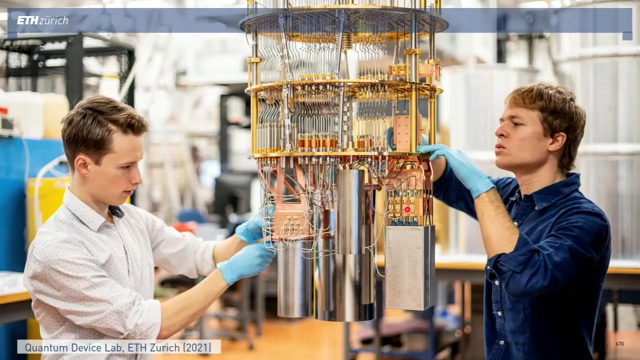 there is kind of a custom-made microwave frequency sample mount with 48 connectors on it. This you package in a microwave-tight and radiation-tight enclosure with some shielding. You put it into a big dilution refrigerator with even more shielding and magnetic shielding here. 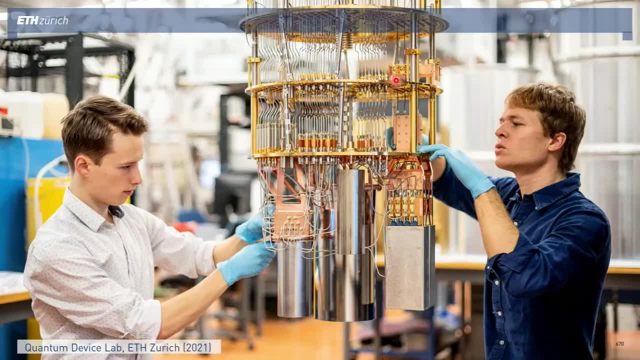 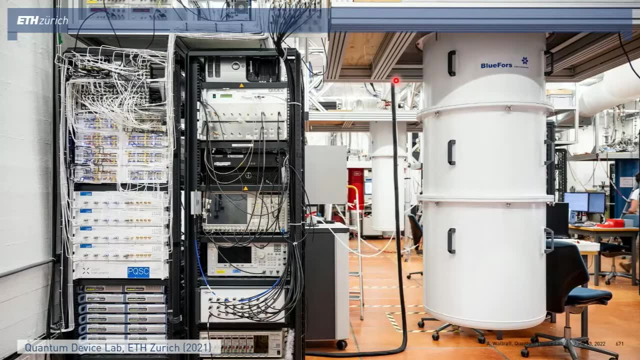 and all your microwave signal conditioning things circulate as amplifiers and so forth. Then you hook up your favorite electronics to it. This is one of the cryostats that we use, and here you see our favorite electronics currently also down there. 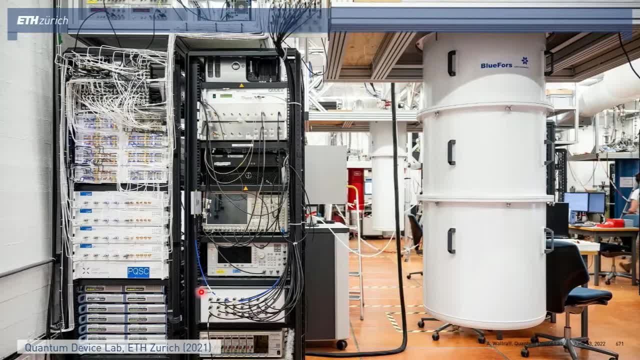 Also other electronics from the last generation that was much more bulky. so we tend to be using the type of stuff on the left-hand side and you see that it starts to get sort of a bit messy. So this is all the electronics that you need. 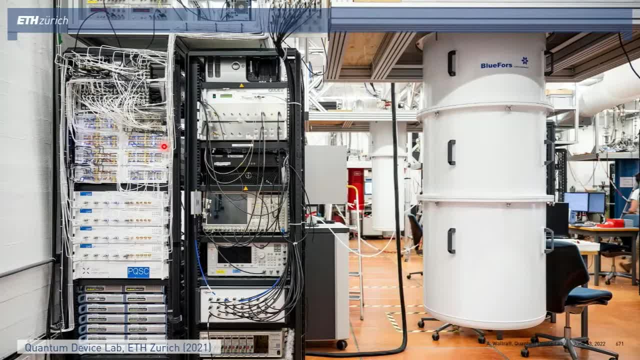 for 17 qubits for one logical qubit, and so maybe there you also see that okay, if you want a million logical qubits, you probably will not multiply that by 10 to the sixth, and so it is more work to do. 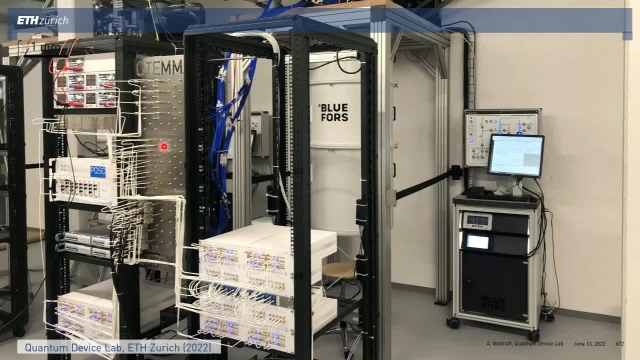 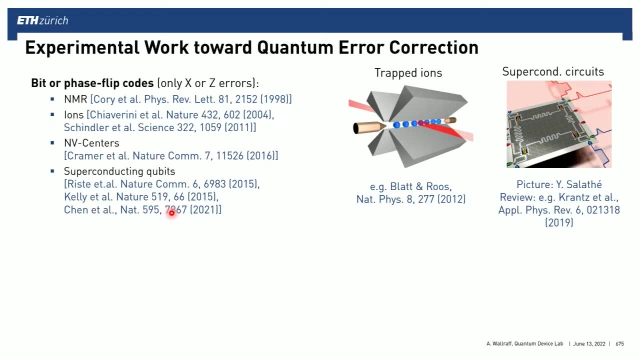 So this is a bit more cleaned-up setup at our new lab at PSI, with kind of more modern versions of the same electronics from your favorite manufacturer. Then you try to make that work, and it is actually quite hard to make it work well, and of course, nothing in science. 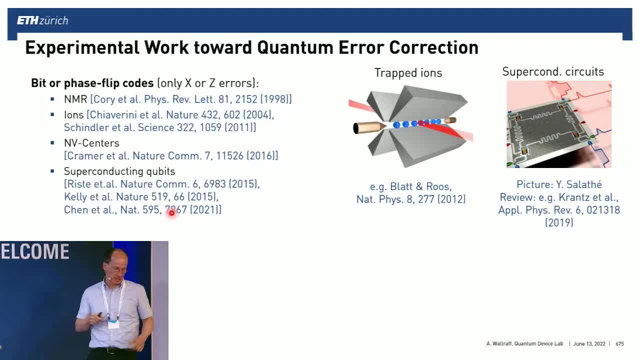 nothing ever stands on its own. so there was lots of previous work on this and the different steps. So there were different steps for first correcting only these X or Z arrows, so bit flips or phase flips simultaneously, or only that arrow but not the other one. 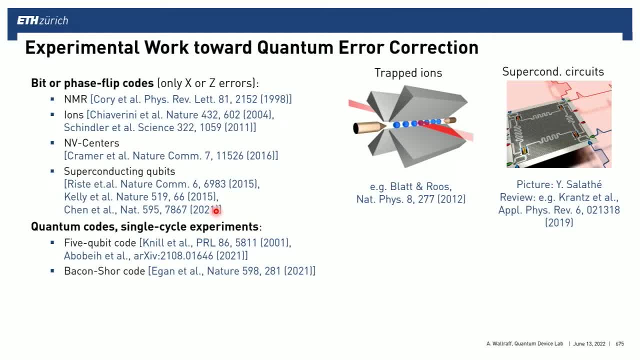 Then there were experiments in which both arrows were corrected, but only once. but in a quantum arrow-corrected system you need to correct it. correct it continuously, so you need to check for errors always. Then there was a repeated error detection experiment. 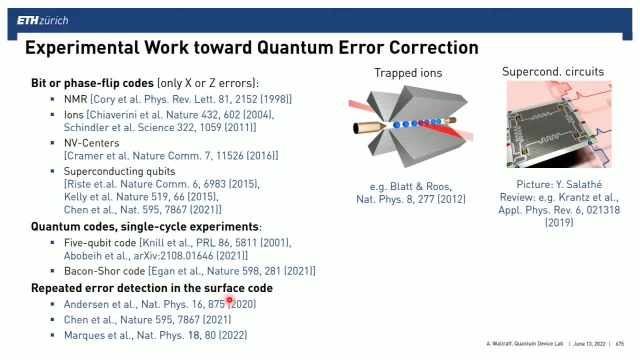 also one from our lab in which the device was large enough to notice whether errors had occurred, but you could not tell where. This thing tells you, oh, the parity has changed. but you need to look at these parity measurements and tell: okay, which one of the 49 qubits 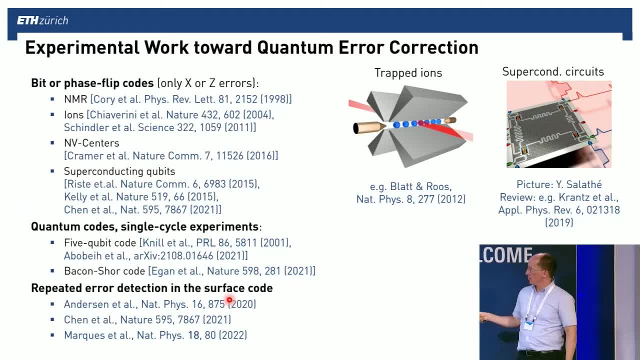 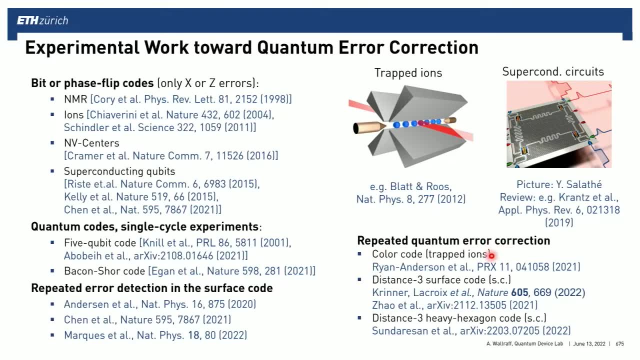 actually had the error on it and you need to decode that. Then at the end of last year or in the middle of last year, there was actually an IonTrap experiment by Honeywell, and then there was our experiment, an experiment from Zhenyuan Pan's group in China. 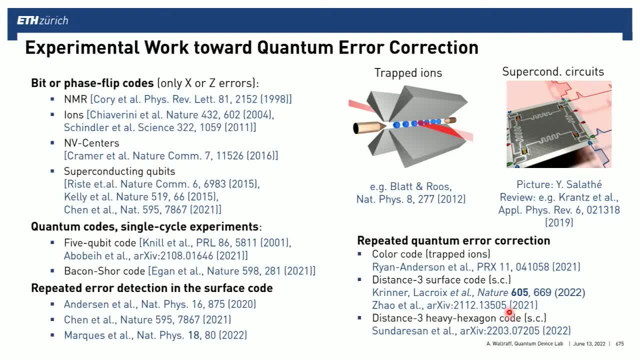 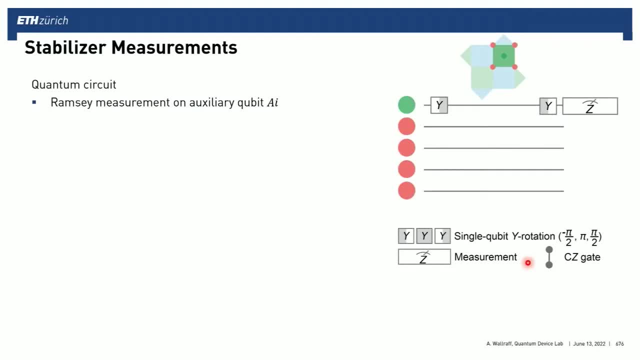 and then also an IBM experiment in March this year that realized a so-called distance three quantum error correction code in a logical qubit. Good, The key element is this: parity measurement. I will say a few words about this parity measurement and then with that we can then get to the final results of it. 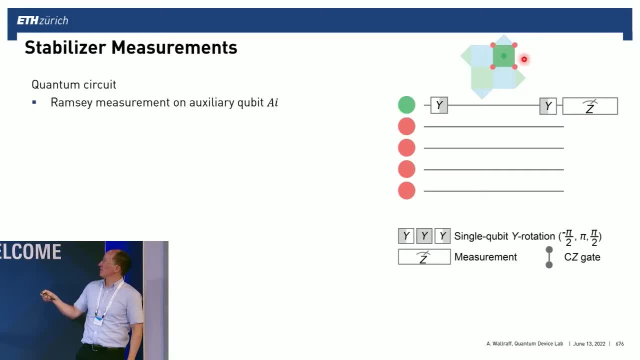 This parity measurement I mentioned. you have these plaquettes here. There is four data qubits, the red dots with an auxiliary qubit in the center, and you run this gate sequence where you run two qubit gates between the data qubits and the auxiliary qubit. 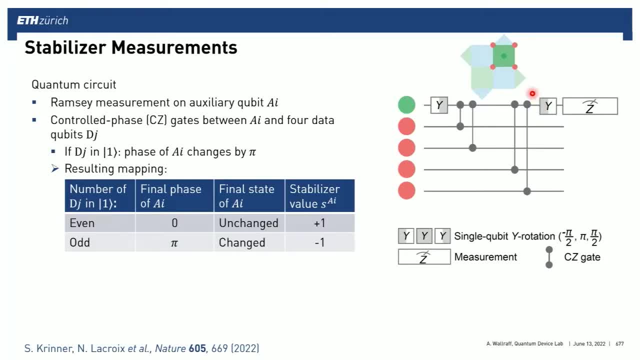 This is in our actual hardware. it is implemented a little bit differently because our actual hardware it does not implement CNOT gates but C-phase gates. but okay, you can ignore that for the moment. The symbol here is a little bit different. 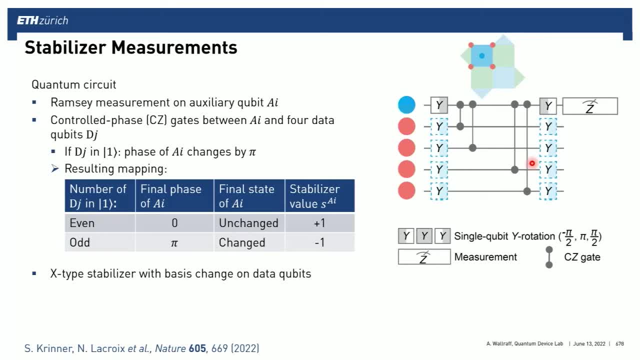 but it is essentially equivalent. You can do the same thing not only for the Z arrows, so in the green plaquettes, but also for the X arrows in the blue plaquettes, by doing this basis change that I had mentioned to you. 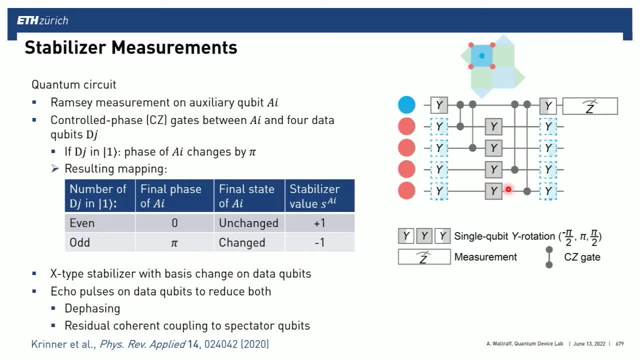 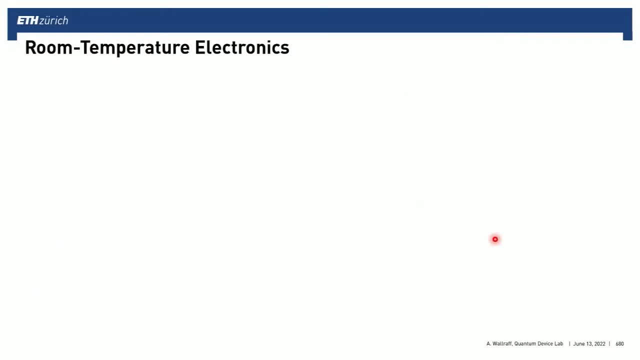 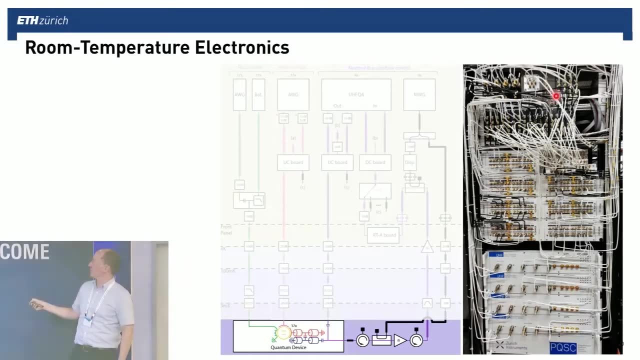 Then there is a trick that helped us is you do some echo pulses in the middle of the sequence. that helps us to improve the quality of our gates. Okay, so now there is my one electronic slide. There is another zoom in of the stack of electronics here. 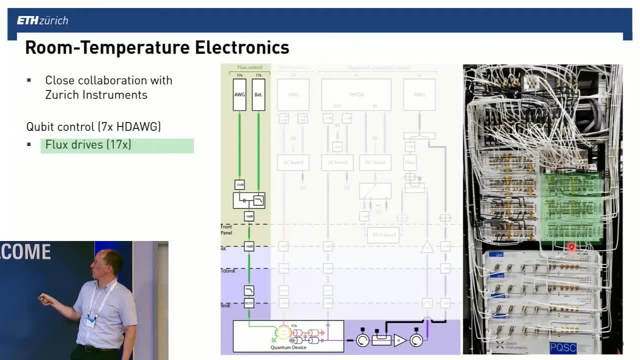 That has these has HDAWGs which we use to tune the transition frequencies. so that applies voltage pulses to our qubits to tune the transition frequencies and what we do for doing two qubit gates: we tune neighboring qubits into resonance with each other. 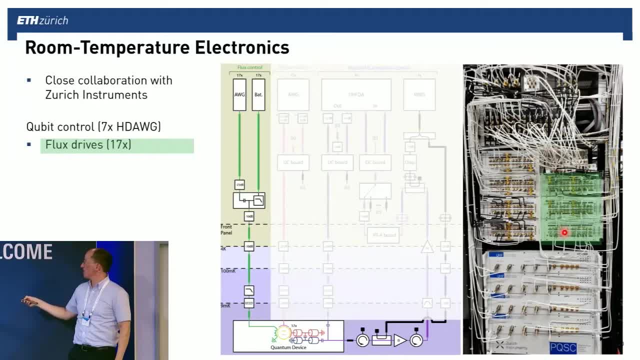 and then detune them again, and that gets done with these boxes here. Then there is another set of these boxes, which are fat, the signals of which are fat, into a mixer that has microwave sources connected to it, which were made in this house, I think. 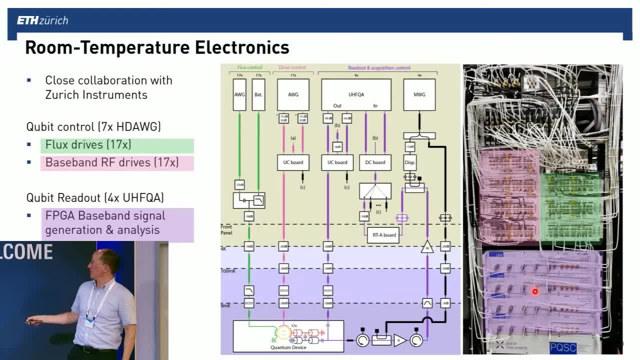 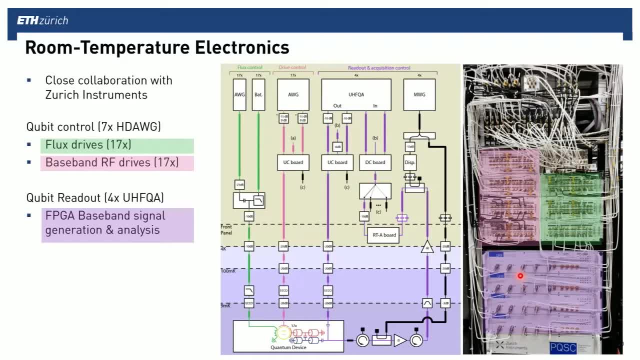 and then there is boxes with FPGAs in them, and then there is boxes with FPGAs in them that detect the measurement signals, that read out our stabilizers on this, which help us to identify where the errors have occurred. Then there is up and down conversion electronics. 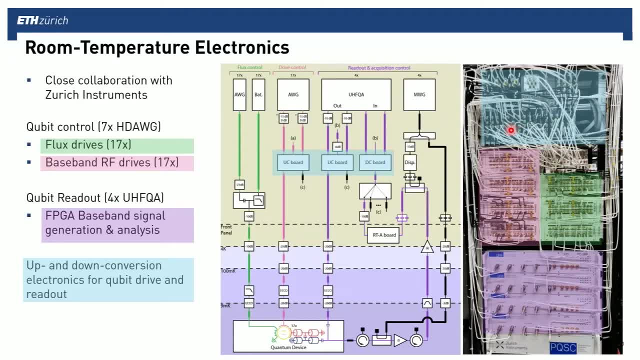 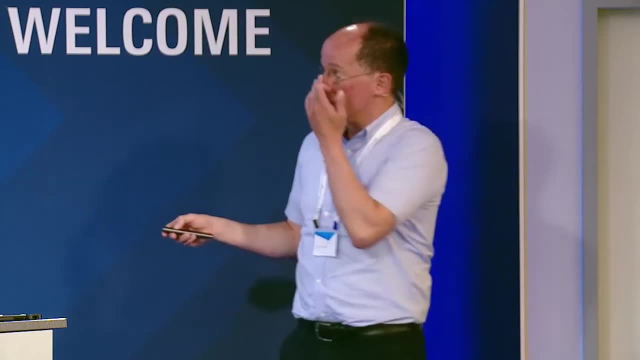 that here were still in a demo version that was assembled in our lab but where you can also now have a box from this manufacturer if you like. Then there is some synchronization between these boxes. with this yellow box at the bottom, You make this all work and it takes a while. 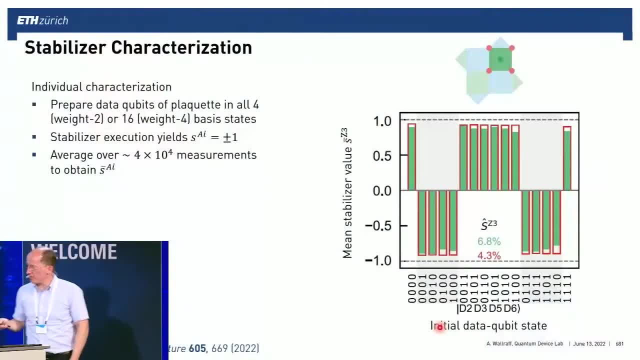 and then you see whether your stabilizer measurements do work and sort of the basic thing that you are trying to do is. so I claim to you that this measurement, this gate sequence, it can distinguish whether there is an even number of zeros and ones in your state or not. 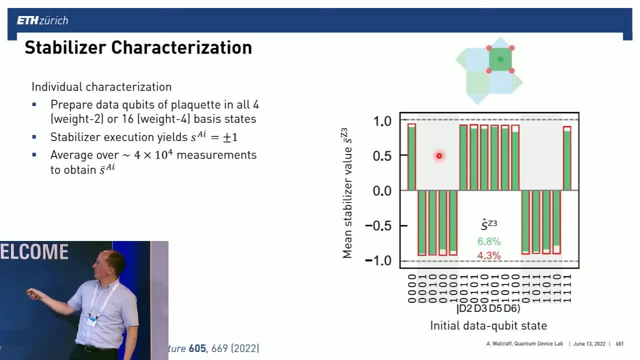 That should be. when there is an even number of ones, then your stabilizer or your parity measurement should indicate a one, and when the number is odd it should indicate a minus one. and so now you can go through this list at the bottom here. 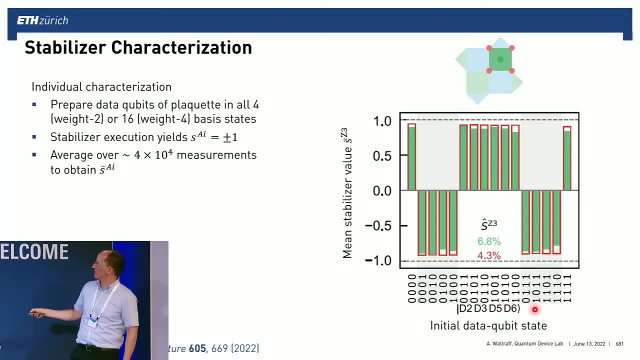 and check whether there is sort of a one. every time there is an even number of ones and a minus one when that number is odd. and you look at this and you see it works, and this quotes the error, and the error is not tiny. 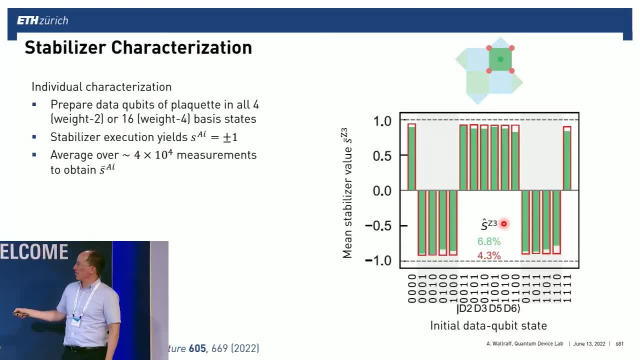 Yeah, it is kind of. I mean it is sizable. The error on it is a few percent. so one thing that I also did not say is, like every two-qubit error on this device is roughly a percent. so you do four two-qubit gates. 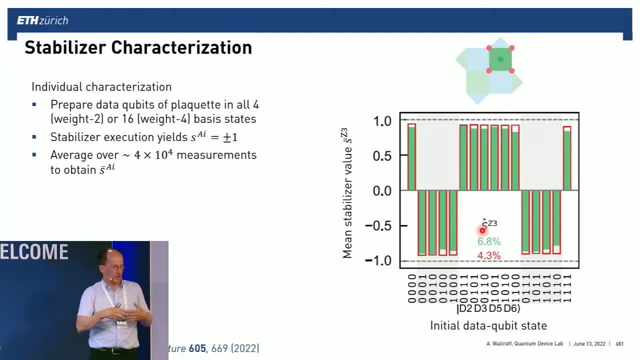 in a sequence and the single qubits have also a little bit of error, and there is a little bit of measurement error and so that accumulates. so you will have a little bit of error in this parity measurement, but the surface code told you that some error is okay. 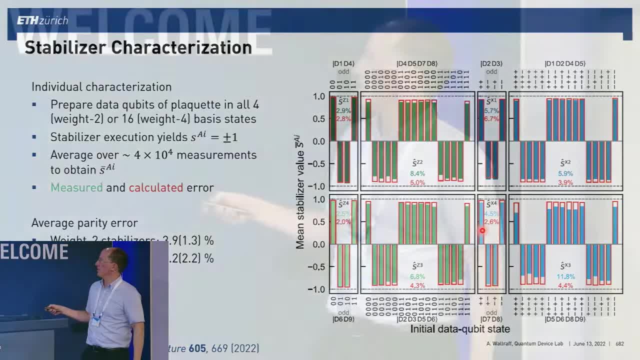 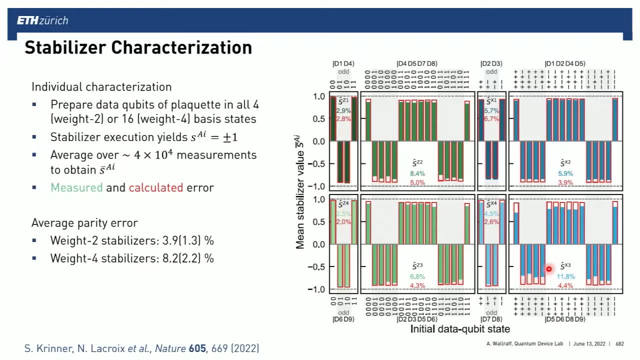 It can recover from some error, as long as that is not large enough. and since there is now not one stabilizer but eight, we did go through all these measurements and then you could sort of stare at it for a while and verify that it is always one when the parity is even. 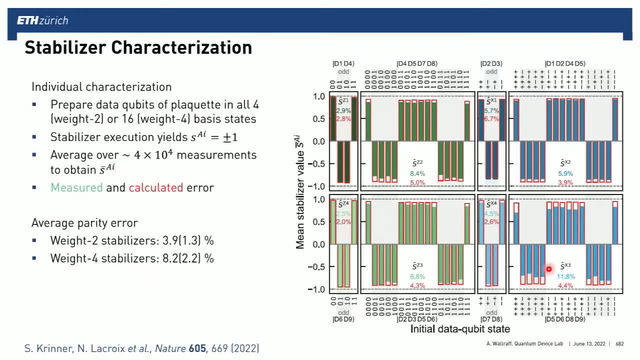 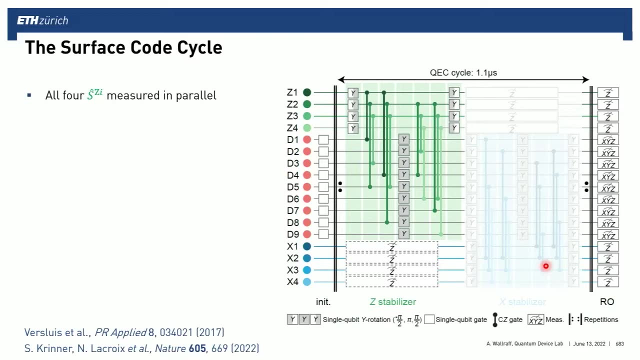 and minus one, when the parity is odd and we can also roughly understand how good it is, which is the comparison to the red outlines Good, so that is probably roughly at the stage where one loses the audience because it gets subsequently more and more complicated. 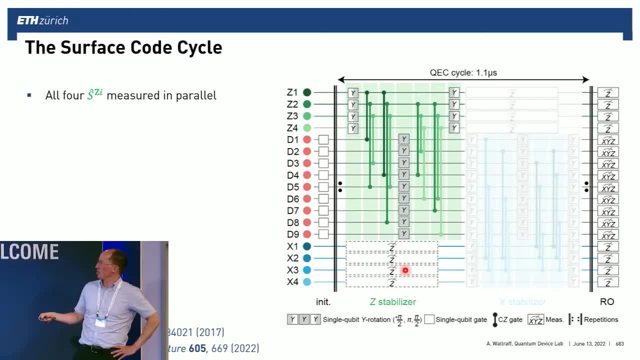 so here is the gate sequence that you execute on this distance: three surface code for one error correction cycle. so you have to do all this stuff to correct errors for one cycle and any quantum computer that is error corrected will have to do something like that. 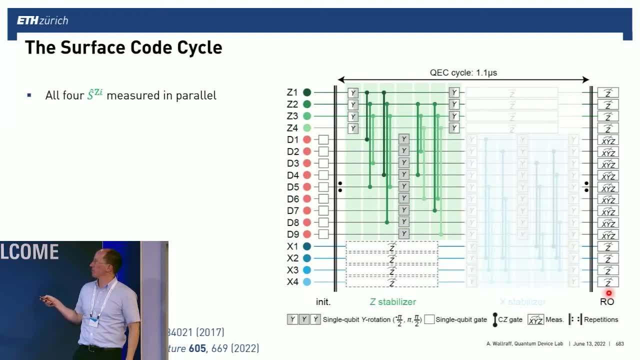 every sort of effective clock cycle or error correction cycle. so there were two types of parities that you measure, in the Z basis and in the X basis, and we do all the gates for the Z basis parity measurements first and then we do all the gates for the X basis parity measurements. 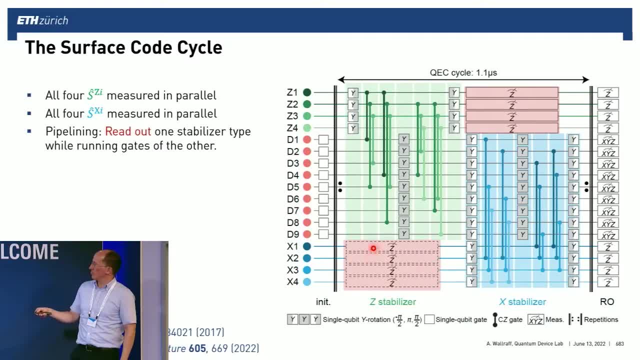 second, And maybe the special thing in our setup, and the one that sets us apart from IBM and Google and others, was that these readouts are very fast, so the length of the readout is less than the accumulated length of the gates for doing the stabilizers. 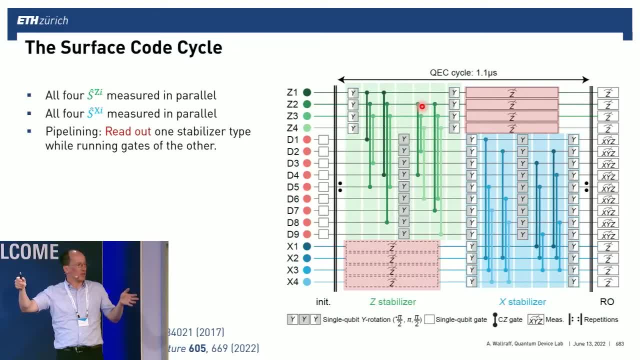 and at IBM, for example, this readout is maybe five times longer. and then, even if you have better coherence qubits, it does not help because your whole thing will last too long. so you need to realize good readout on your auxiliary qubits. 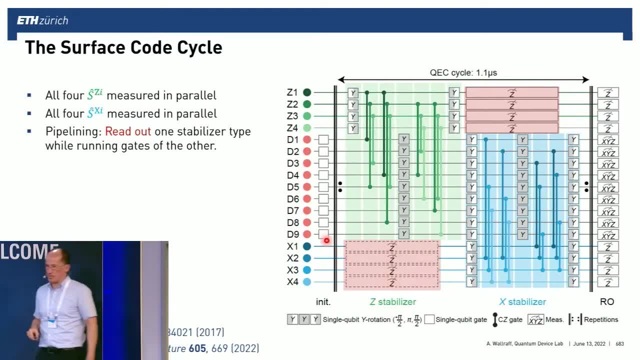 because that is what you look at- to verify whether you had even or odd parity in your devices. Good, and then you program all the software on your electronics to apply this pulse sequence and see whether that works. You run it to prepare this logical zero. 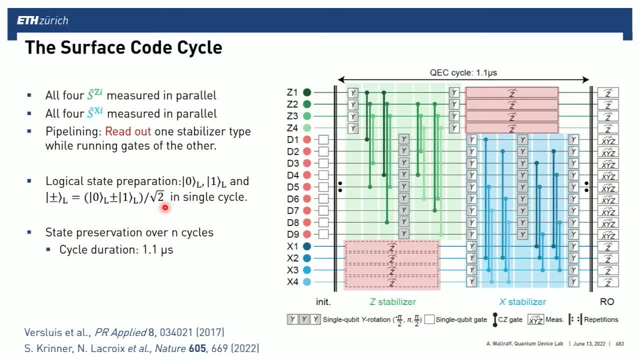 logical one, and the superposition states which I have mentioned, and this whole cycle for us now takes about a microsecond. and, okay, there is some detail about leakage, which I think I will. So it is very, very important, but I will not bother you with. 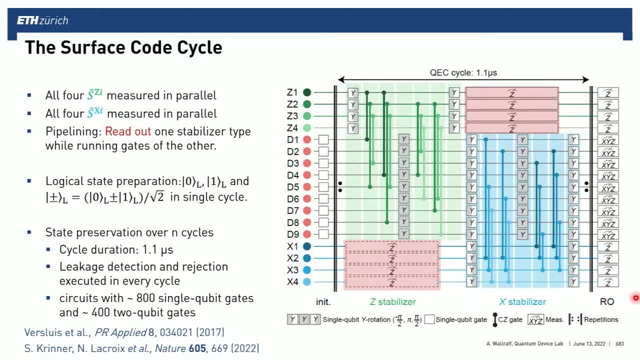 And what is maybe also interesting to say: if you now count number of gates- so we have executed the cycle for up to 16 times- then you see that there is about 800 single qubit gates and about 400 two qubit gates. 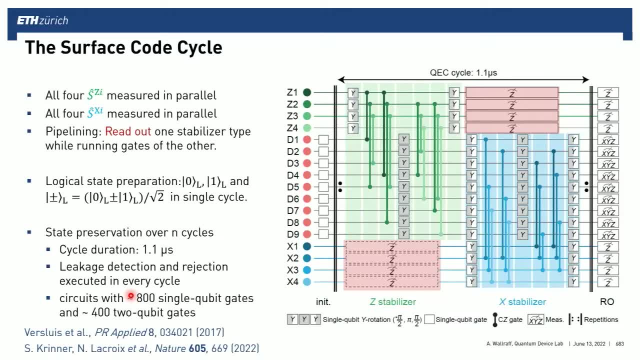 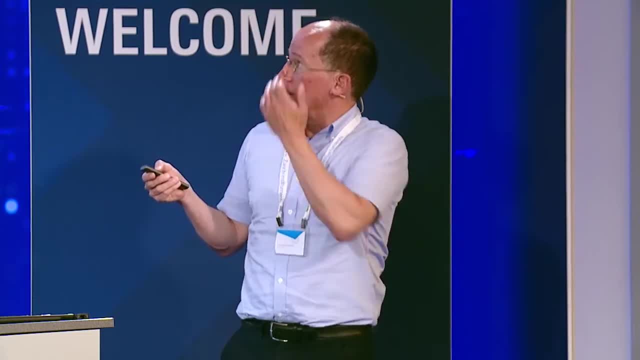 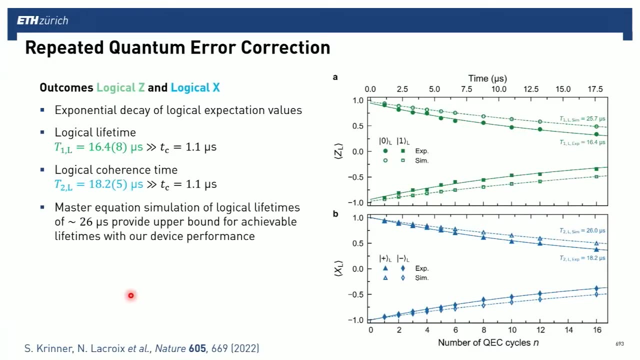 So complexity-wise, it starts to be on the same scale as this quantum advantage or quantum supremacy experiment that Google did a while back. Okay, so maybe to leave some time for the questions, I would likely skip this slide and not explain the details. 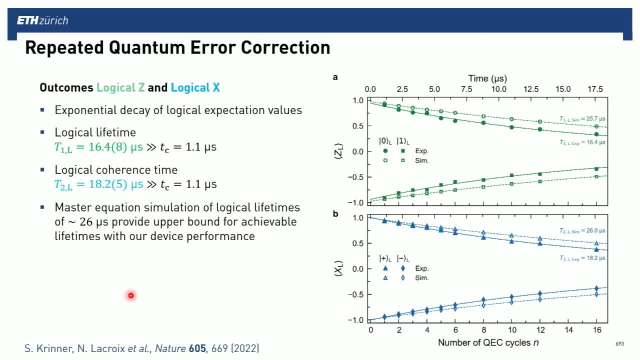 So this is essentially about now. you compare how your single qubit would decay from the excited to the ground state. and now you do this complicated thing with all the encoding and the error correction and you now look at how your logical qubit decays from the 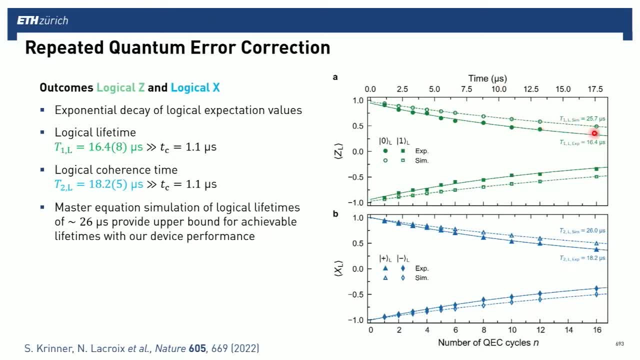 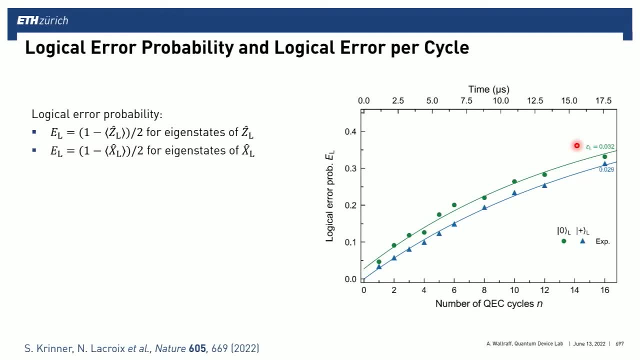 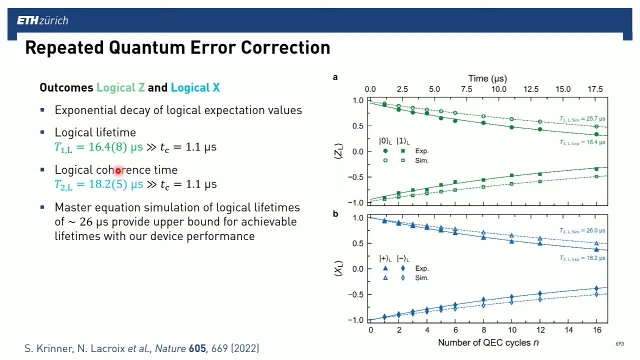 excited state to the ground state and you can extract that decay time if you want. Okay, maybe one thing I should still say, and the decay time. so one of the aspects that matters is how does this decay time that you extract from these curves here, which? 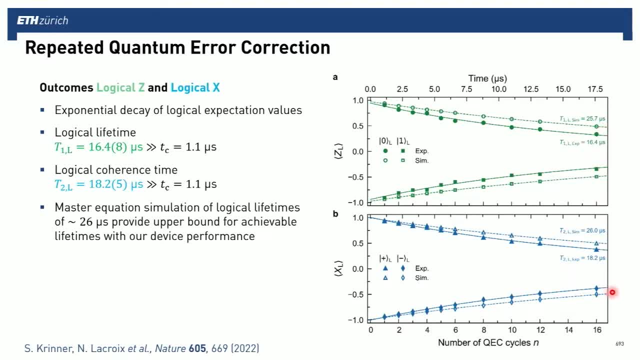 is like this energy relaxation time and the dephasing time that I mentioned in the beginning. how does that compare to the cycle time? the time that you need to run one error correction cycle And the relationship between these two numbers will tell you how much error you make during. 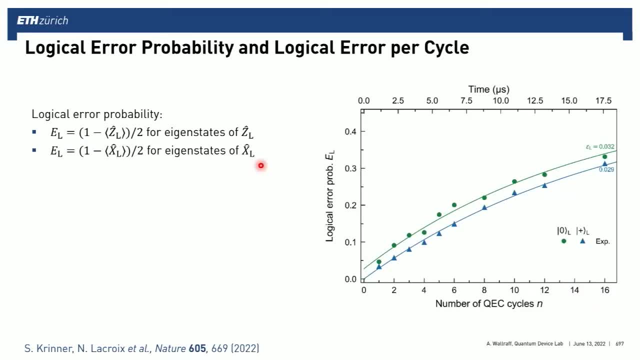 one cycle. And that is what is on the next slide, which I will maybe then explain. Okay, I will explain a bit better. So from the curves on the previous slide you can correct how the error accumulates in your logical qubit, both in the Z basis and in the X basis. and so here is how the 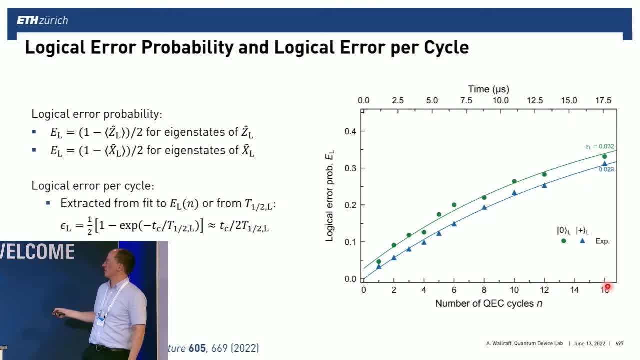 logical error accumulates. So once you continue running your error correction cycle, your accumulated error gets worse and worse, which is not surprising. Things decay with time, even when you are trying to correct errors. But from these curves you can now extract how much error there is. 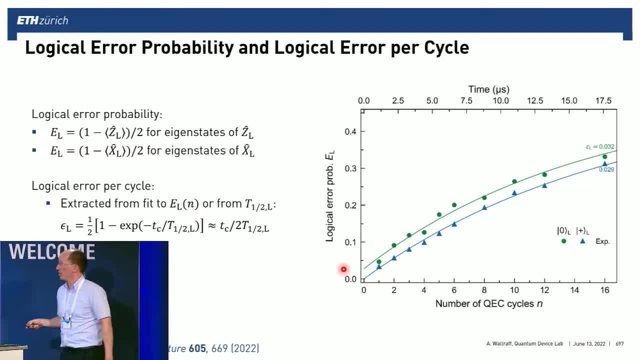 Per cycle, per one round of error correction, And in our case this is about 3%, And this is kind of interesting to notice. So this is built up from 24, two qubit gates which have 1.5% error each and which accumulates. 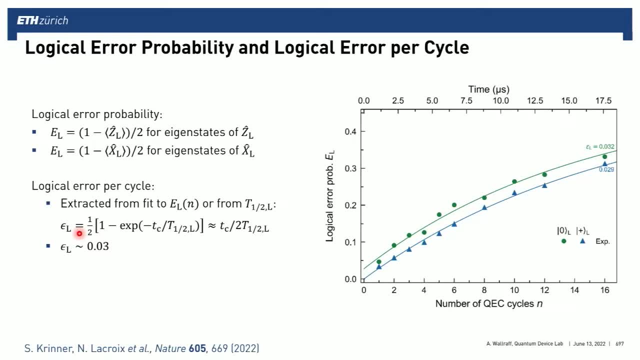 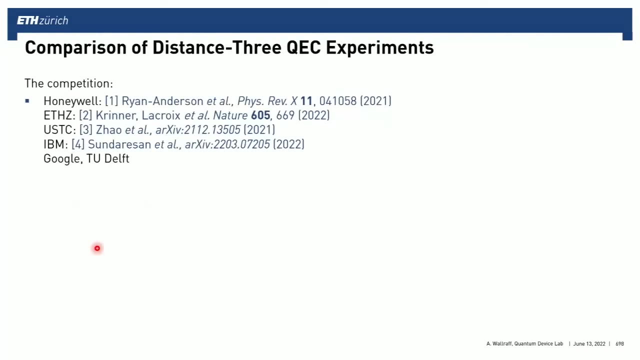 But with evaluating your errors from the measurements that you do on using these auxiliary qubits, you can correct for these errors And you can also get the logical error array to be only on the order of 3%, And so now you could. so first maybe you could ask yourself: how good is that in comparison? 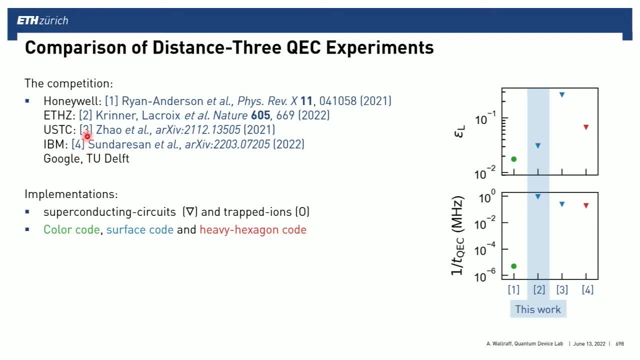 to other distance, three surface codes And, as mentioned just after us, Jean-Y Pan's group put a paper on the archive that discussed their results. There's this work by Honeywell and there's now work by IBM since March. And so here's this: error per cycle. 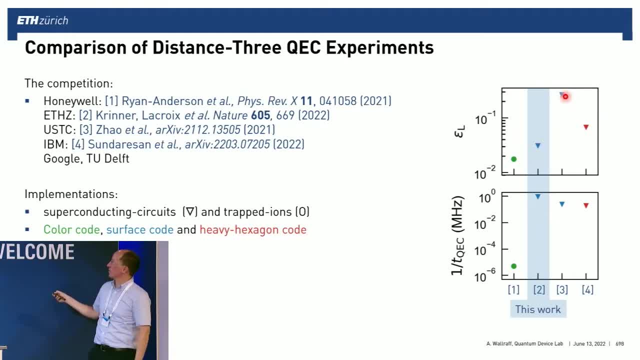 And so Our experiment has a lower error per cycle than both the other superconducting qubit experiments. It has a little bit higher error per cycle than a Honeywell experiment, But then you look at the ions and at some stage wall time will also matter. 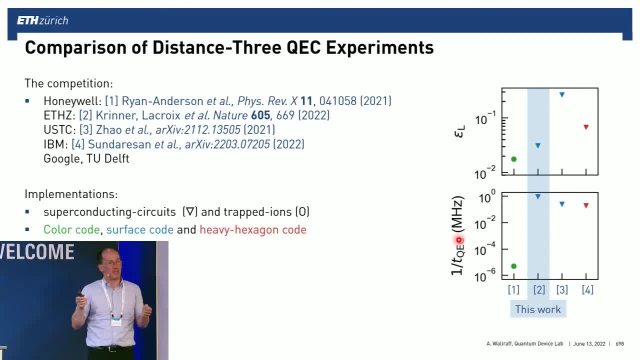 And the ion experiment is very, very slow, And the main reason for that is that you need to do individual measurements on the ions which store the error information, And then You have to sort of move the ions physically around somewhere else, so that while you do, 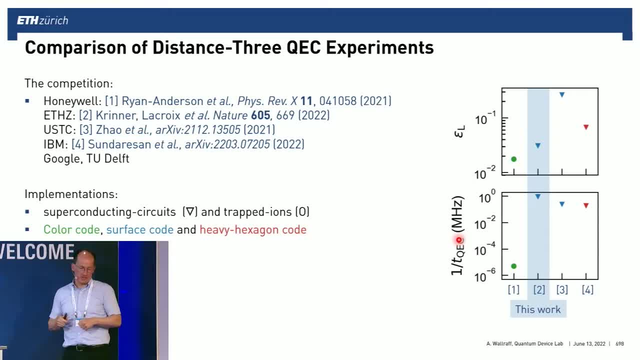 the measurement, it doesn't destroy the information stored in the data qubits And that makes their experiment essentially five orders of magnitude slower. And so maybe, like, as long as you talk about normalized quantities, maybe you don't care so much, But once you once wall time will matter, or so, and like whether you have a factor of 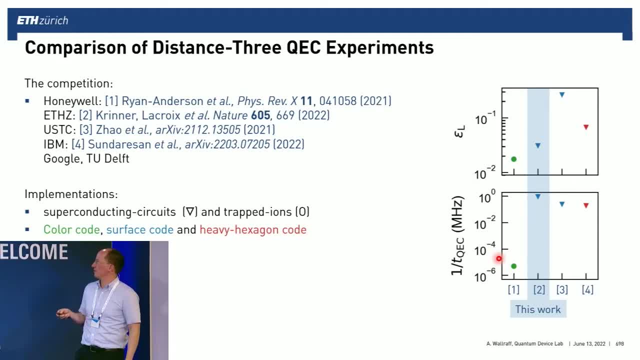 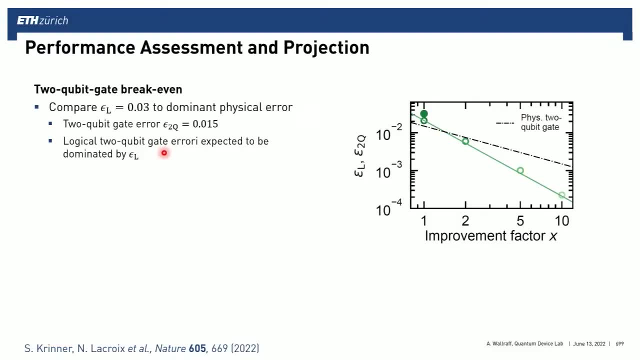 10 to the five in front of some duration for your algorithm will likely matter. So And so then, finally, how good is 0.03 error per cycle? That's clearly way worse than you would need for a real processor, And so what we chose to compare it to is to compare it to an error rate. that would be. 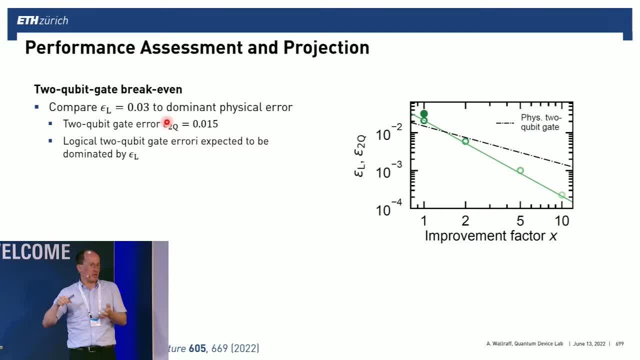 relevant when you're trying to do gates between two logical qubits. So the next step would be you take two of these things times 17 qubits- or maybe a few more because there is a little bit of overhead- and you would run logical gates between two logical qubits. 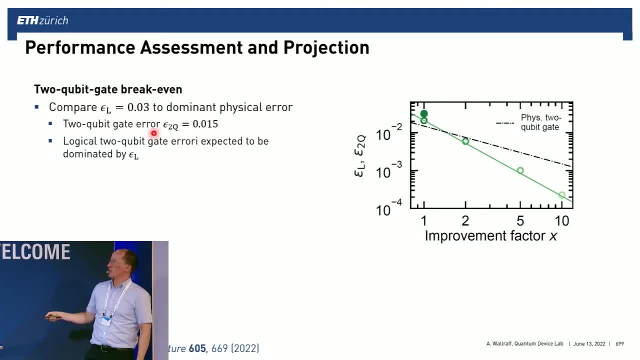 Maybe in the simplest to consider case there, what would matter? if you can do transverse logical two qubit gates- which I do not expect you to understand what that means immediately, but maybe some of you do- If you could do transverse gates. 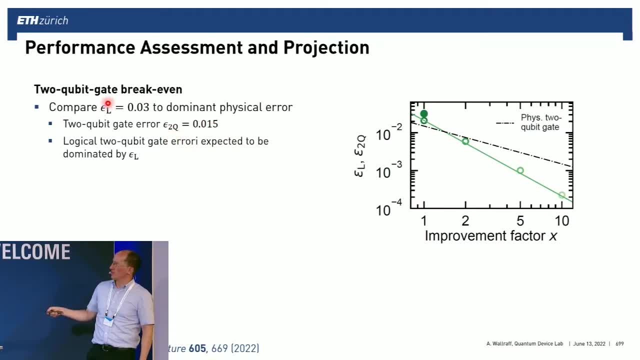 what matters is the physical two qubit gate error. We see that the logical error per cycle is about twice the physical two qubit gate error. This you can actually use to and no worries. I am sort of finished now so that there is some time to take questions. 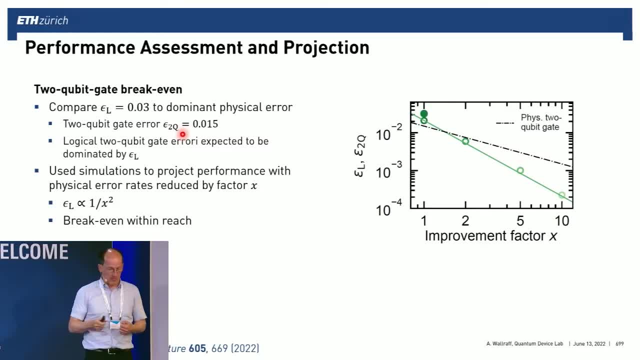 You could use that to ask yourself like: how close are you to some form of break even? In the end, what you want is you want your logical qubit to be better than your physical qubit. There is various senses in which you could discuss that. 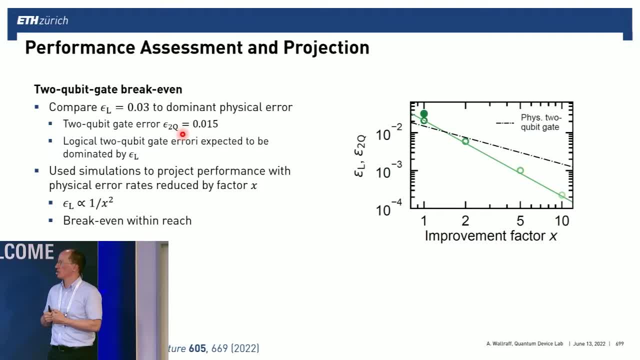 either as a memory qubit or when you want to do gates between two logical qubits. In the end, I think our experiment is pretty close to this break even, but it is not really better than this break even. You could now say, oh, this is disappointing. 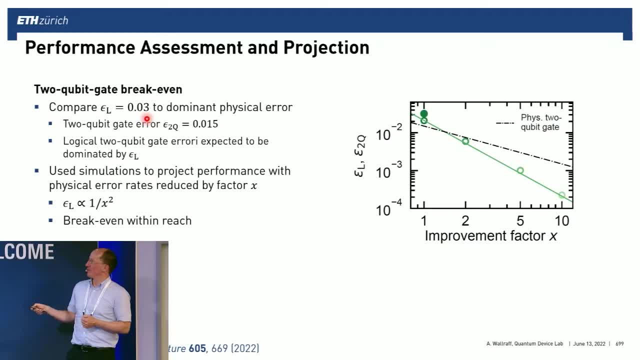 so why did you do that? A colleague of mine on Twitter said: oh, you made a logical qubit and it is worse than your physical qubit. Okay, good, We think it was hard enough. We worked at it six years. 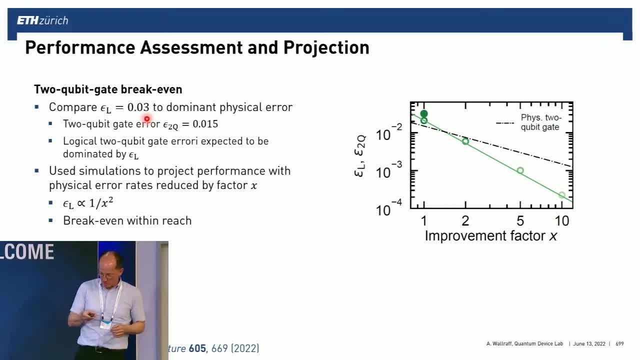 We were pretty happy that it worked at all. I think IBM and Google would also have been happy if they had done it. So this is close to the threshold. What is important maybe that it is not very far yet. It is not a factor of 100 away where you would think. 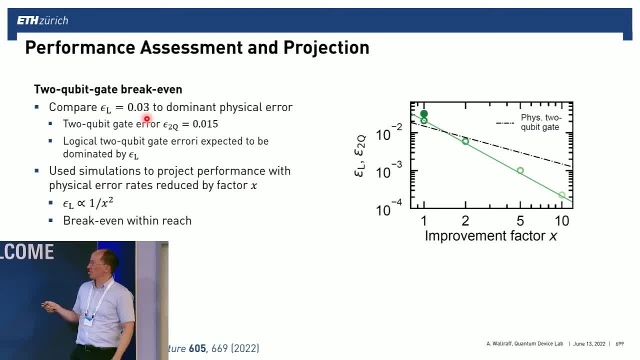 you would now need another six years to get it across this threshold. We are thinking we are pretty close. Also, the threshold is something variable. In the end, you want to be much, much better than the threshold, not just close to the threshold. 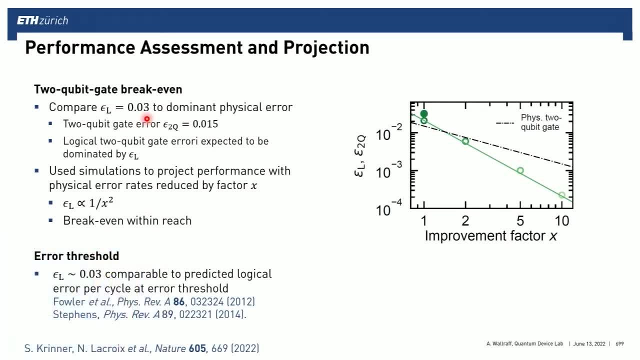 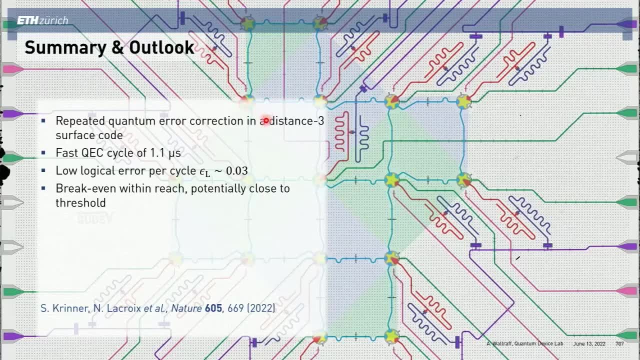 so there is even more work for everyone. There is more analysis that you can do to verify that. So, to sum it up, we have done this distance three surface code. I hope I told you a little bit about what that is and how it works. 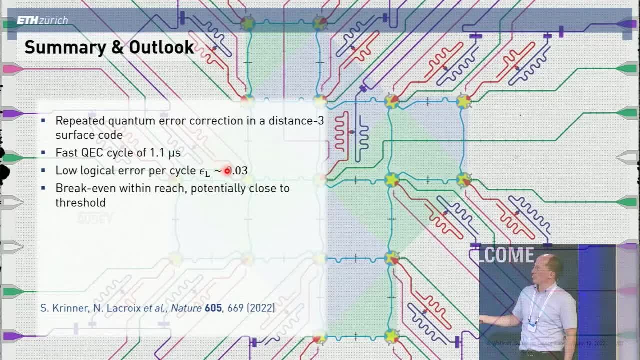 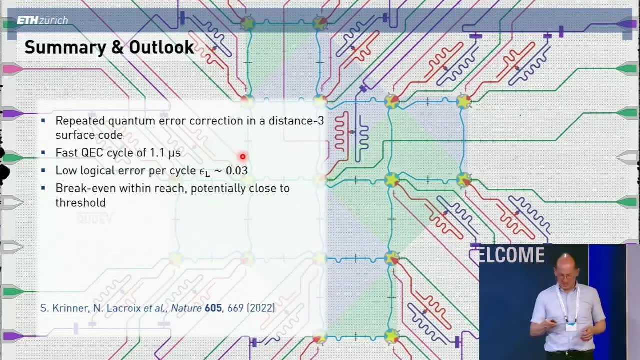 It has a fast quantum error correction cycle. It has a small logical error rate. If you are in the first year of doing this then it is always kind of small because there are no other logical error rates for distance three code from anyone else at that stage. 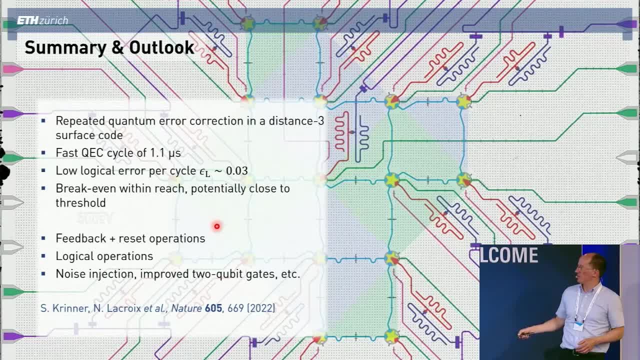 This break even is within reach. The next thing that we want to do is, if we have electronics, we want to do this first generalization with low latency, or so we can do feedback and resets, for example, and then we would look into doing logical gates. 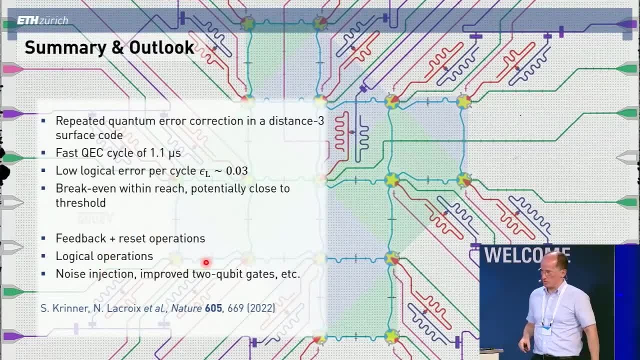 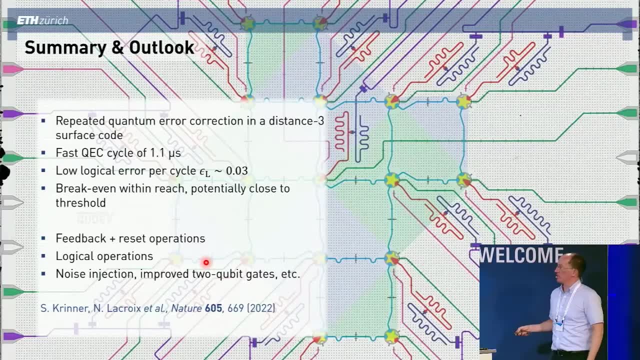 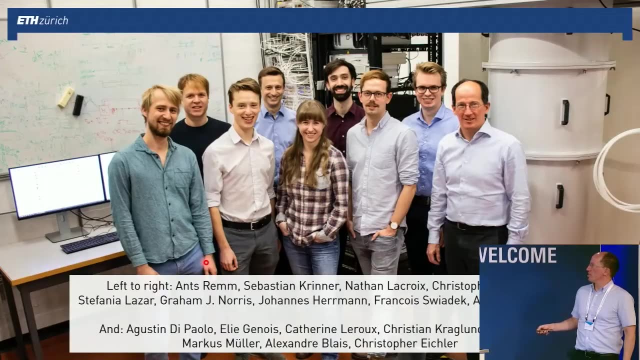 between logical qubits and maybe seeing how resilient these logical qubits are to injecting noise into our devices, to see how they respond to artificially increasing the background noise level. I should mention once more, so this is a picture of the experimental part of the team. 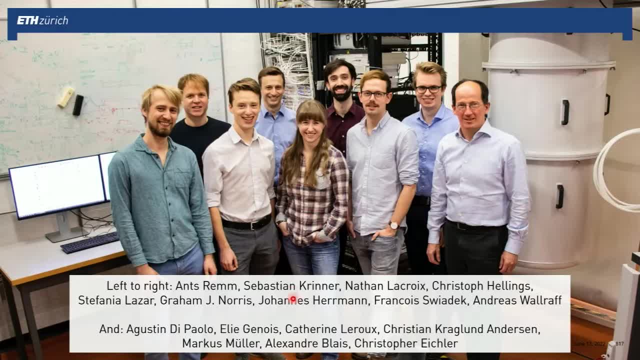 It has everyone but missing Christopher Eichler on this one. There is a list with the theorists again and it mentioned once more that really everyone here contributed throughout many years to that project and with that I would like to thank you for your attention. 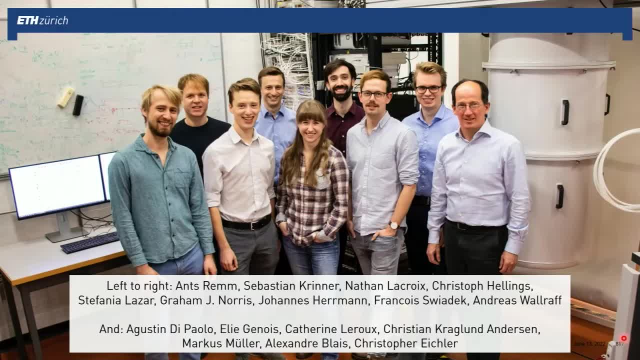 and on the next slide there is a picture that we took sometime last summer with everyone who was currently at our lab and was going to be at our lab next term, also all the undergraduate and master level students. All right, So thank you for your attention. 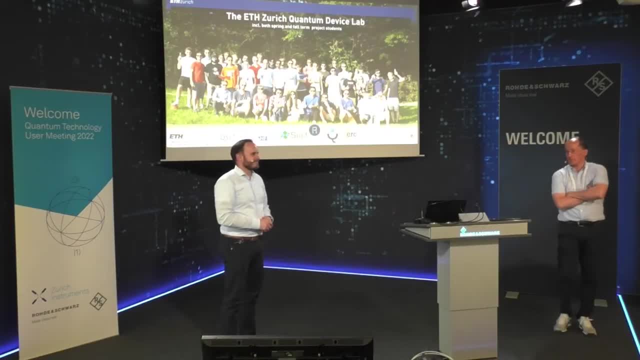 Thanks a lot, Andreas, for this really great talk. I enjoyed it a lot. I am sure there are a few questions still open. Daniel, wait a second, we need the microphone. I have a question about decoding. So for the Distance 3-. 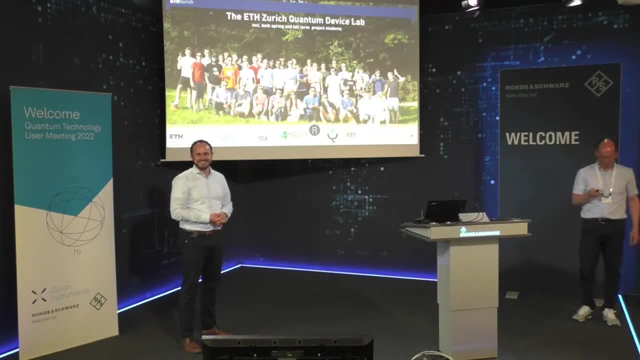 I guess you can do a lookup table. but how about that scale if you actually go to proper surface code with a larger distance? As far as I know, minimum weight perfect measurement does not really run on FPGA. Is there anything on that? Yeah, it is very hard. yeah. 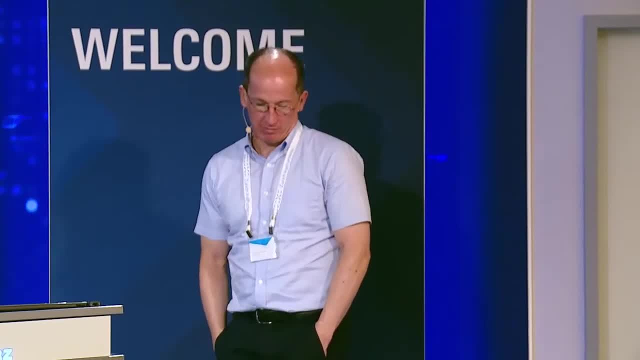 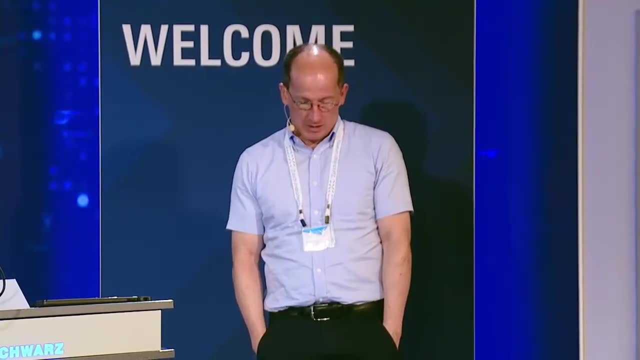 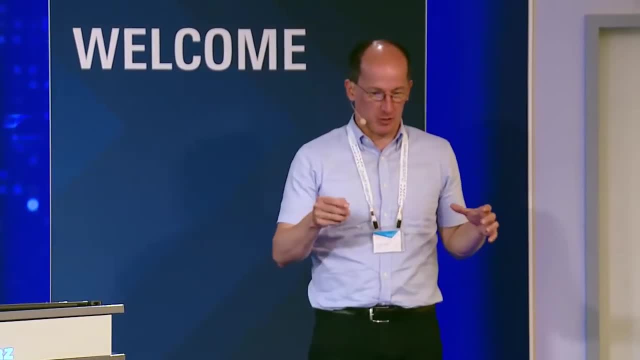 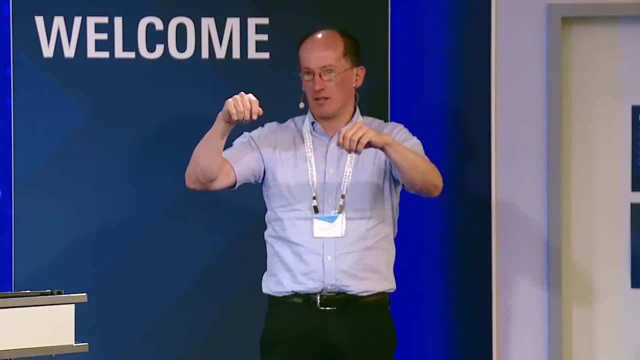 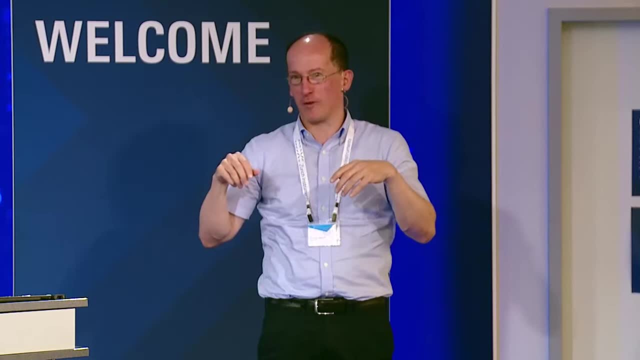 In our case there were eight of them, And you look at which one of the eight ones indicated an error and you do that for every time step, And if you do not have eight but 24,, for example, and if your distance grows, 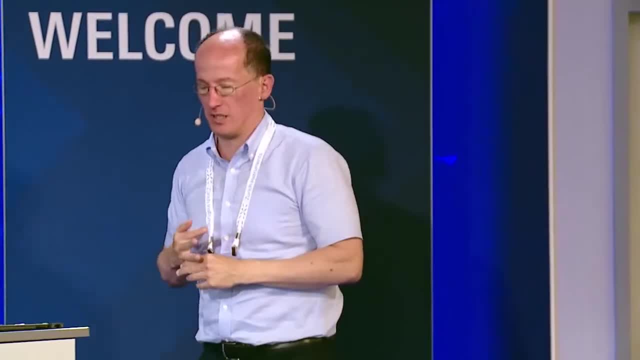 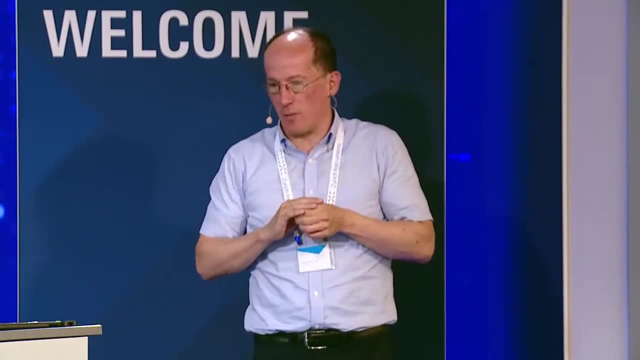 this gets a complicated computational task in itself. this gets a complicated computational task in itself, And the question is: how do you solve that? And the question is, how do you solve that? There are people thinking from the theory side. There are people thinking from the theory side. 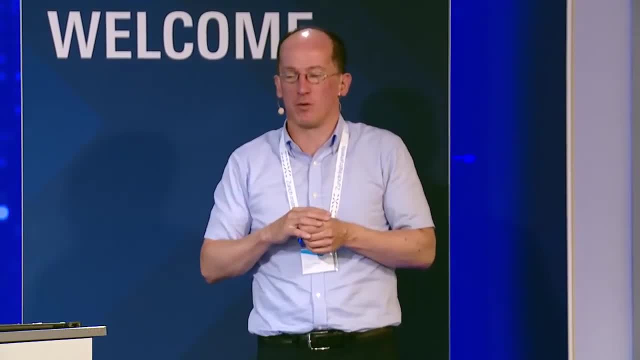 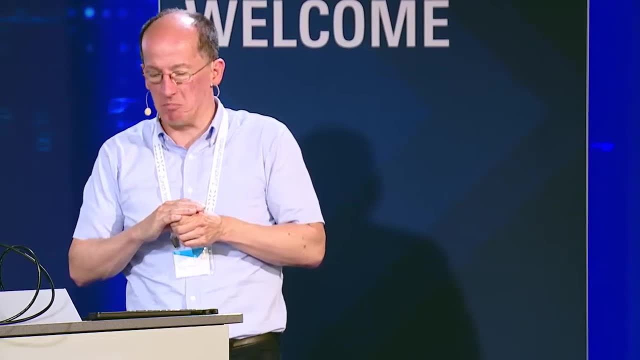 about how to do that and maybe how you could simplify the decoder to be good enough and still not excessively expensive to run. and still not excessively expensive to run. That is a fair question. So my next step: difficult problems on the experimental side. 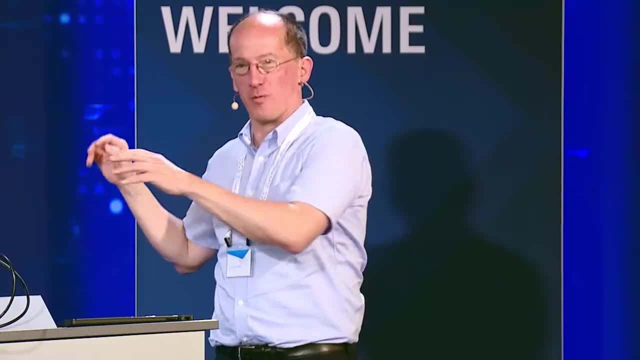 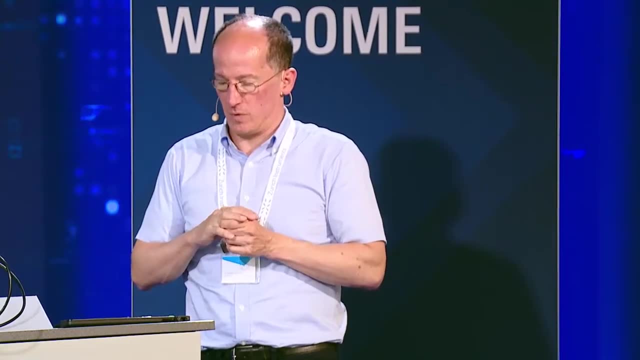 difficult problems on the experimental side are. I find there are harder ones than that one for me, and so I do not think too hard about it. and so I do not think too hard about it. And there is, for example, a group in Cologne that thinks about: 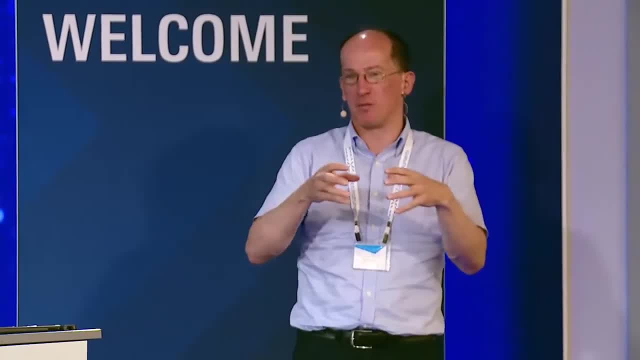 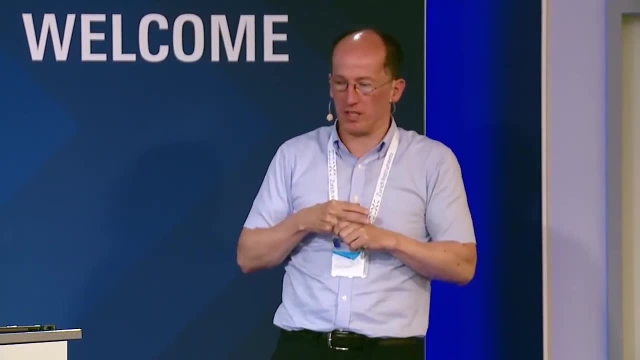 how to simplify the problem enough. how to simplify the problem enough. so maybe just run the decoder on a subset of the whole cell and see how good you can get. And there are also people who think about doing various decoders and see which ones do better than others. And the computationally more demanding ones typically do better, but they cost more. so that is maybe one other way how this could fail, If you cannot make a good enough fast decoder that looks at the errors in your quantum computer. Fair point. Thanks a lot. 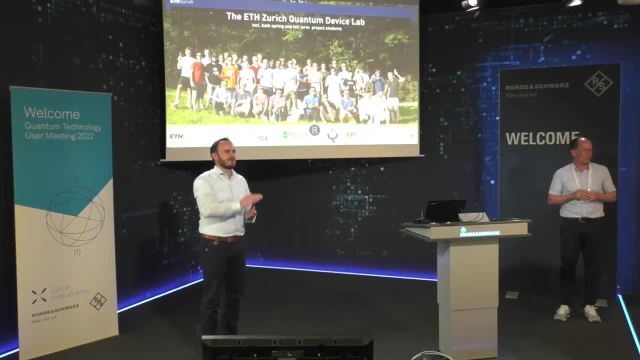 Are there other questions at the moment? Malai, you have a question, Maybe also for everybody participating virtually. if you have a question, please type them in. we will take them over. Malai, please go ahead. Thank you for your talk. 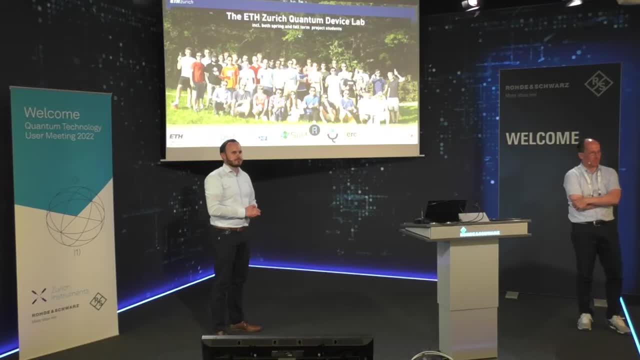 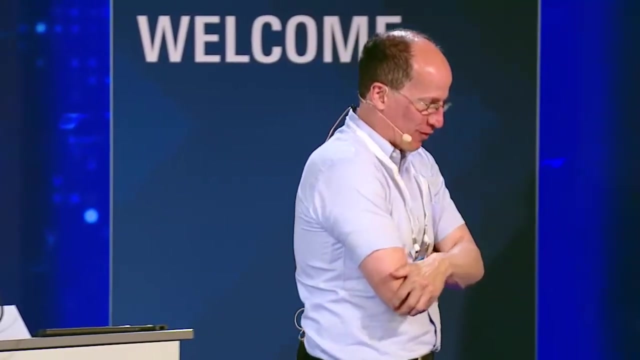 so this is a substantially large experiment with real-time error detection going on. Did you observe any rare events of correlated errors due to cosmic rays and so on? Thank you, That is also a very good question. it also gets asked always now because there were some. in the experiments at Google, there were some indications that there were correlated errors. So one of the reasons how this can work is if there is not too many simultaneous errors on any of the components and if you have something disastrous happening locally, for example. I do not know. some high energy particle hitting your device and creating disturbances locally, then it could lead to errors, to an accumulation of errors at a certain instance in time over some space, and that would destroy your ability to actually correct for that error. I think we have not. 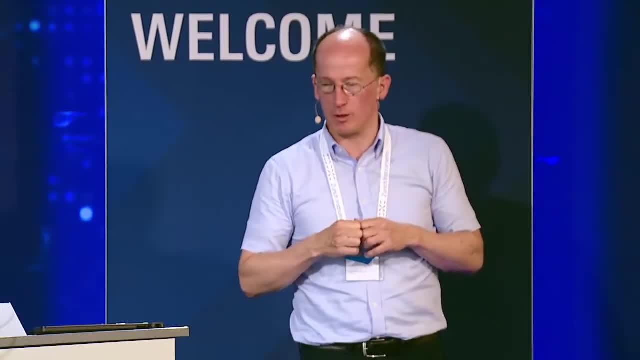 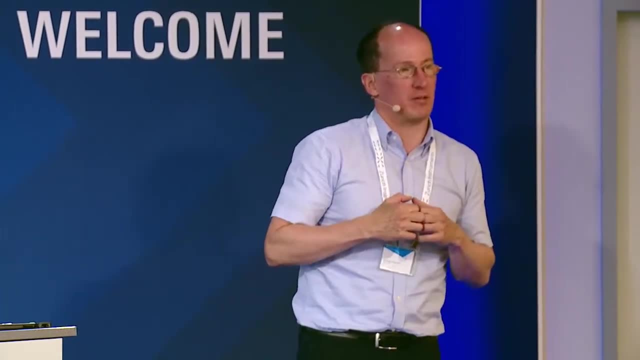 I think we do not have as many chips as Google has and we have probably accumulated. measurement time was less than theirs, but so far we have not seen anything that is obvious on that level. Why could that be? I do not know. I think people started to look at: 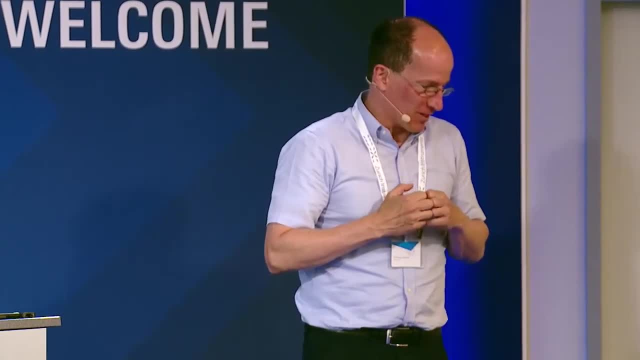 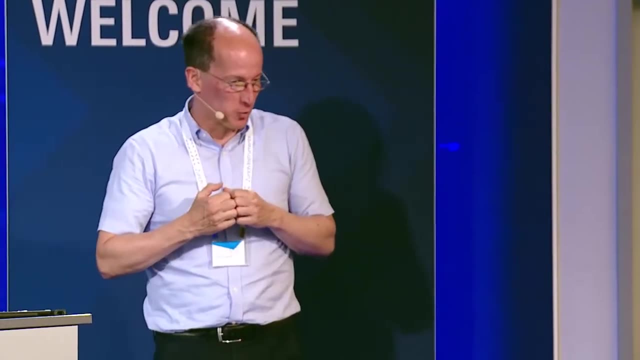 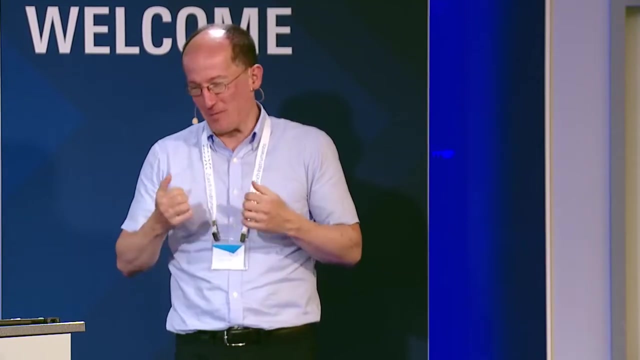 whether there is more, whether there is more natural radioactivity around Santa Barbara, for example, than in Zurich. They used to work in essentially an aluminum container or so while we were in a proper Swiss concrete building, so maybe that matters. I think it is interesting. so there were people. 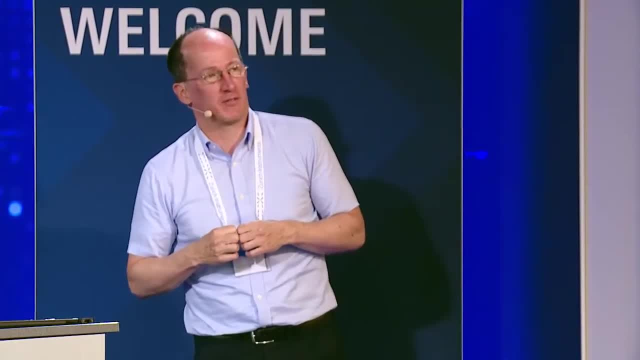 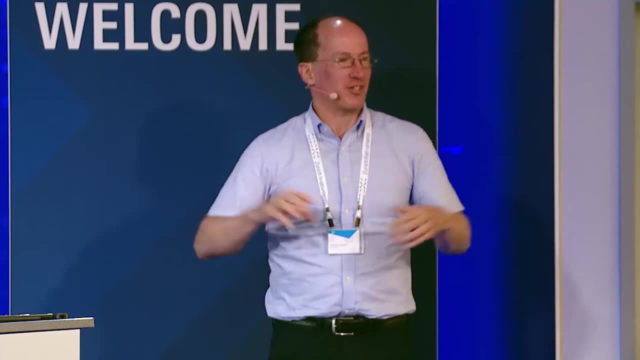 who tried to put radioactive materials next to their devices and see the impact of it, and they saw the impact of it and that type of phenomenon matters and could it matter, like if you now build a large scale quantum computer and you do not want it to be limited by 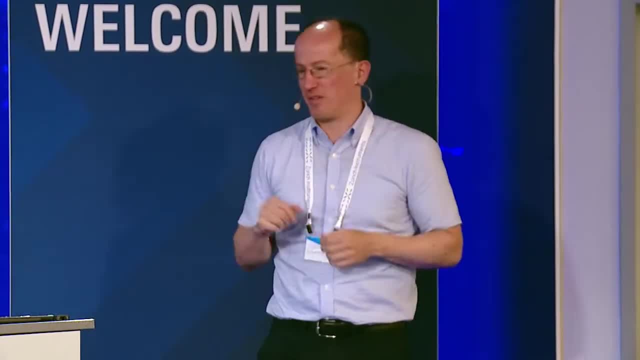 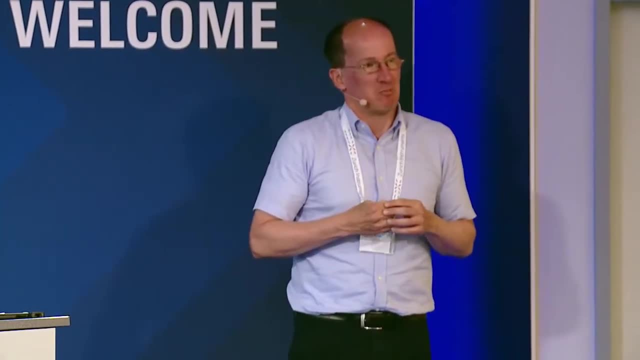 cosmic rays or so that is also a concern, but we have at the moment we have nothing to say about it from the environmental side. I think this type of problem should be there at some level, and how important is it? it is kind of difficult to say. 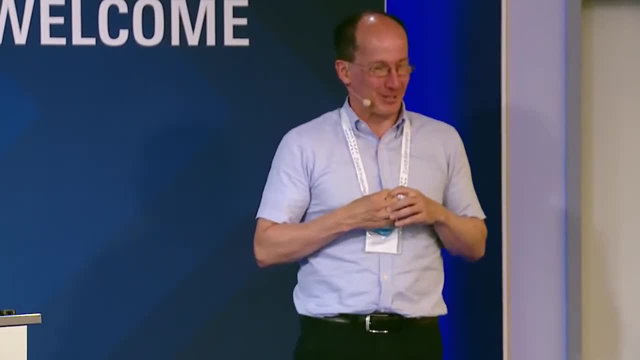 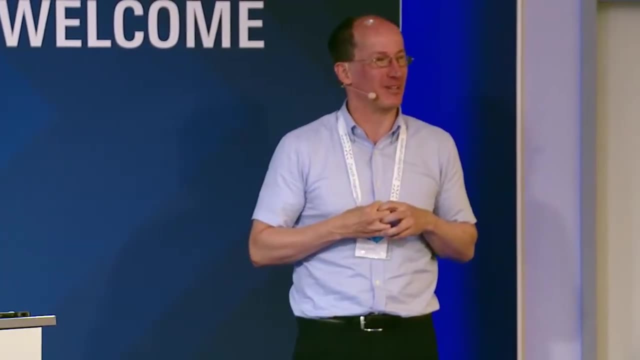 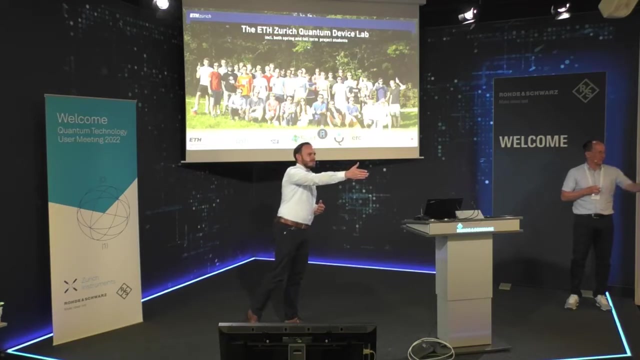 Switzerland also has very big mountains and I know people who do experiments in tunnels that the Swiss army has drilled through all the big Swiss mountains. so I think we would have a good position for our quantum computer as well. Good, thanks a lot. I think there is another question. 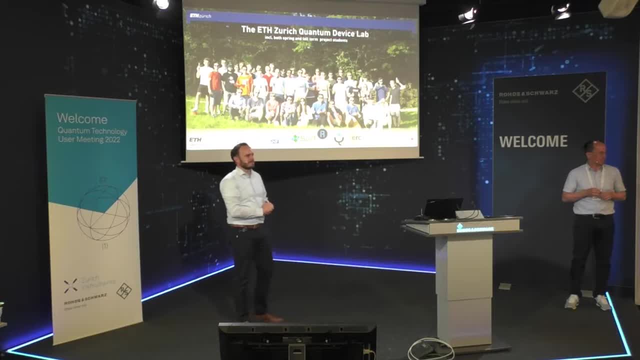 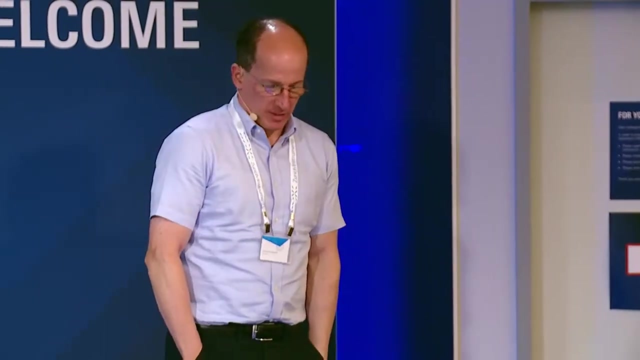 in the very front. Thank you for a very nice talk. My question is: what is the dominant kind of error that you see? Is it phase noise from the control electronics or is it crosstalk between readout lines? The dominant error currently is our two qubit gates. 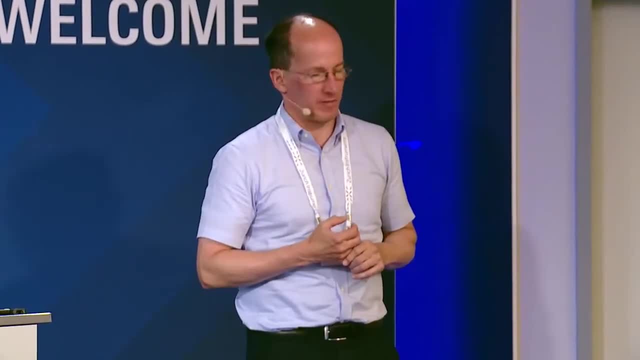 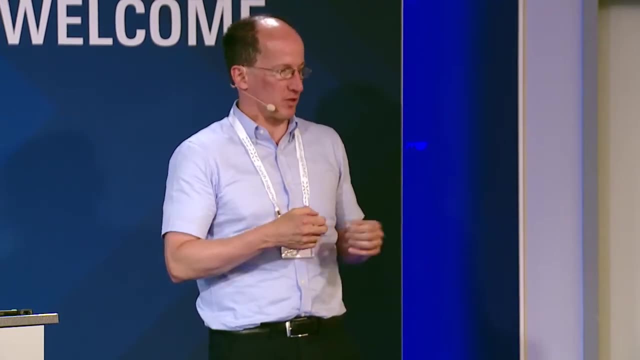 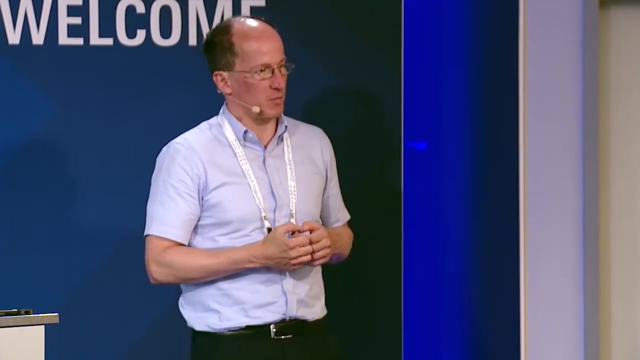 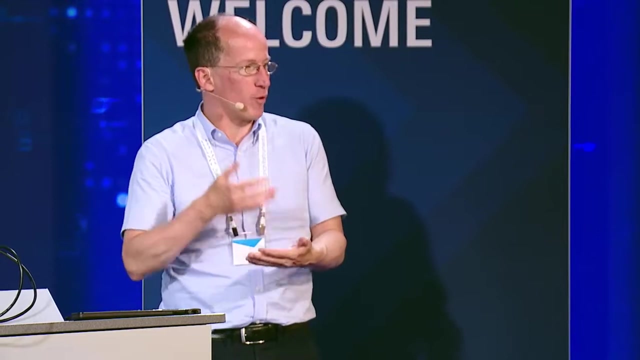 they are the worst single part in our device and the two qubit gate. error currently is dominated by surface defects and so these surface defects- it is an ensemble of likely microscopic in origin defects. and those microscopic defects because there is many of them and they are all over in energy. 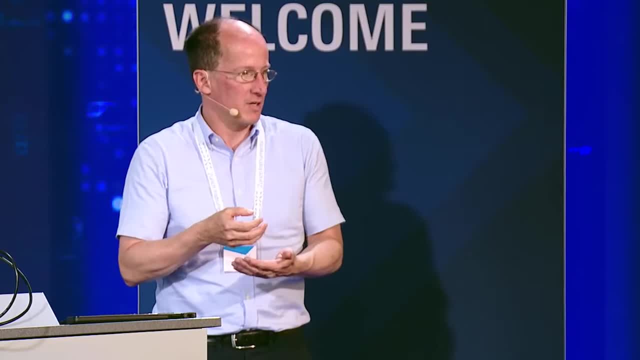 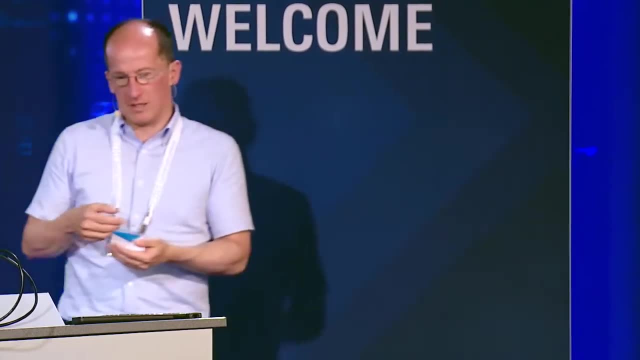 or so some of them tend to couple strongly to the qubits, and those who are then most strongly coupled to the qubits, they really adversely affect the two qubit gate fidelities, and so my feeling is, if we did not have those, we would probably 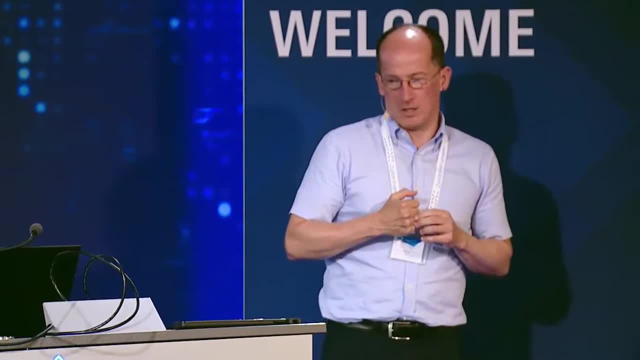 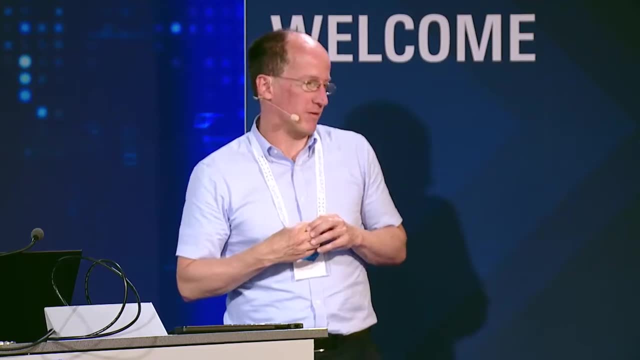 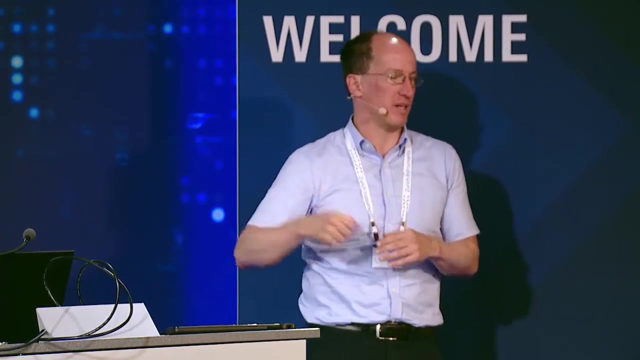 have done the experiment maybe half a year earlier or so and the overall performance would be better. so I think currently it is we are working on improving our fabrication techniques to mitigate that some and hope that we can gain kind of the two qubit gate fidelity to get across this threshold. 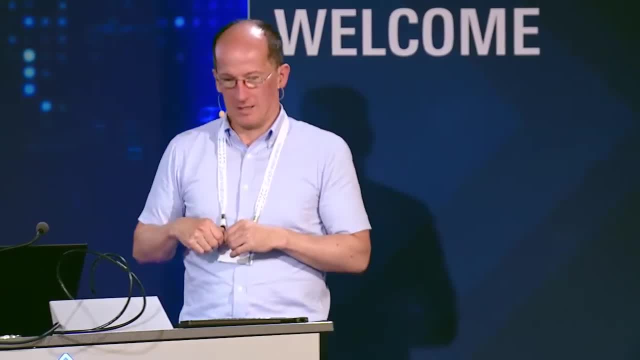 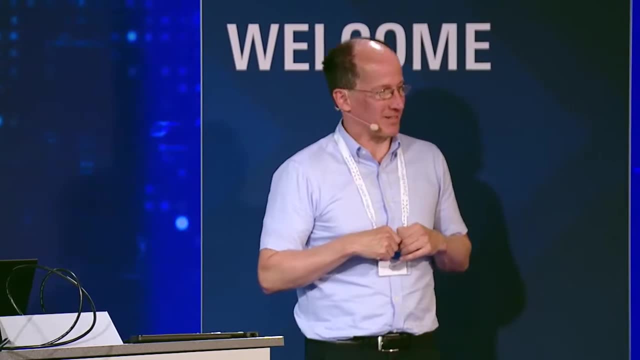 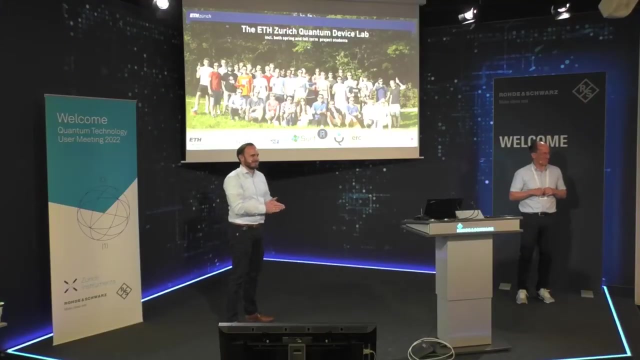 for example. so it is at the moment. I would say, at the level that we are at. it is something that we need to fix and otherwise we will tell the manufacturers of our electronics to improve it. good, with that, let's hope that the manufacturer of your electronics 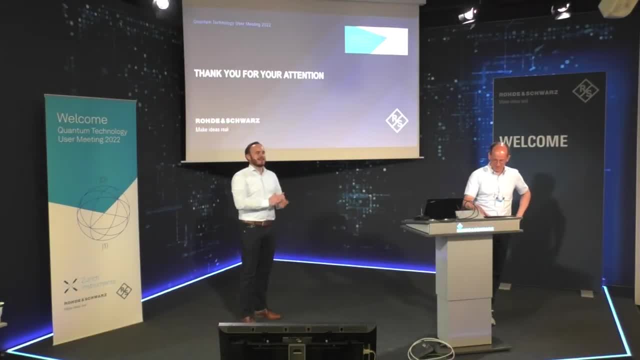 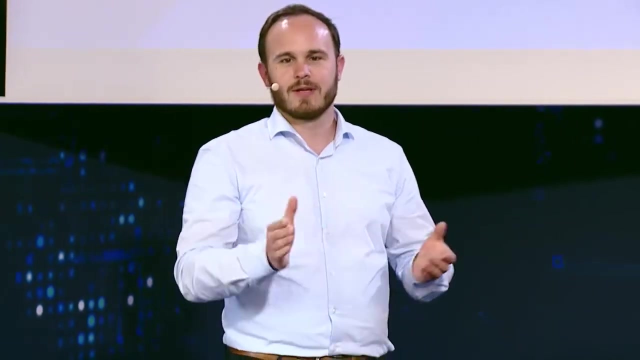 hears that. are there other additional questions? I don't see any at the moment, so with that I would close the session and all talks for today. let's thank Andreas and all speakers again. thank you. so with this we close the virtual event for today. we will come back tomorrow.